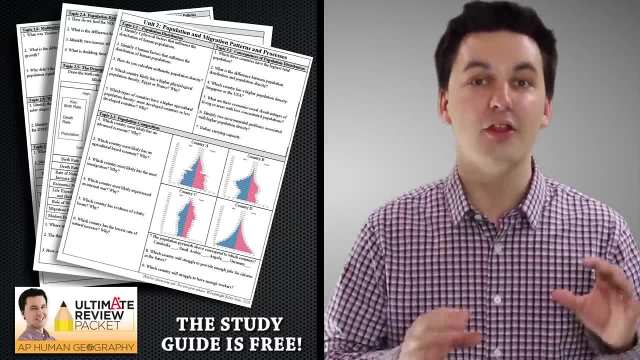 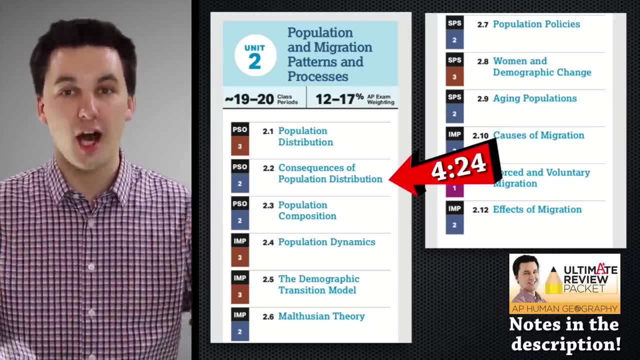 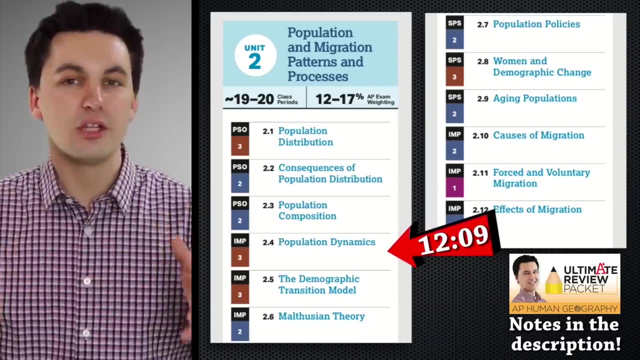 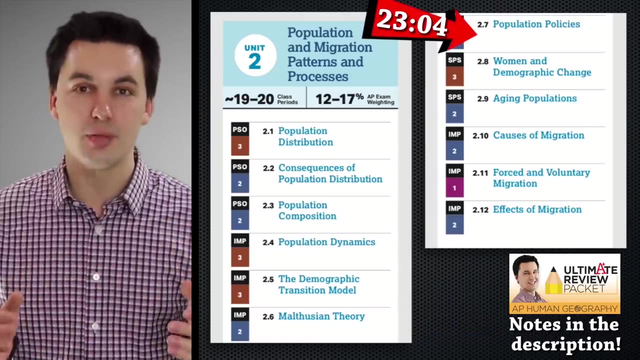 Go get the study guide- It's part of the ultimate review packet- and then follow along throughout the video. First we're going to be talking about population distributions, Then we're going to move on to talk about actual consequences of population distribution From there. then we'll go on to look at population composition, Then we'll look at population dynamics and then the demographic transition model. We'll then go to Malthusian theory and also population policies. Next we'll elaborate on those population policies and look at women and demographic changes. 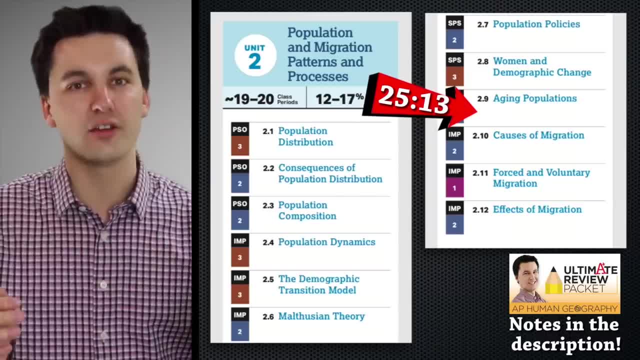 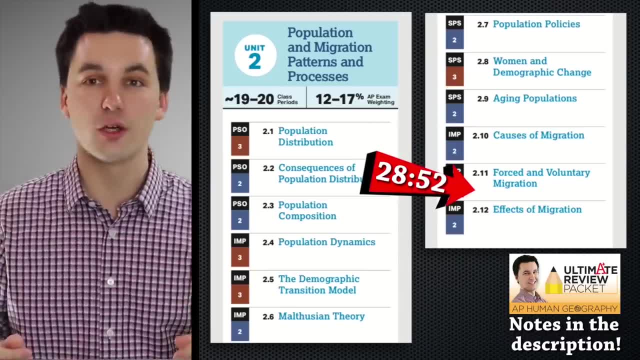 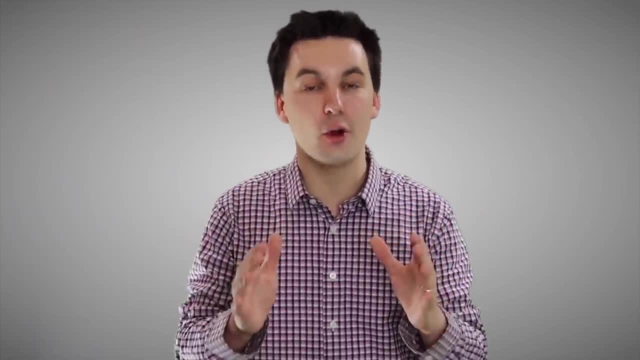 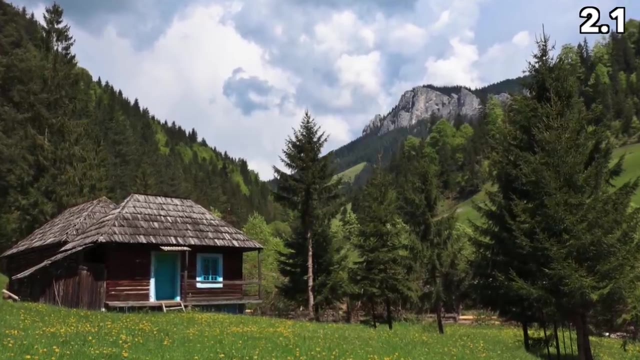 And also we're going to talk about population distribution And also aging populations and the impact that has on society. After reviewing all the different population concepts, we'll shift gears into actually migration, Moving then to forced and voluntary migration and ending with the effects of migration. As you can see, there is a ton of stuff in this video and it's going to go pretty fast. When geographers study population distribution, the first thing we have to ask is: why would someone live in this location versus that location? A lot of times it comes down to the climate, It comes down to life. 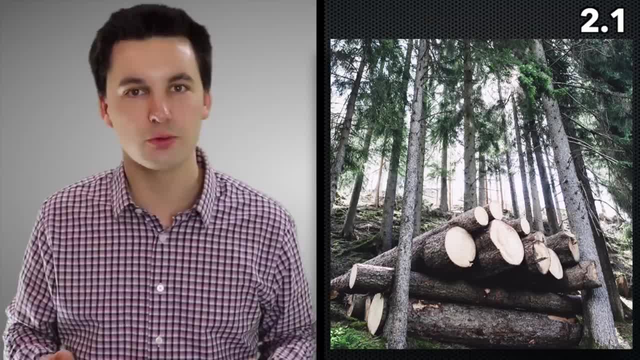 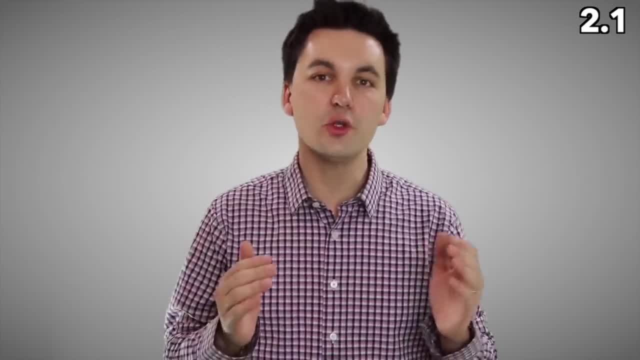 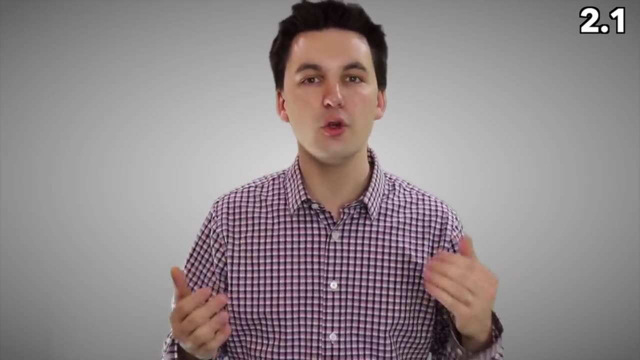 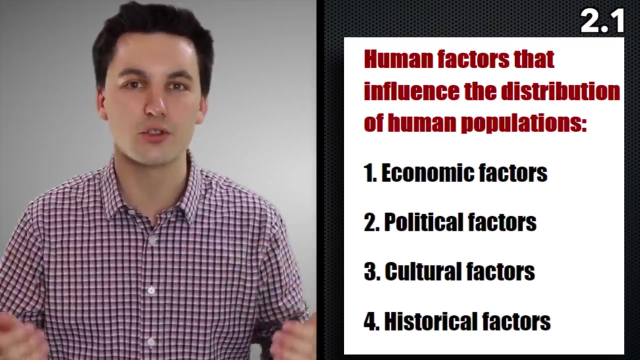 It comes down to land forms, It comes down to bodies of water or access to natural resources. All these things shape the development of society in an area. So those are just the physical factors, But there's also human factors of why someone would live in place. one over place. two: For there, think about your own life. What do you value in life? What do you want when you're looking in the future? One: hopefully most of you are saying: I want to be successful, But you want to have a job. There has to be opportunity. Economics, our first human factor. Economics is actually the number one reason why people are successful. 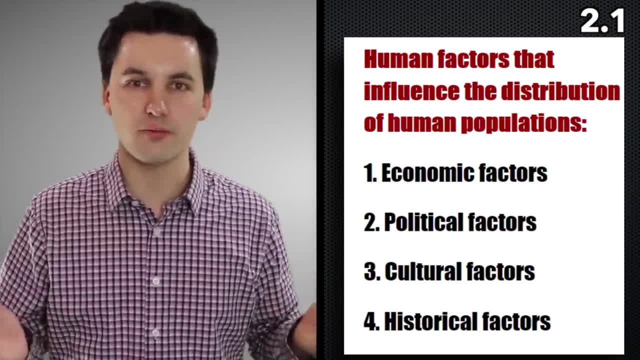 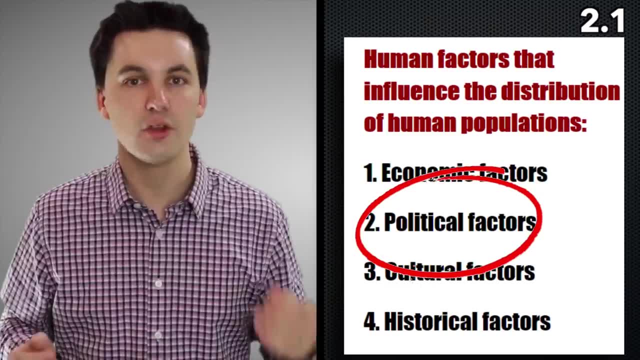 people migraine. Next thing is: we want to live in an area, probably where we feel safe. You don't want to live with uncertainty, So political factors come into play. We want to make sure that, whatever we're living, the government is functioning correctly. There's 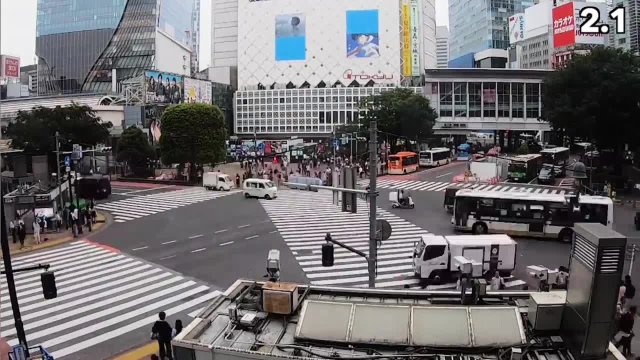 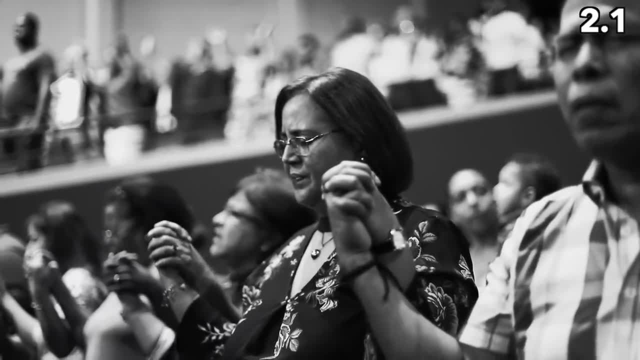 stability in society. It's not anarchy. We aren't constantly unsure of what's going to happen. Then we also want to make sure we're part of a community that accepts us. Cultural factors are really important, And then, lastly, historical reasons come into play. Some people 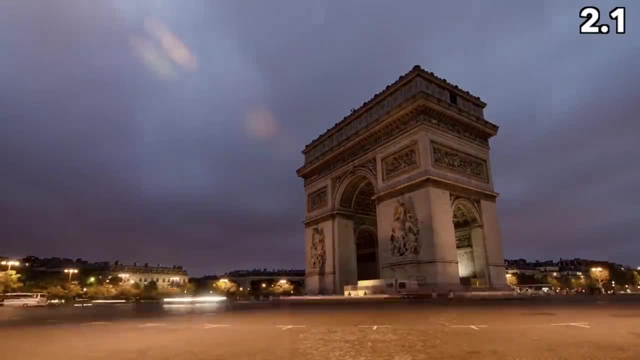 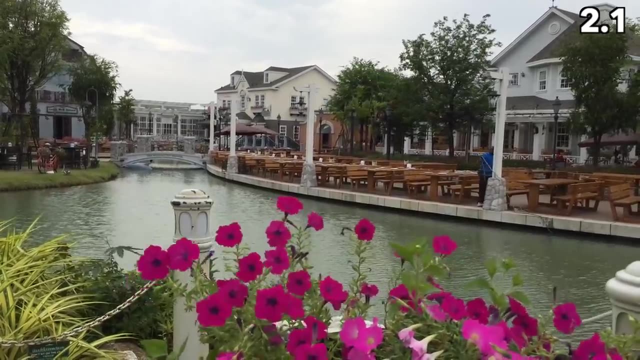 choose to live in a city because of the architecture or the historical significance of it, And others live there because, well, they're born there and the city was just created based on historical events in the past. Now we're going to talk about population density. It's 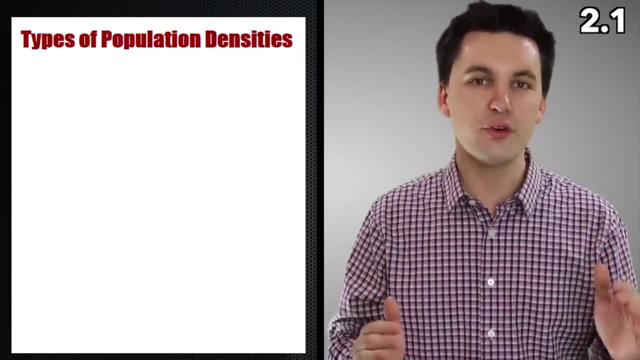 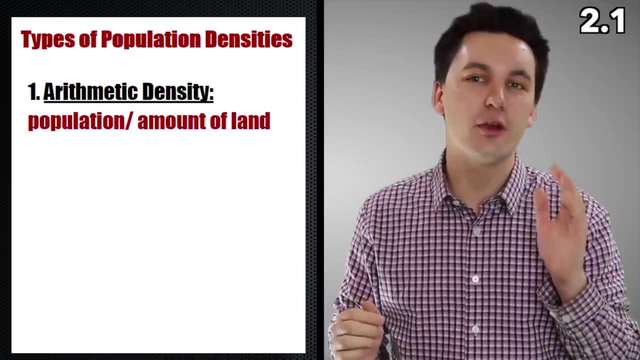 just the amount of people that are living in a particular area, And there's three different main densities that we cover in human geography. They all show different aspects of society. Our first type of density is the arithmetic density, and it's our easiest one to calculate. 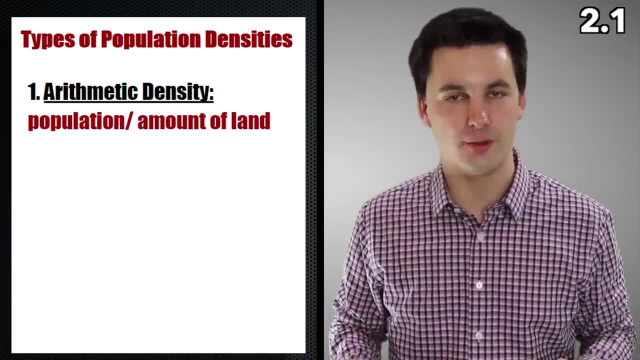 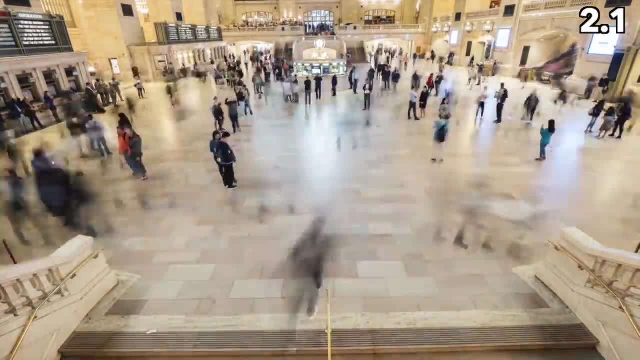 We just need to take the total amount of people and we divide it by the total number of people in the total amount of land. Really, it just shows how spread out people are. Are they clustered, Are they dispersed? This density is great for just getting a quick snapshot. 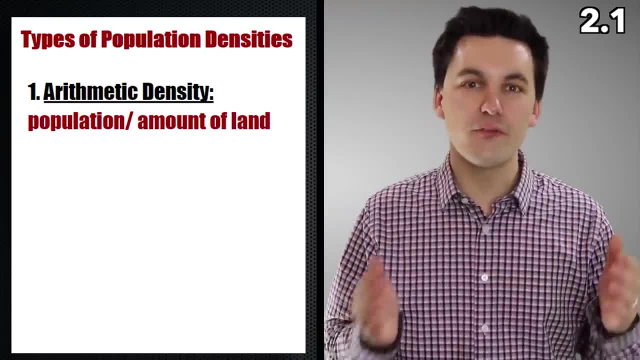 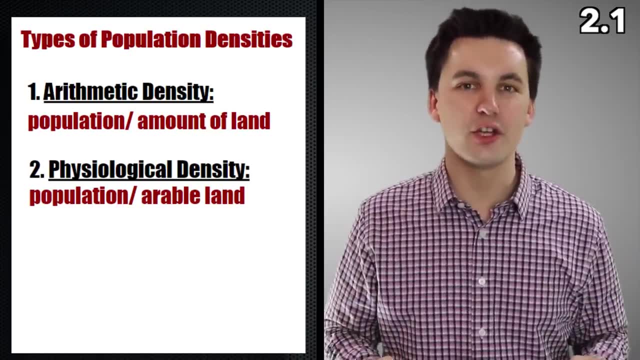 of a society. Now the next density is really important. This one is our physiological density, and it's showing us our total population divided by the amount of arable land. What this density shows us is how much food do we need to produce per unit of land. Higher this number is mean. 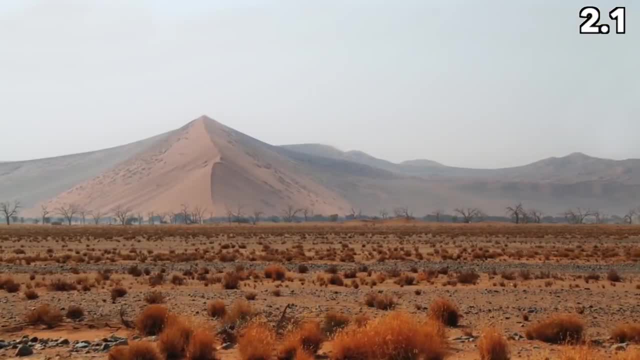 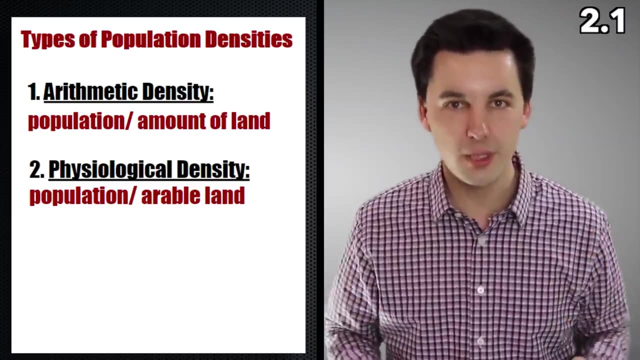 we're going to put more stress on our land, We might run into issues like desertification or where we start to see our soil become infertile And no longer able to produce food. That would be a big issue, especially if you want to. 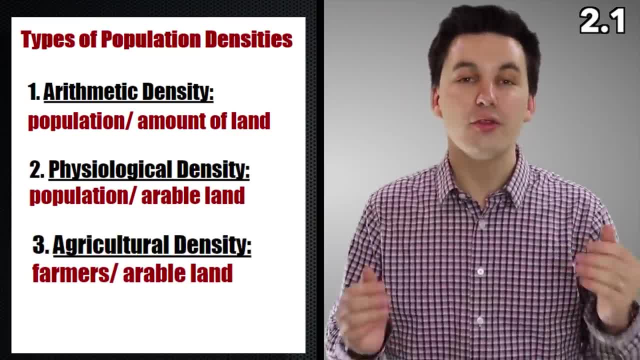 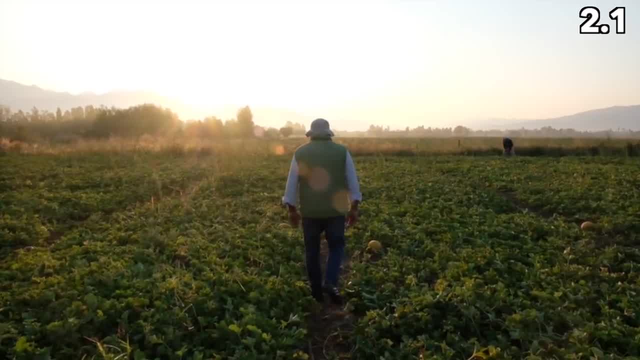 get out and get some Chipotle. Lastly, we have our agricultural density, and this is our farmers, divided by arable land. What this shows us is how advanced is our technology If we have a really low number. that means we don't have a lot of people working in the 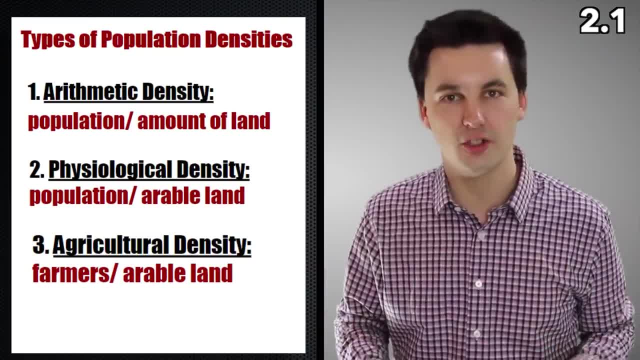 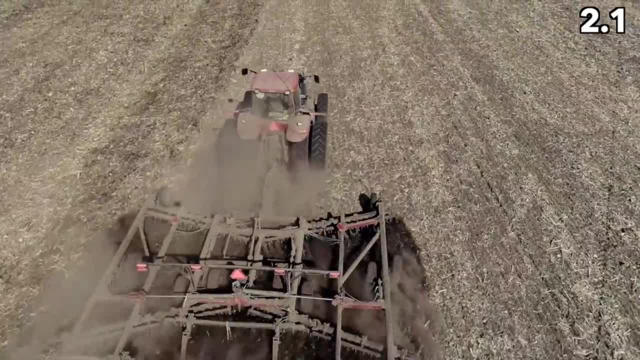 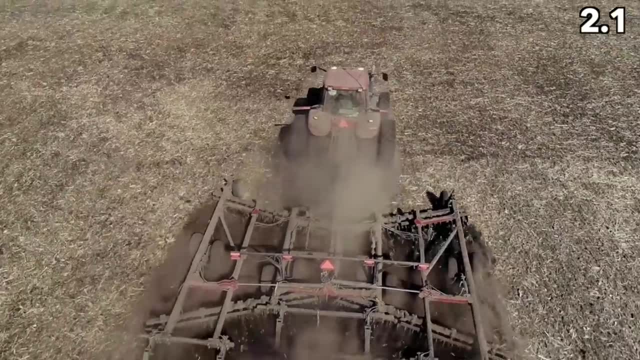 field of agriculture, They're allowed to do other things. We can see more specialization, and that's normally because then the society is using more advanced techniques when it comes to farming, Whether it be tractors or combines, whether we're having more pesticides and fertilizers. we no longer have to have as many people actually 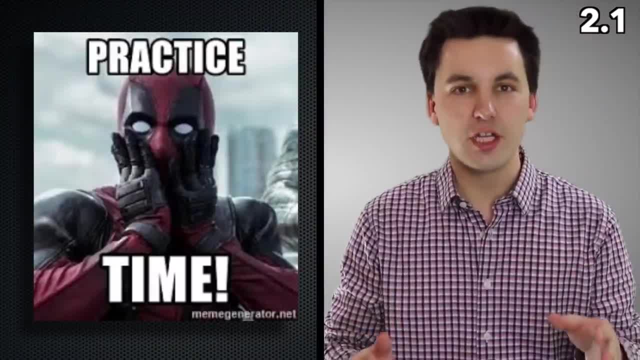 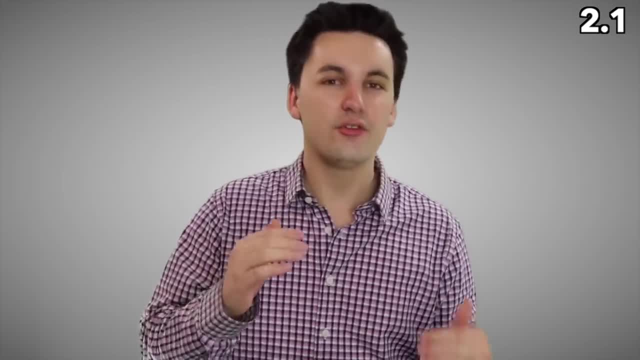 working in the field of agriculture. Those are important to understand. Pause this video and answer questions four and five in your study guide. Once you're done, unpause the video. All right, how'd you do? Did it make sense, Did it not? If you need a little bit, 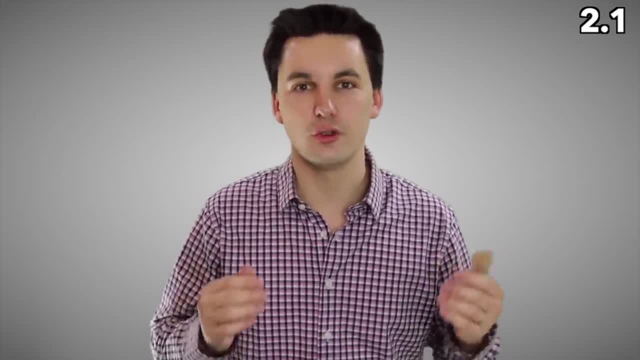 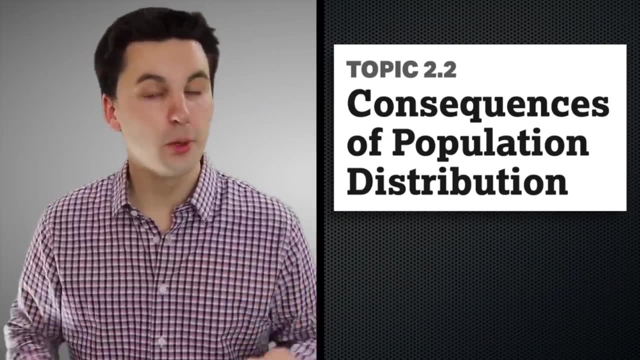 more time to practice some of these concepts. check out some of my videos on the YouTube channel. I actually have a great one on Minecraft where it analyzes all the different population densities inside Minecraft. All right, we're on to 2.2, where we're looking at these consequences. 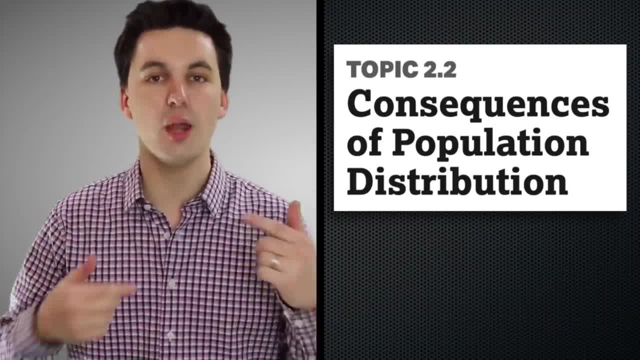 What we're going to do right now. pause this video, try to go through and answer the different questions. Unpause the video once you're done. This way, you can see if you know these concepts already or if you're going to need a little bit of review. 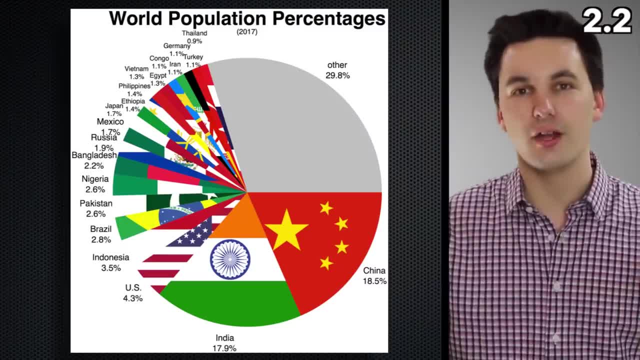 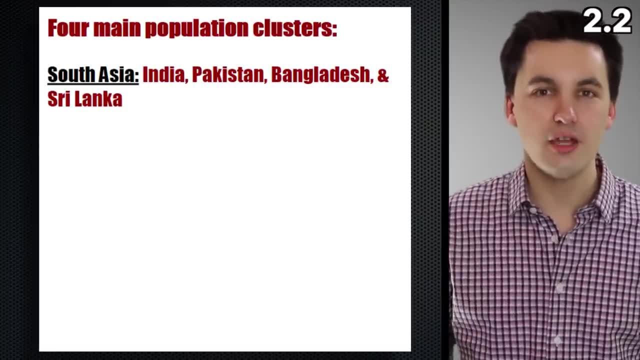 Populations are changing all over the world. Today we have China, India and the United States with the highest population totals, But the world has four main population clusters. Here we have South Asia, Southeast Asia, East Asia and Europe, where populations are growing. 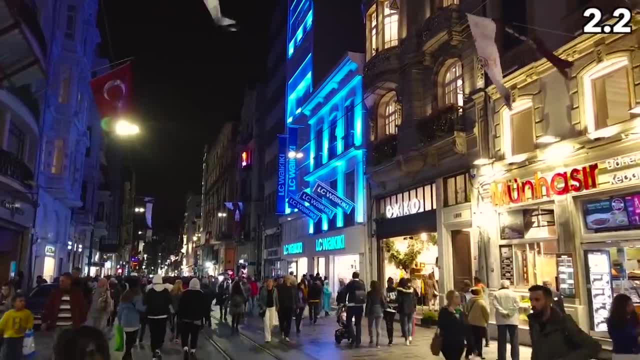 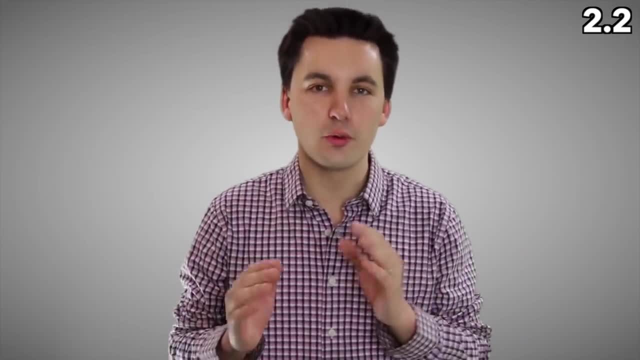 at a very fast rate. Actually, Europe recently is starting to slow down a lot. Now, throughout all these review videos, I'm going to try to highlight different concepts that students sometimes get confused with, The first one that we really need to understand the difference. 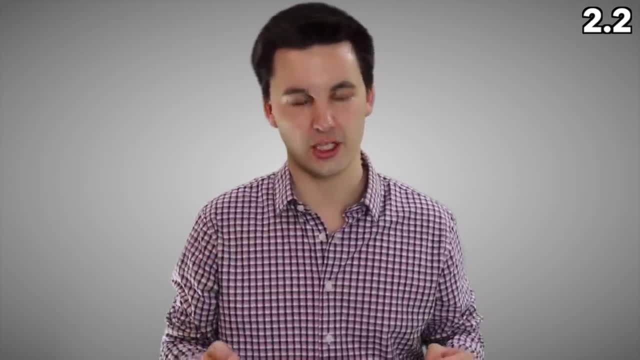 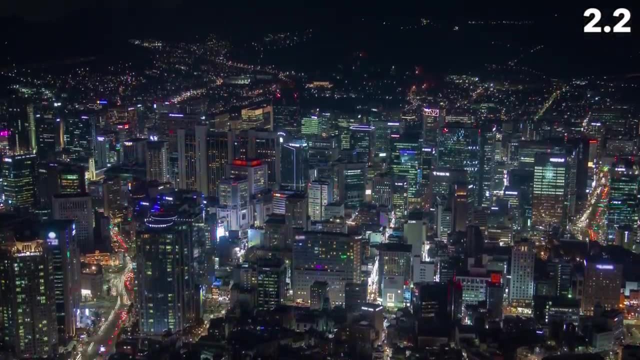 between is population distribution and population density. Population density: when we're talking about this, just think about how many people are in one spot, So how many people are located here. When we're talking about distribution, it's how many people and where they're living. It's the spread up. So where are things located? 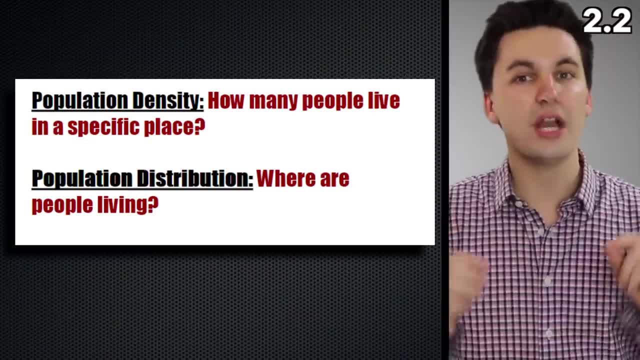 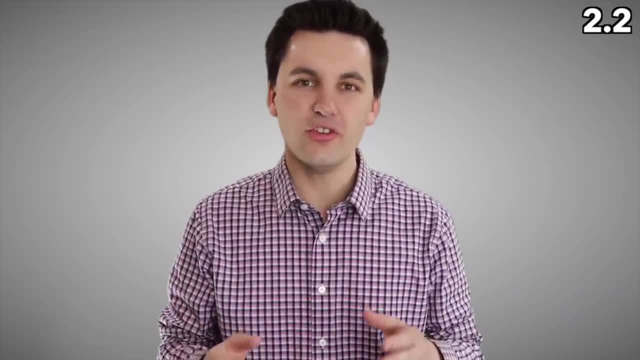 Are they clustered together all together? Are they dispersed? We're not looking at the actual numbers, We're looking at more of just the location. Another area where students sometimes lose points is on questions that apply concepts to different states. What country do you think? 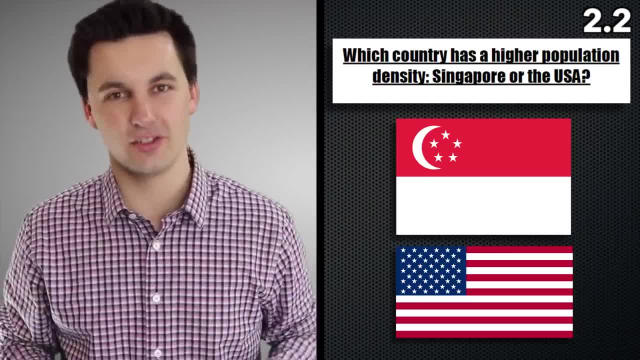 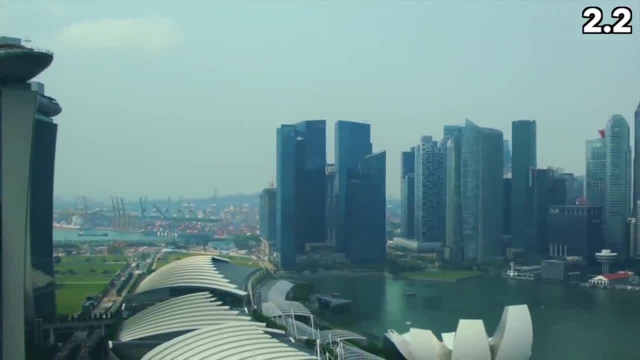 has a higher population density: Singapore or the United States? Even if you don't know much about these two states, you can break this down If you can remember where Singapore is kind of located within the world- and I know that their size isn't as big and the 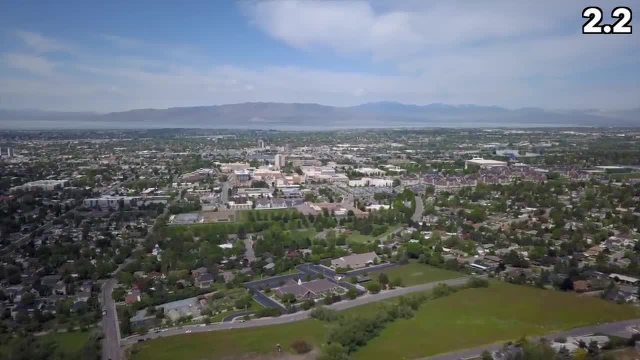 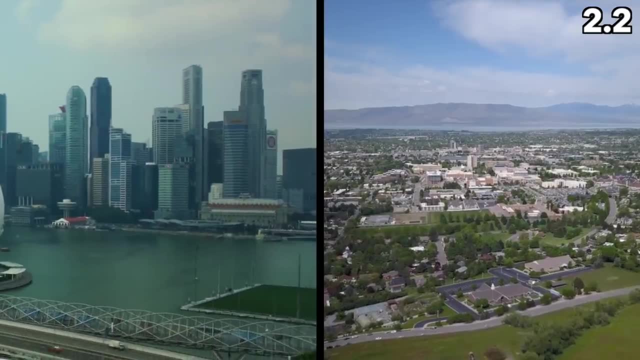 US is geographically very large. they're spread out over a large area. answer: Singapore. Singapore actually has over 8,000 people per city. The United States is only around 90, 94 people per kilometer. Now, you don't have to remember. 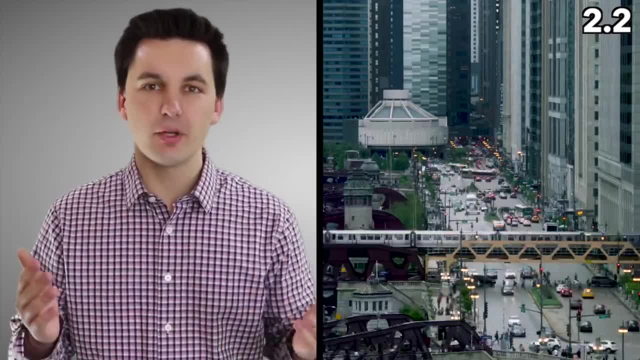 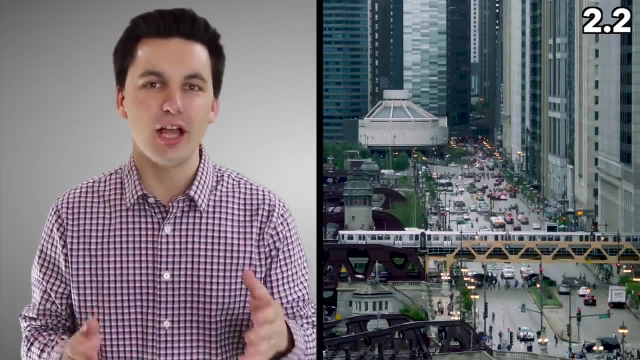 those numbers, but just be able to understand these concepts. Just by having a general understanding of density, geographers can infer a bunch of different things that might be occurring inside a state. States that have less concentration in their populations are more likely to see. 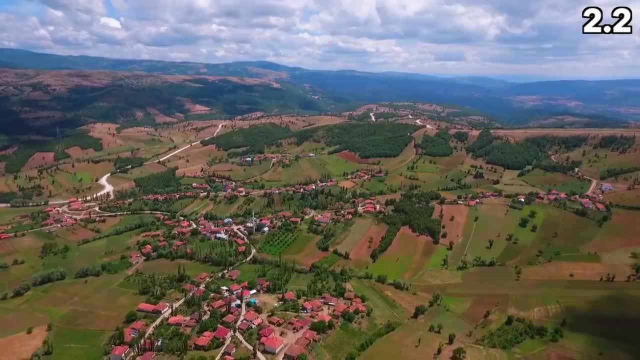 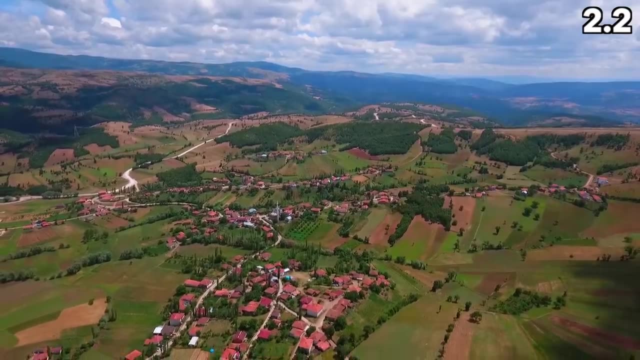 populations dispersed throughout the state. They're going to be spread out. This is going to create things like, maybe, primate cities, which we'll talk about later in our unit six video. It's also going to lead to a lack of services and goods for people. We'll see less schools. 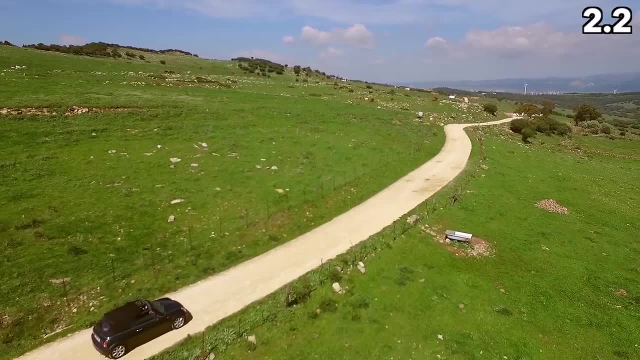 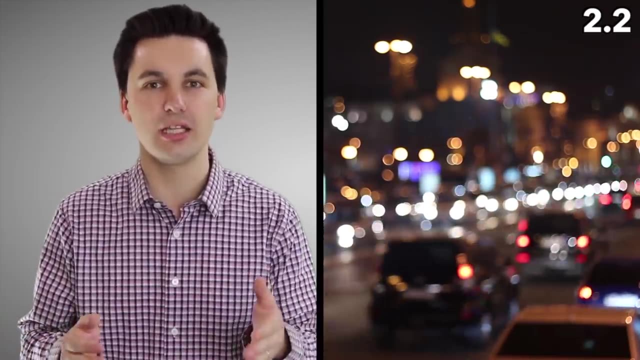 less health care, less hospitals, We're going to have other issues that are going to occur, And so we have a lot of communities who will become isolated. On the other hand, we could look at one of the disadvantages to actually just being in a very densely populated area. 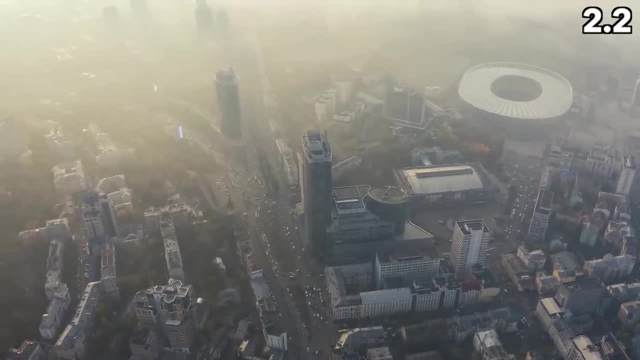 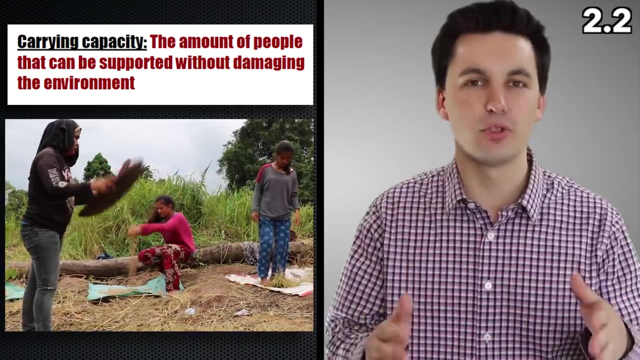 When we're talking about the environment with pollution, when we're talking about overpopulation, a lack of actually being able to find jobs because there's so many people who are trying to get them To wrap up 2.2,, we're going to talk about poverty. 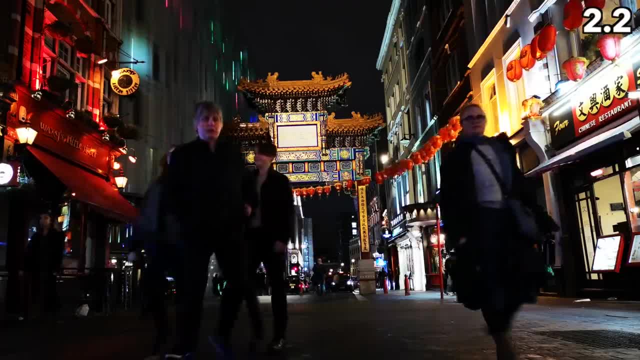 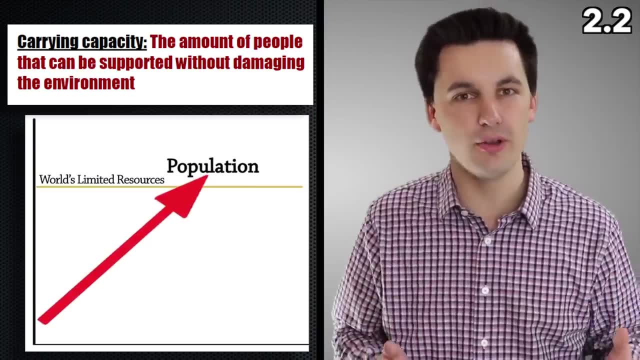 We're going to talk about carrying capacity. Carrying capacity is just how many people are living in one geographic area without damaging the environment. If we exceed this limit of how many people could live in an area and the environment starts to be damaged, we have exceeded our carrying capacity. 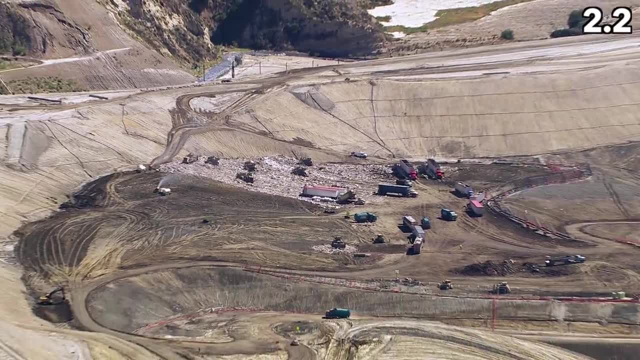 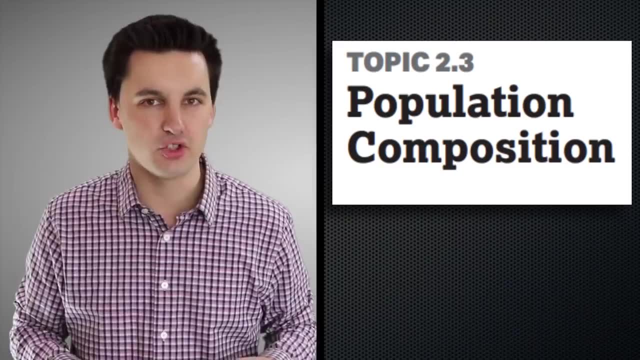 People are going to start dying, The environment's going to get destroyed, We're going to lose arable land. We might start to see other catastrophes occur within society. 2.3 is all about population composition. Here we're looking at age structures. 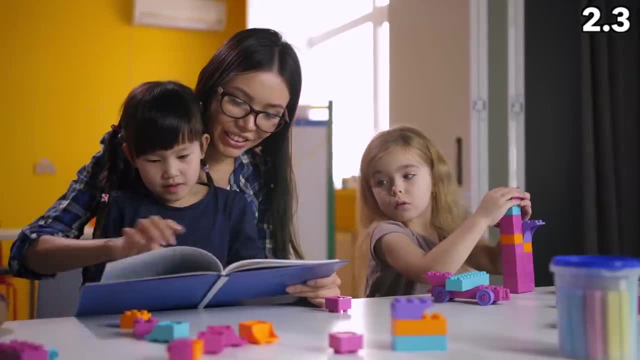 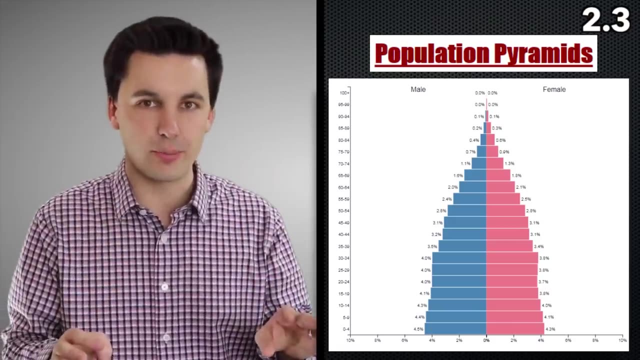 We're looking at demographic data. We're going to be looking at gender. We're also talking about population pyramids. There's a high probability the AP test will have one of these on there, So we're going to quick review the population pyramids. 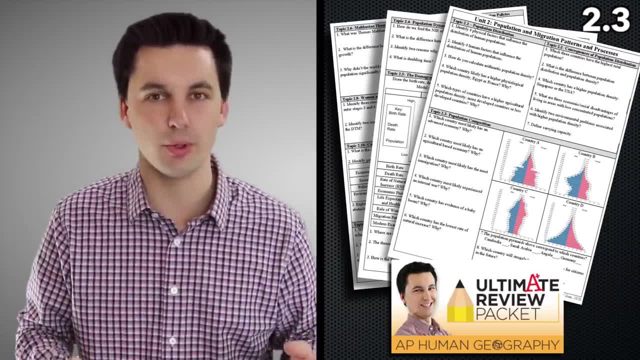 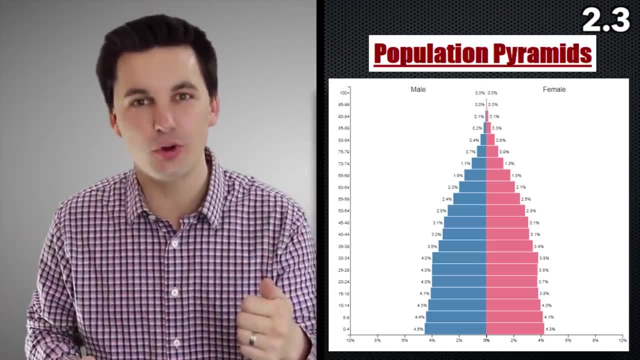 Then I want you to pause this video, practice these application problems, and then we'll go over the answer. Okay, here we go, Really quick. One of the first things we should know is when, looking at this is we can see it's broken. 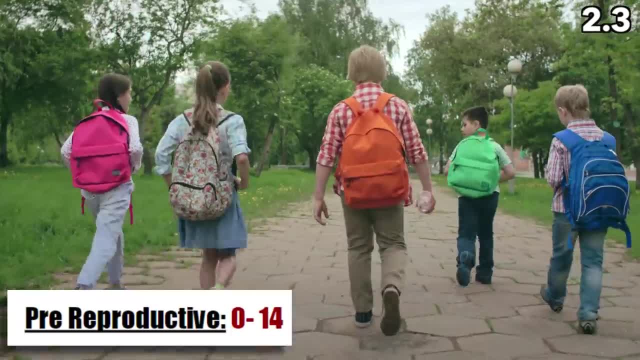 down by age ranges. We have our pre-reproductive years, which is zero to 14.. We have our reproductive years, which is 15 to 14.5.. We have our reproductive years, which is 15 to 14.5.. 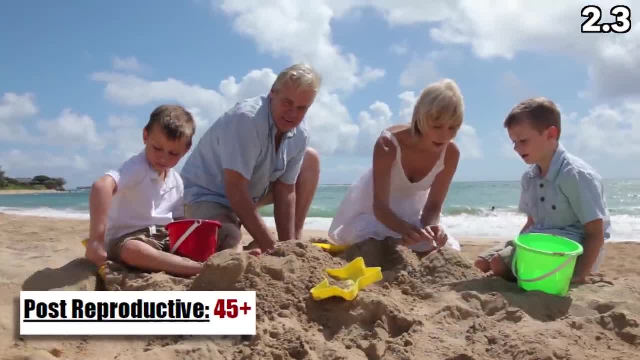 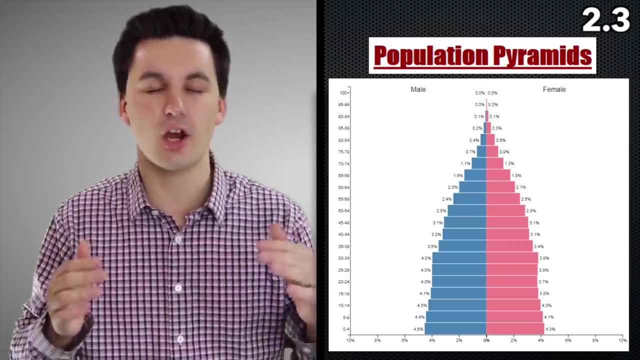 We have our reproductive years, which is 15 to 14.5.. And then we have our post-reproductive years, which is 45 and up. That's important because it shows us well growth rates. Are we growing as a society? 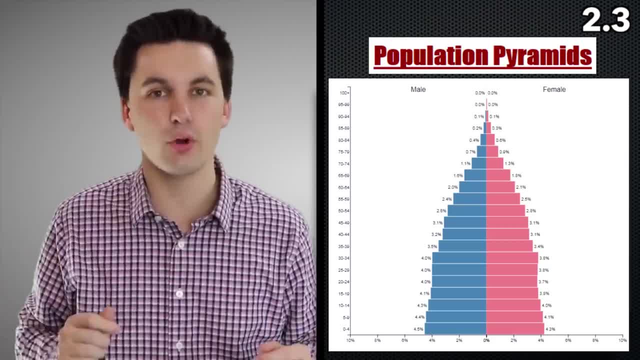 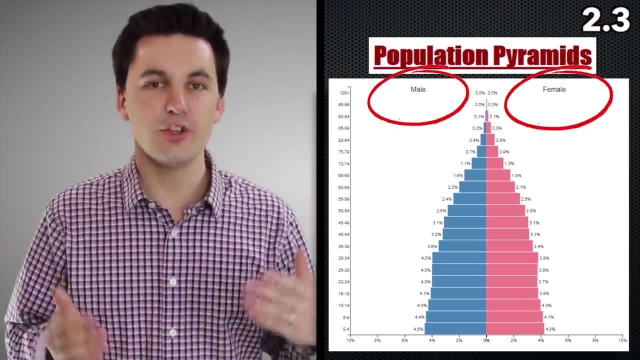 Are we not? Are we more likely to have kids five years down the road, Or are we going to start to see a shrinking of the children population? The very next thing you need to notice is it's broken down by gender. This can show us a lot about the culture or just how society is currently operating. 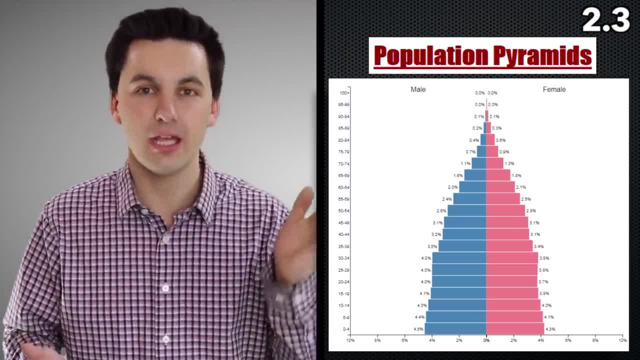 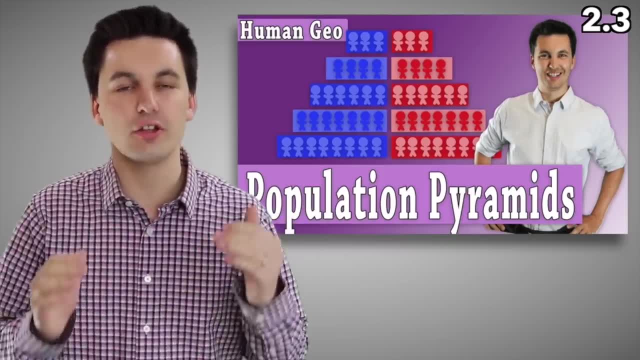 It can also reveal some historical events that maybe occurred in one of these societies. That was a really quick review and if you're still struggling with this concept, go check out one of my YouTube videos that'll cover this concept more in depth. Take out that packet if it's not out yet. answer the following application questions. 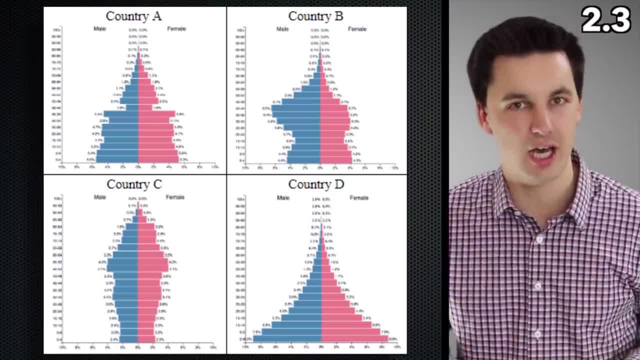 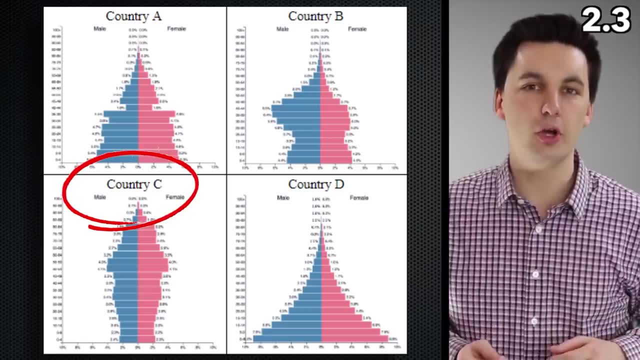 Question one: we're trying to figure out which of these countries has the most advanced economy. This one's going to be country C. As the economy advances, we start to see less people having kids. more people urbanize. They live in large cities where you don't need to have a large family in order to take 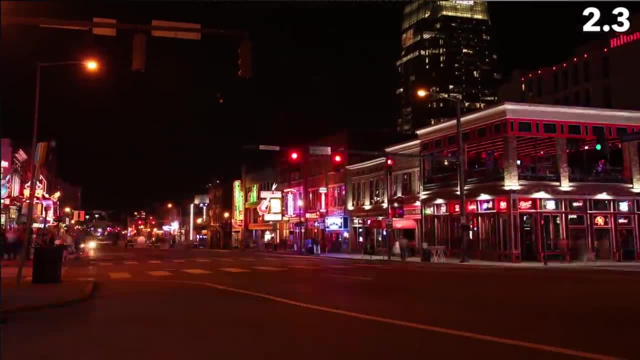 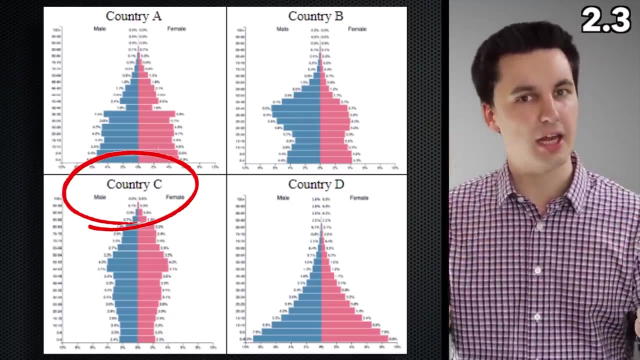 care of the home or to be able to work on the farm. So advanced societies see their population growth drastically decrease Right away in your head. when you see that go okay, we have a small base not having a lot of kids. we're starting to see our populations living longer and it's starting to be more. 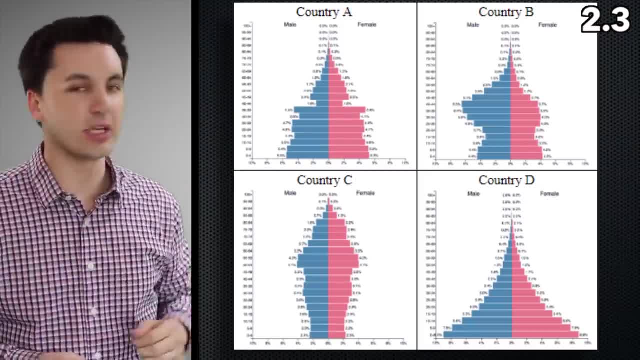 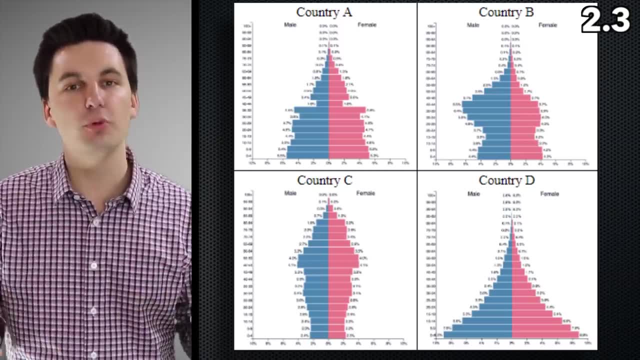 evenly distributed. It's advanced. Question two, on the other hand, we can see, is asking the opposite: Which one of these countries is most likely to have an agricultural-based economy? This would be an economy that's less advanced. Country D, we can see, has this massive base. 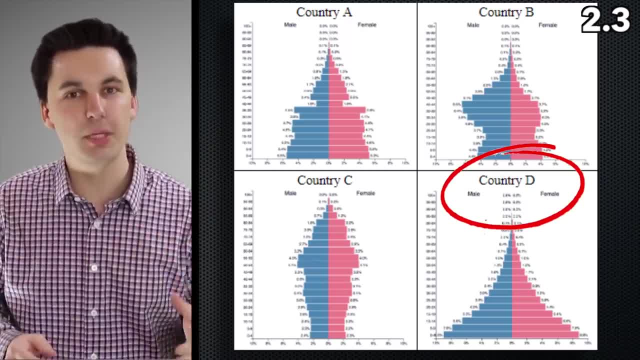 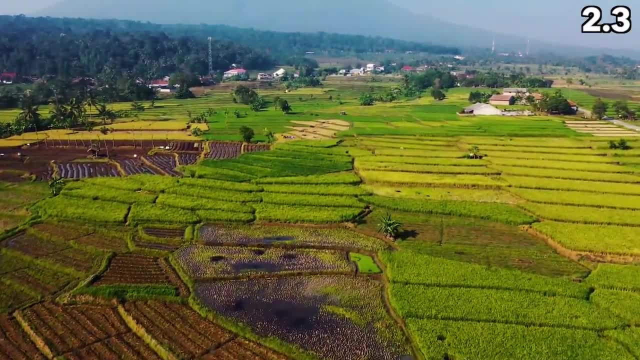 That huge base is showing a real growth, Really high birth rate. Lots of people are having kids. That's normally a sign that a country's in more stage two of the demographic transition model And they're having a lot of kids because they don't think they're all going to live or they 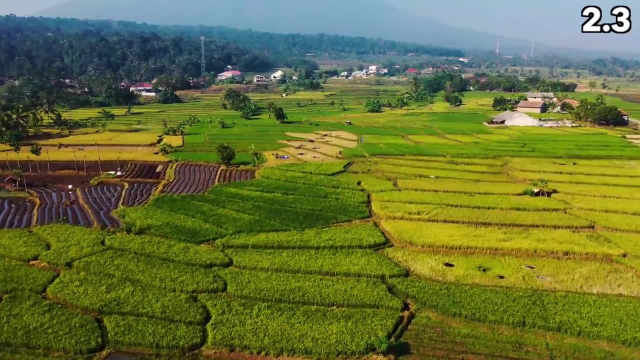 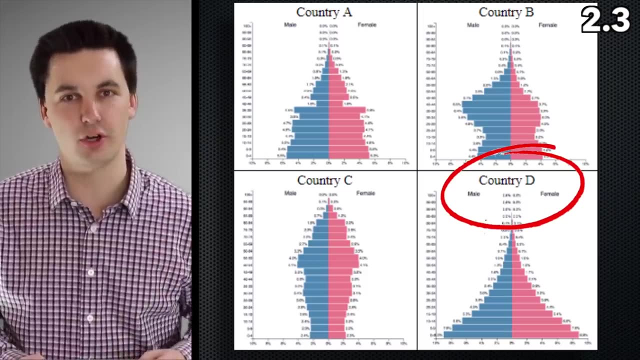 need a lot of help around the farm, around home. This is the one that's going to have that large population growth and is more likely to have an agricultural-based economy and less urbanization occurring Now. question three is about immigration and which one of these countries has the most. 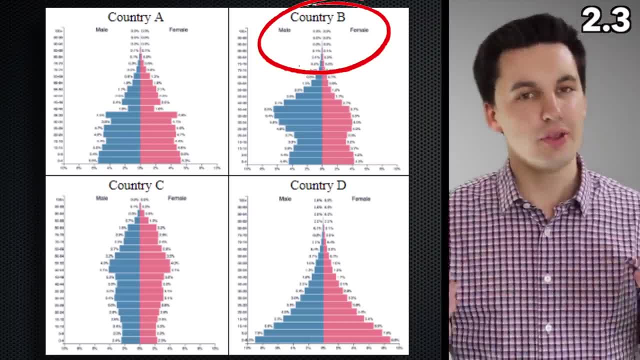 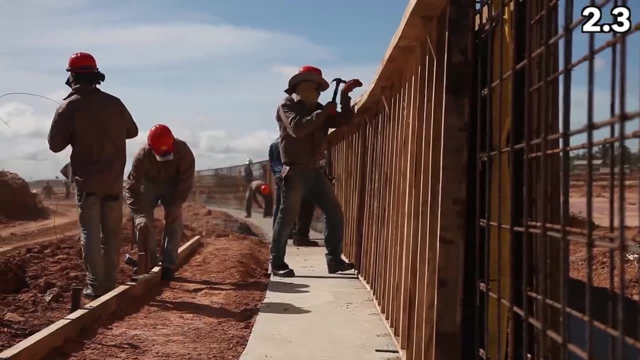 immigrants coming into the country. You can see when, looking at country B, this is going to be our answer. The majority of the men that have come into the country are around the working ages. This would lead me to think that they're having some guest workers. 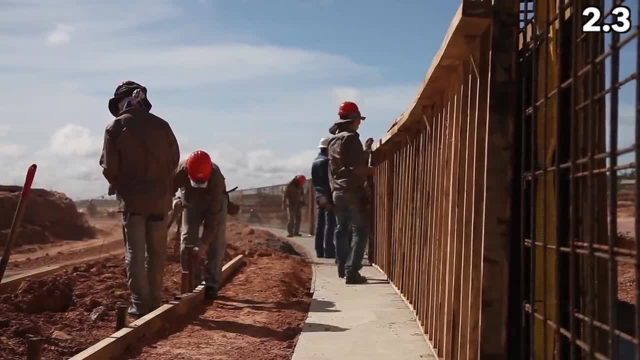 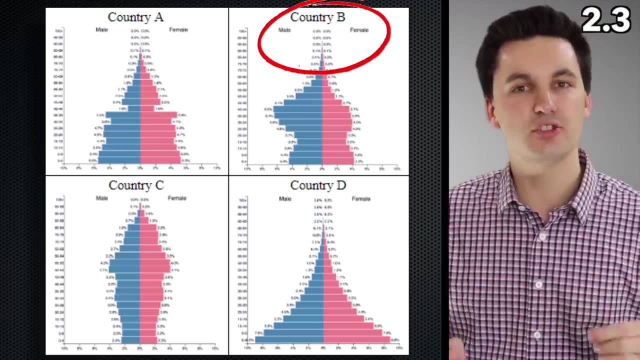 People come in when they're in that working age There's a lot of economic opportunity and then once they hit that retirement age or they start to get older and are leaving that working age, then they start to leave society. So guest workers would be a very logical conclusion here. 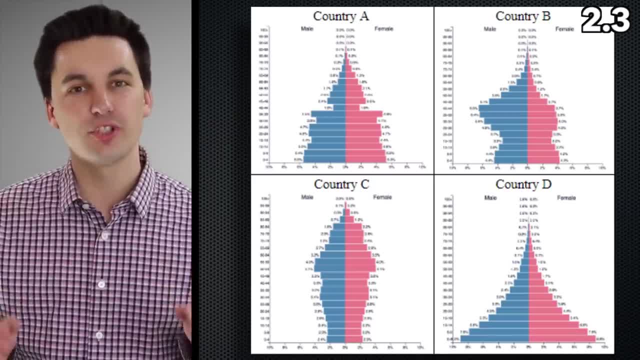 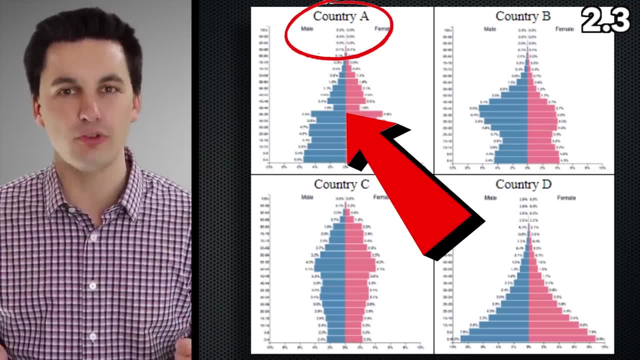 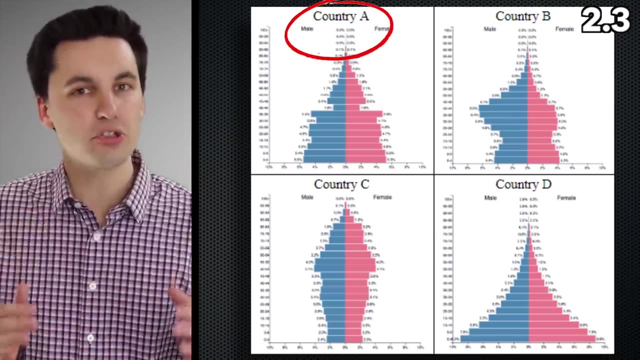 Question four is another tricky one as well: Which one of these countries would most likely experience an internal war? But the answer is: A look closely at the age ranges between 40 and 44. You can see a big drop off. What that would show us is, since it's both men and women, it's more of an internal struggle. 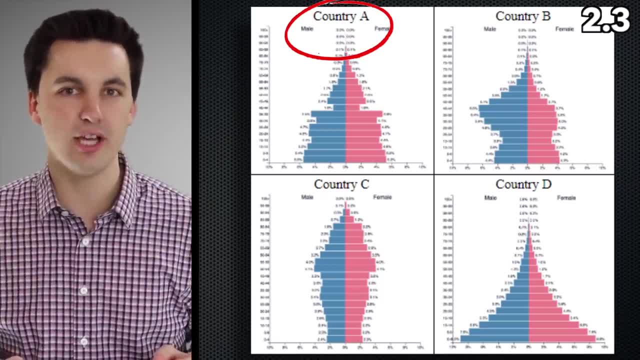 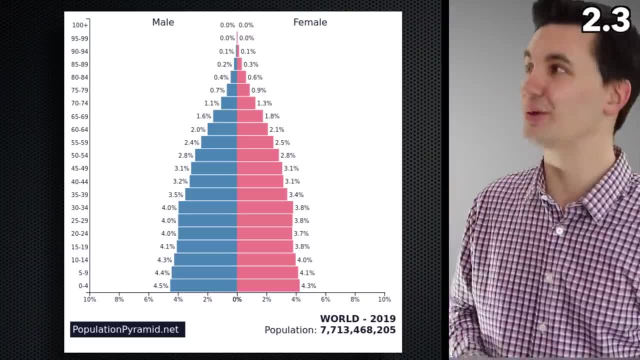 Both of the genders that are impacted, and it's just for this one period of time again, that 40 to 44 range. So that would be why this one would show more of an internal war. Kind of cool actually if you think about it. 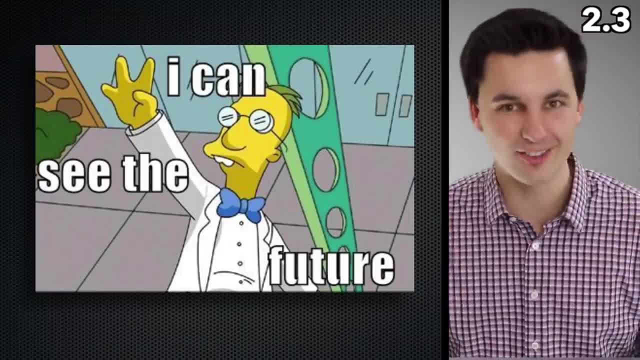 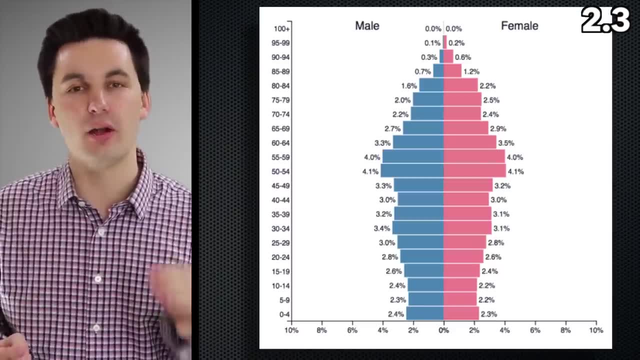 You can see back in time with these things. You can also see in the future. They're awesome. So question five now is looking at which one of these countries might have a baby boom occurring. This is going to be C. Look at the age ranges around 50 to 55.. 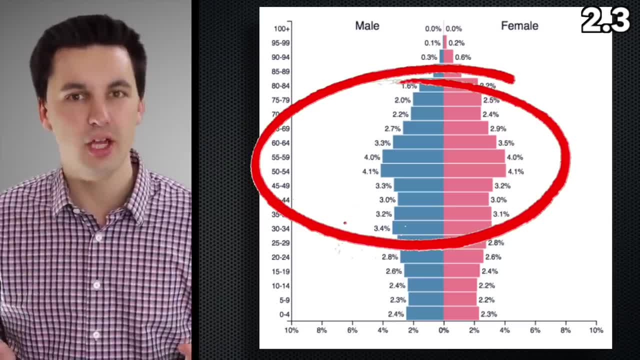 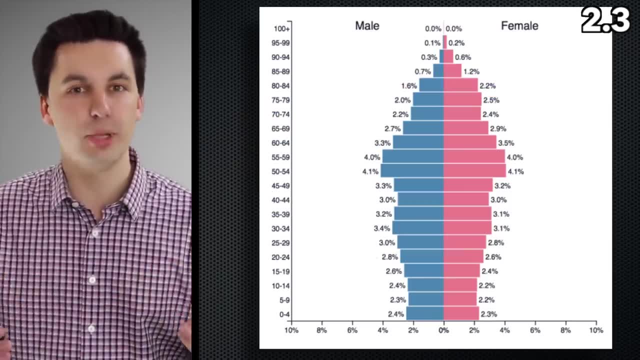 Here we can see about a population increase around five- 6%, where we're seeing this big boom and then it dips back down. There's a bunch of different reasons why it could occur. A lot of times it's a war or some big event. 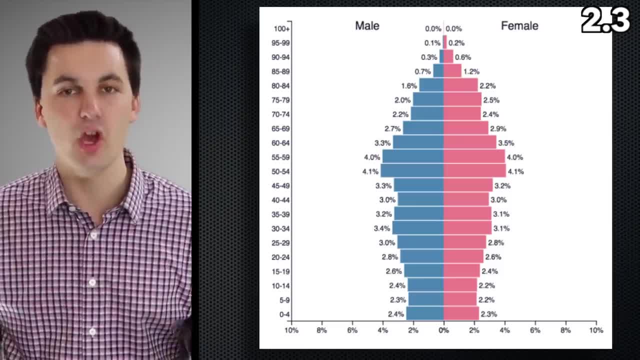 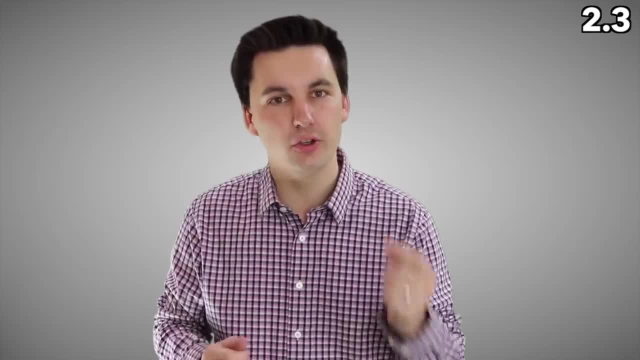 Actually, right now there's speculation of: will the COVID-19 virus cause a population boom? Are you starting to get it? Hopefully this is helping Here. you can see a bunch of different ways. we can make really good inferences just by looking at these population pyramids. 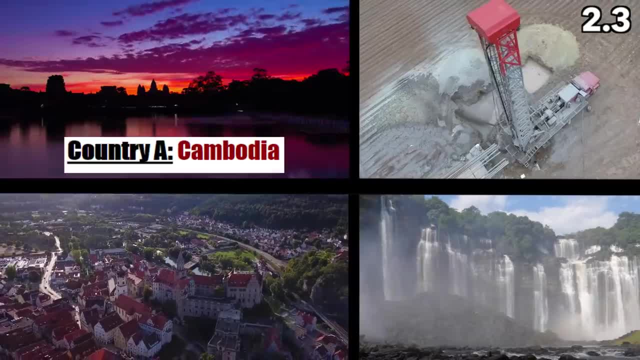 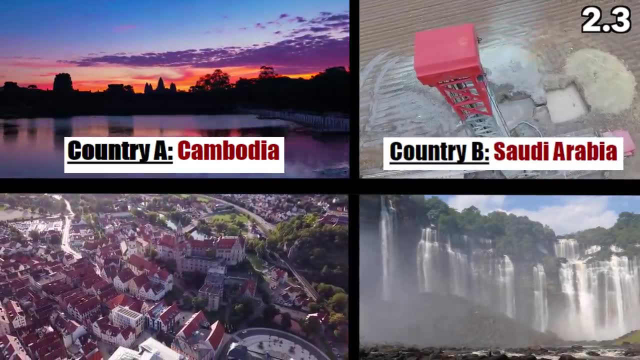 All right, GRI-verse. the time has come to reveal these countries. Cambodia's country A- you can see that internal civil war. Country B is Saudi Arabia. That's actually looking at the oil production. When we're looking at those guest workers, a lot of men are coming to work in the oil. 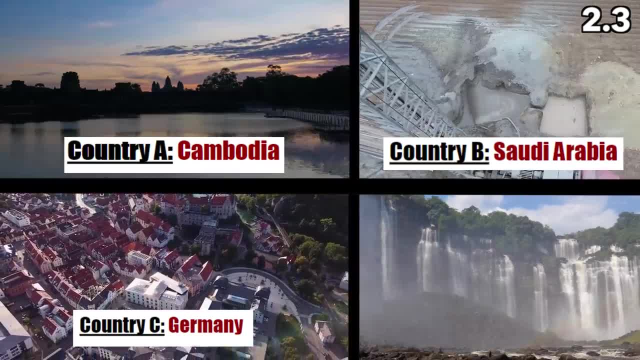 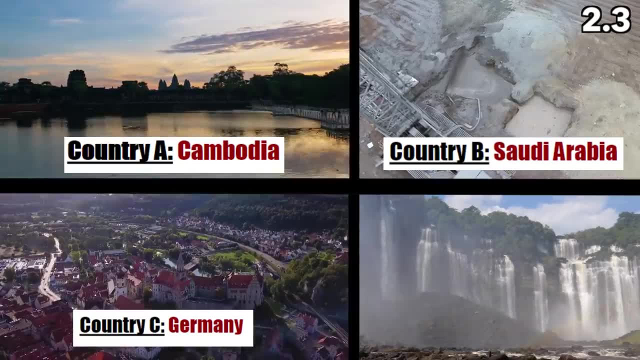 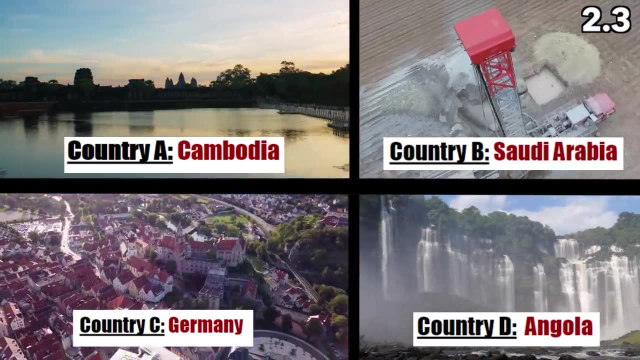 fields, the rigs, and then they leave. Country C is Germany. Germany's a lot more advanced and they're actually struggling right now with population growth. They're trying to increase it because their population is starting to dwindle. And country D is Angola, where we have a large base, lots of population growth happening. 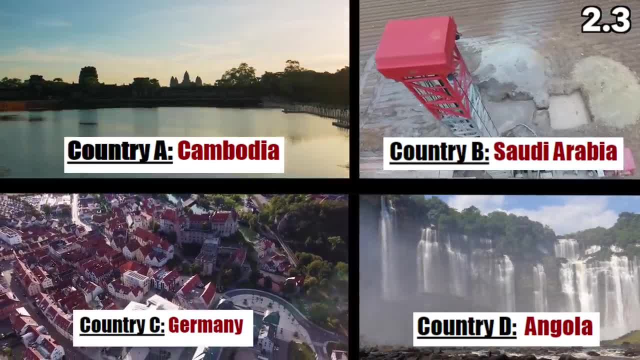 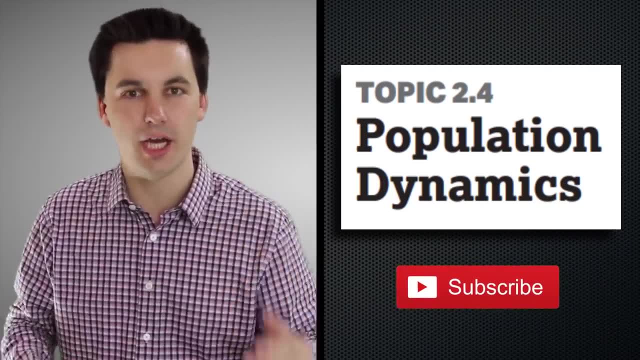 still in that stage, two stage eventually going into three and we're starting to see some changes. So 2.4, with our population dynamics, is looking at the CBR, the CDR, the TFR, the NIR. This is going to be the basis for the demographic transition model. 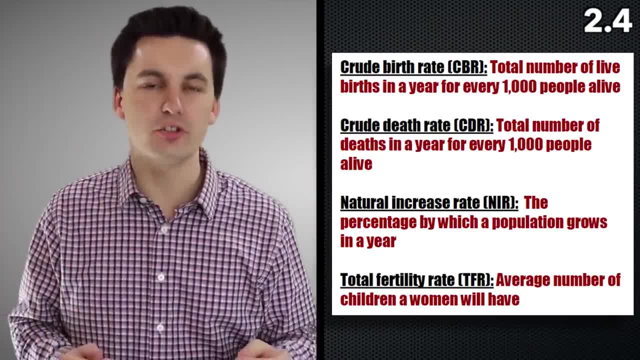 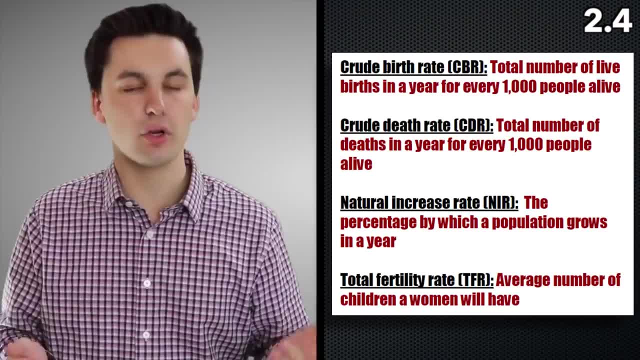 These are the technical definitions, but it's more important to understand these concepts. See how many people are being born compared to how many people are dying, And if that's a positive number, we have a positive NIR. Our natural increase rate is going up. 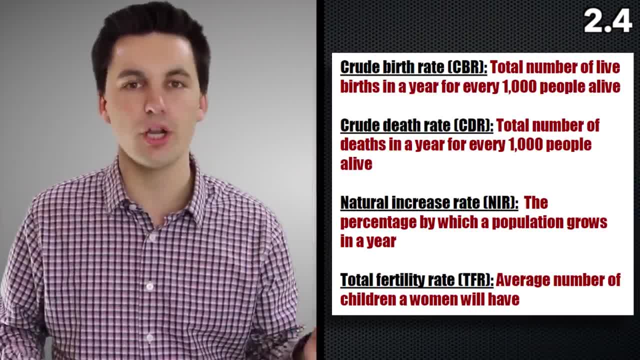 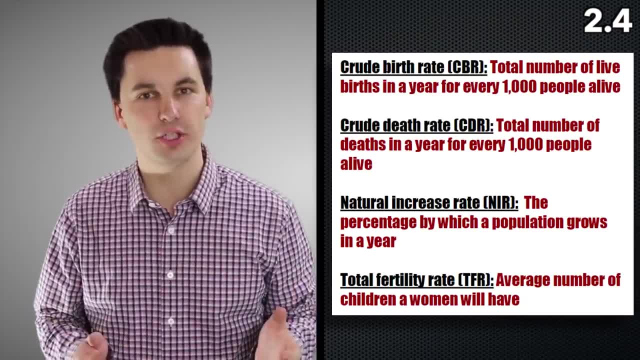 We're growing. If it's negative, more people are dying than being born and our society is getting smaller. One of the areas where students get confused is when we're looking at TFR- our total fertility rate- and CBR- our crude birth rate. 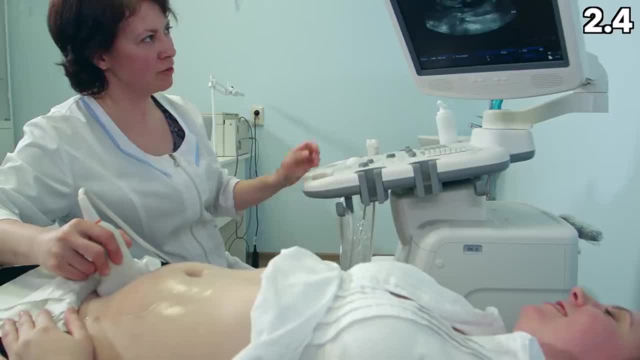 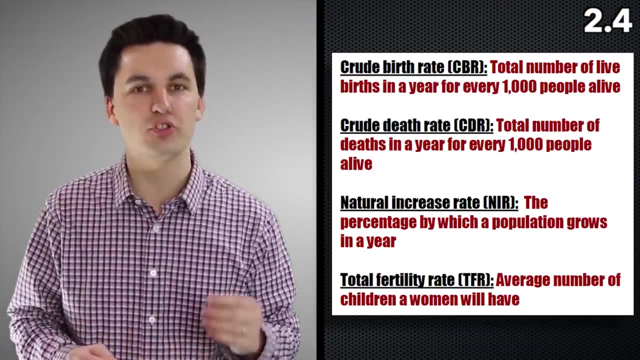 TFR is looking at the average amount of children born to each woman. where crude birth rate, our CBR, We're just looking at how many people are being born in society. Now. TFR is important for geographers because here we can see if our population is really. 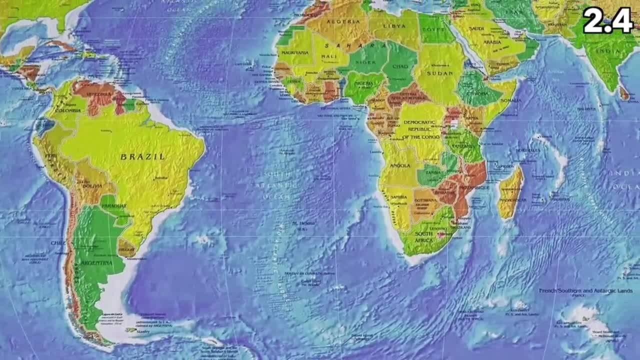 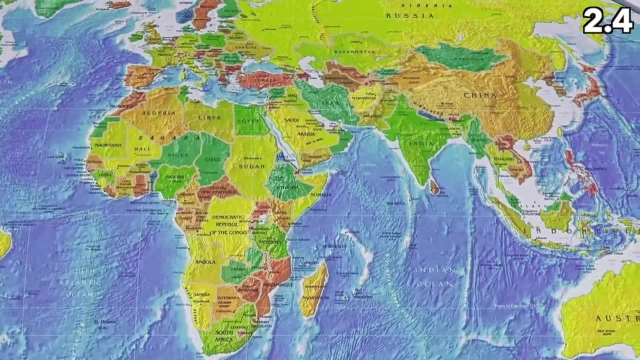 going to be able to sustain itself. A TFR of 2.1 is the replacement rate. This means we're not growing but we're also not shrinking, And it's known as a concept of ZPG- zero population growth. We have stabilized. 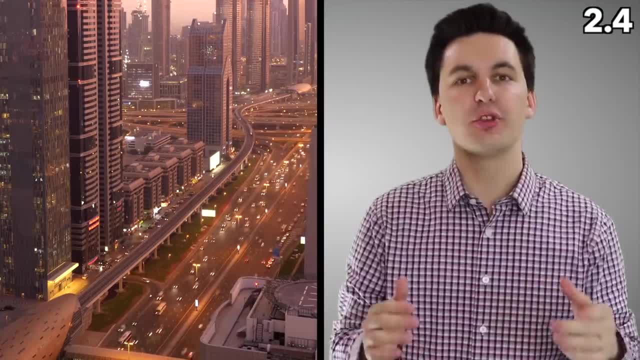 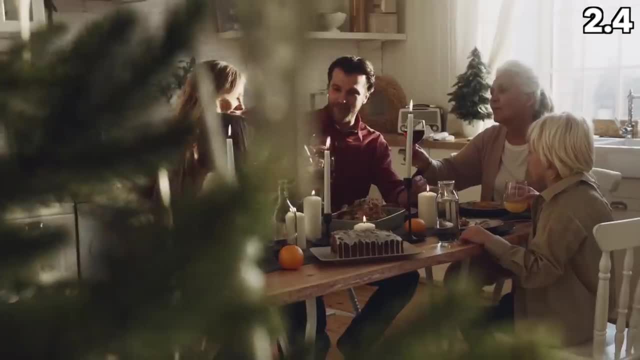 So 2.1 is our replacement rate. That again is our TFR. One of the things we can also see when looking at societies is, as their economy advances, as they become more developed, We start to see people living longer and deaths go down. 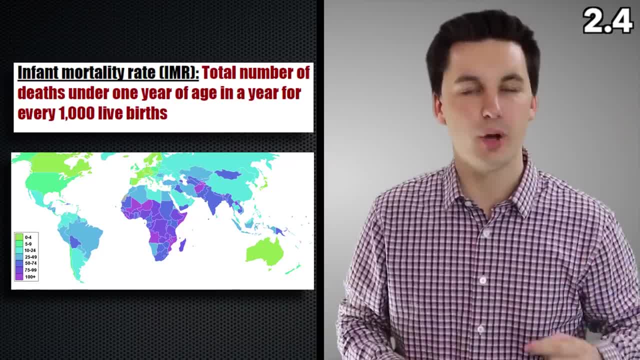 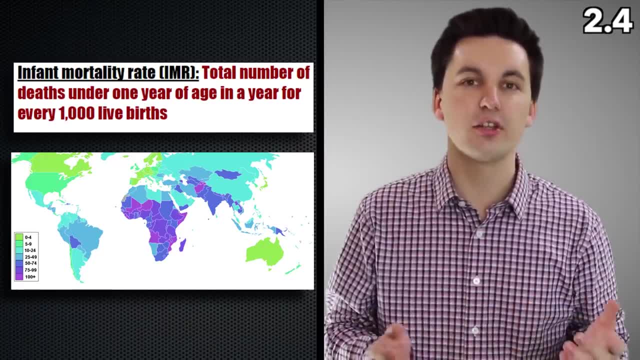 And there's a bunch of different reasons for this. One is our IMR decreases, That's our infant mortality rate, And this is more of a sad metric, but it's looking at the kids who die, particularly under the age of one. 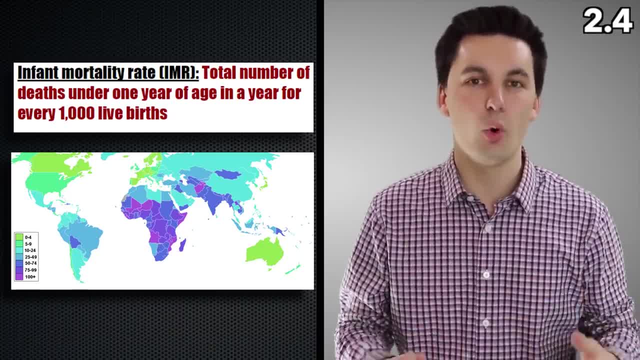 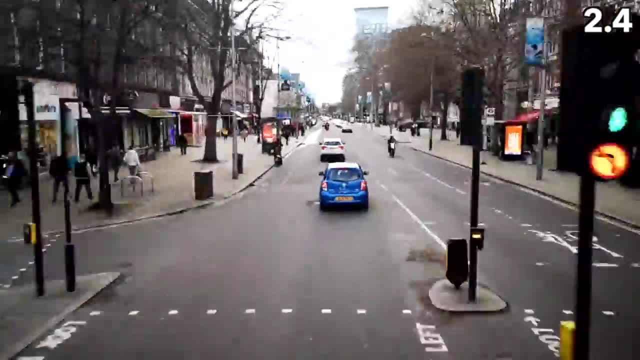 Infant mortality rates. if it's higher, that means we're going to have more large families, because people are going to have kids, expecting them not to all live Countries that are more economically advanced see more rates of urbanization, which leads to more people living in city. 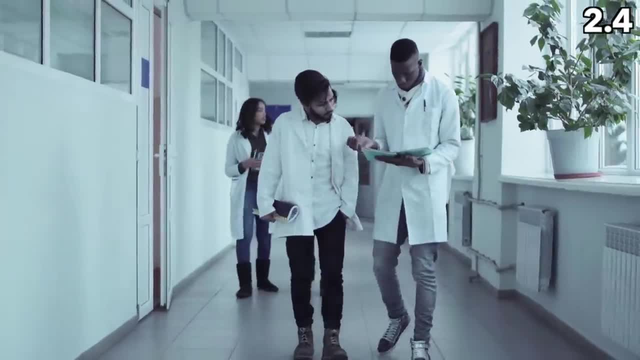 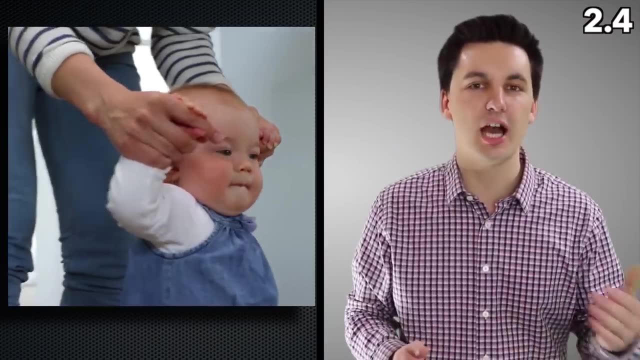 It'll lead to, then, the creation of hospitals and clinics, And since the citizens are now wealthier and they have more access to capital, they're able to pay for these things. We also see things like the IMR decrease because of a new focus on education on healthcare. 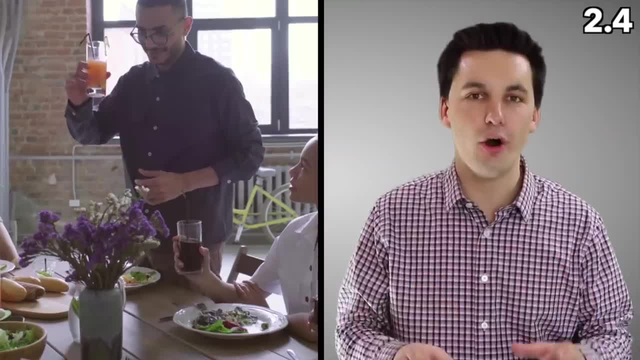 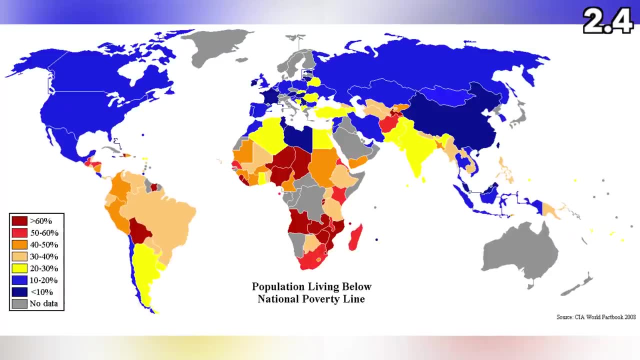 practices and people are more informed, making better decisions, And all of this allows us to have better standard of living and reduce our death rate, which is great. Countries that don't have as strong of an economy are more likely to struggle with population. 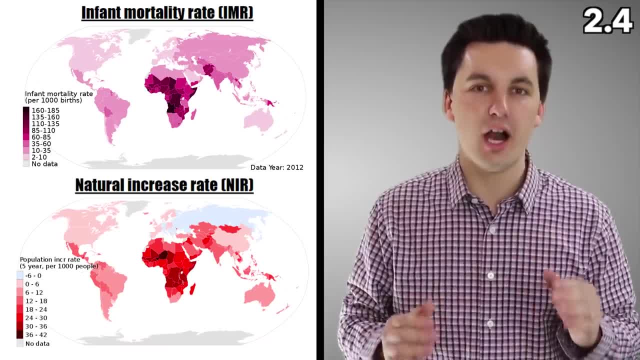 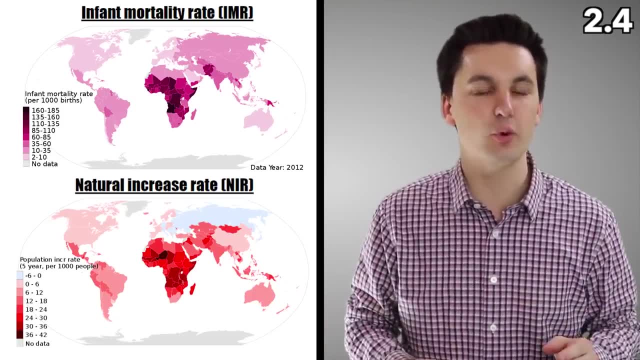 And that's what we're seeing. They're going to have population growth and they're going to have a higher IMR. That death rate, then, of the children is going to lead to more births happening, And this means countries have to worry about doubling time. 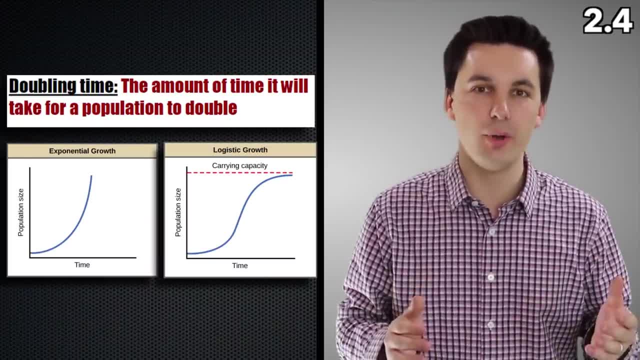 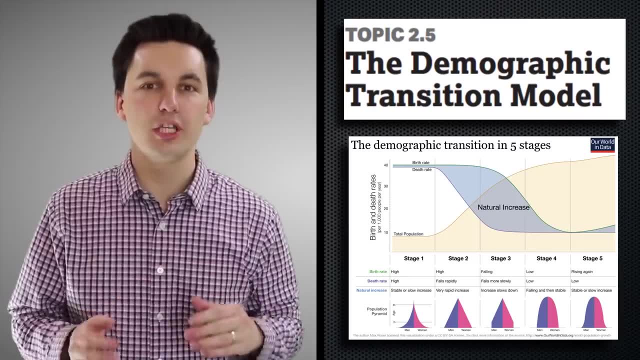 Doubling time is just the concept of how long will it take for the current population to double in size. All right, now we're going to talk about the demographic transition model for 2.5.. Here we're going to be looking at the NIR, the CBR, the CDR. 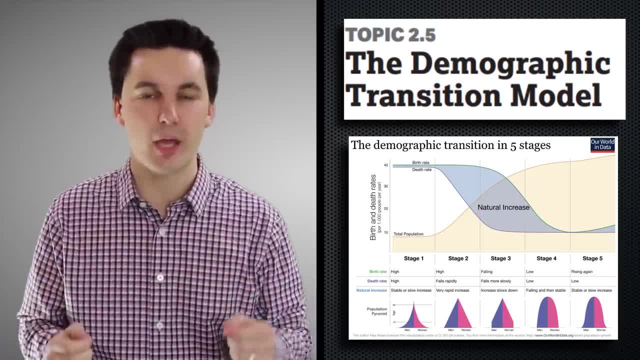 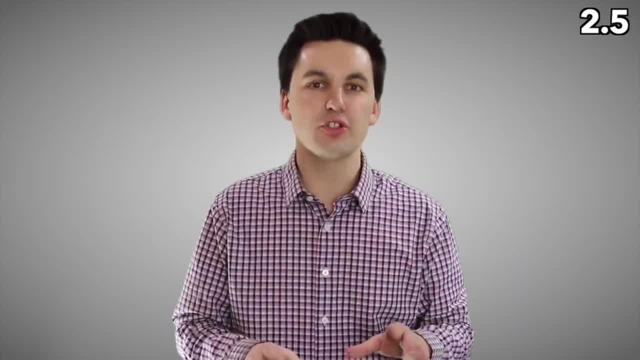 All these things are coming back and we're going to be talking more about economics and the impact on population growth, The most important thing in this unit, because it connects to almost everything. what I want you to do right now: pause this video, go through this section of the study guide complete. 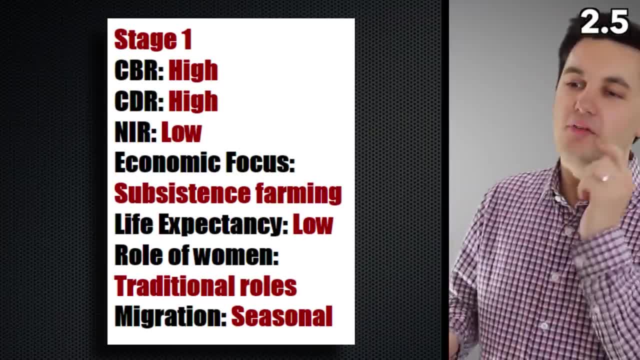 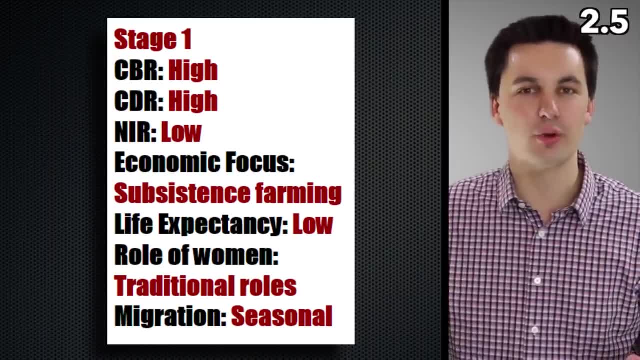 it, Then what we're going to do is quickly break this down. Stage one: we can see we have a high birth rate. Our total fertility rate is high. That CBR is high. Lots of people are having children And that's partially because our death rate is so high. 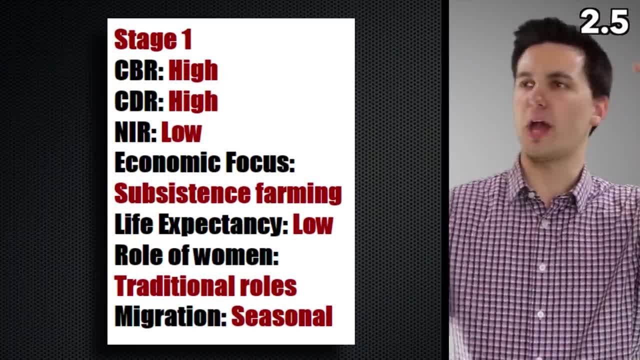 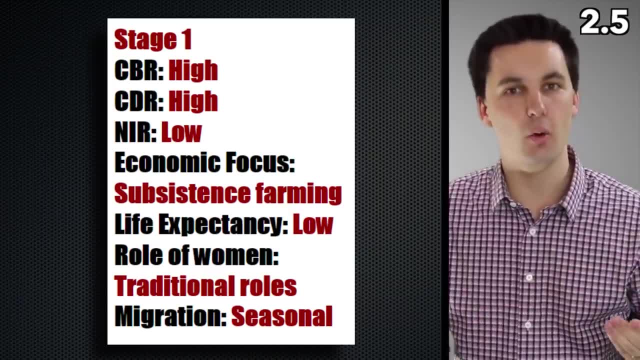 You're dying practically to anything here, Because our births are up here and our deaths are up here. Our NIR, Or our rate of natural increase rate, our RNI, is actually really low. Societies that are in this stage are also going to be focusing on things like subsistence. 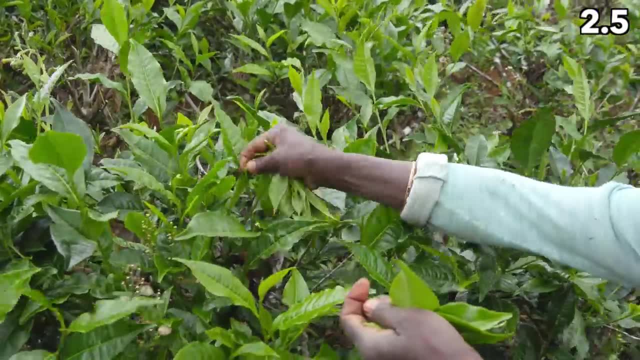 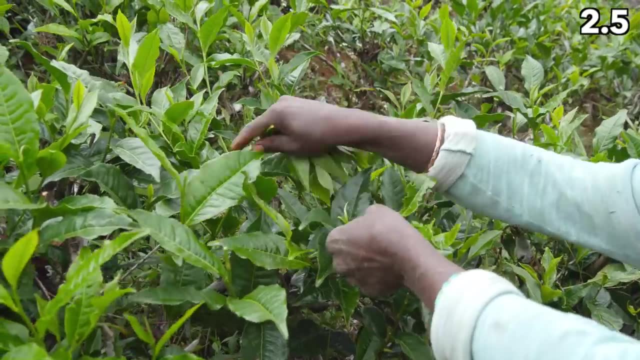 farming. We're not going to see a large production. You're focusing on just providing for your family And when looking at life expectancy and our health, we can see our knowledge is really limited. People don't really have a good understanding of medicine yet. 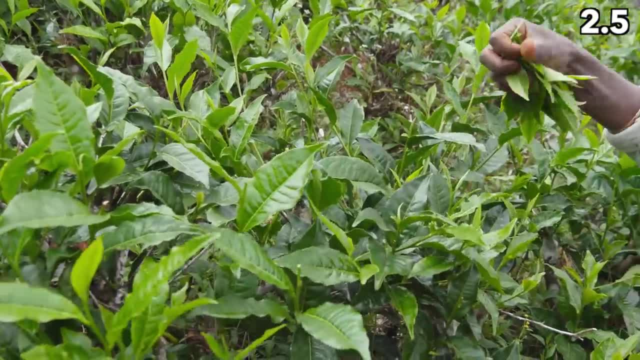 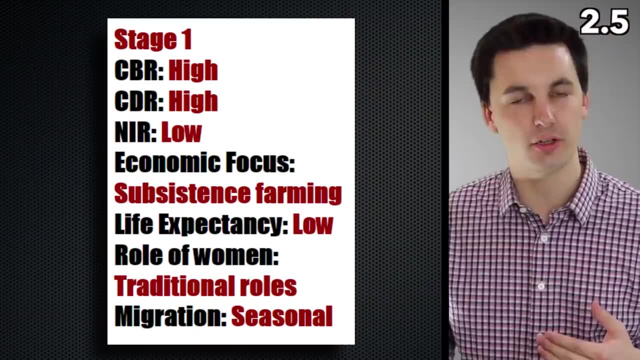 And so that also leads to more deaths. Women in stage one are not allowed a lot of opportunities within society. Society's going to view them in a very traditional way, As just mothers and caretakers For migration patterns. we could look at Zielinski, who created a model that focuses on the demographic. 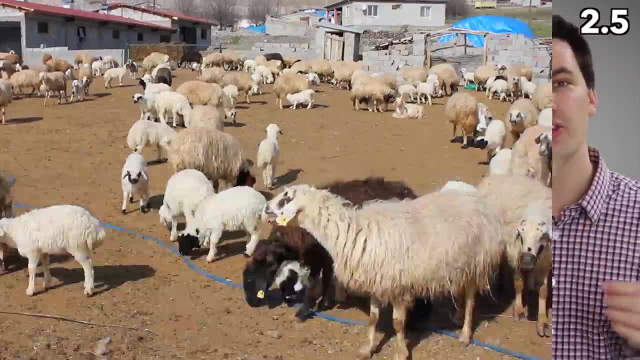 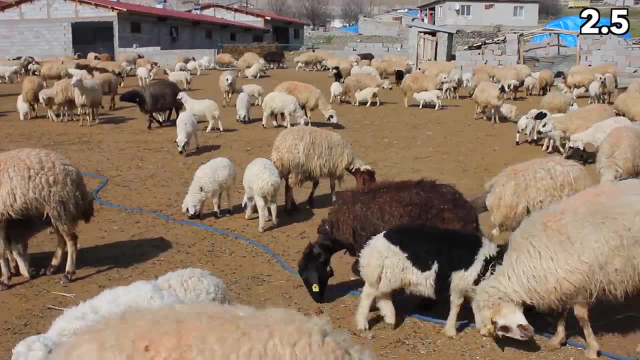 transition model. People migrate for a bunch of different reasons, But in stage one they're migrating essentially just far enough to get what they need. They're just going to be going along with their food source. So a lot of times it's seasonal migration that's occurring in stage one. 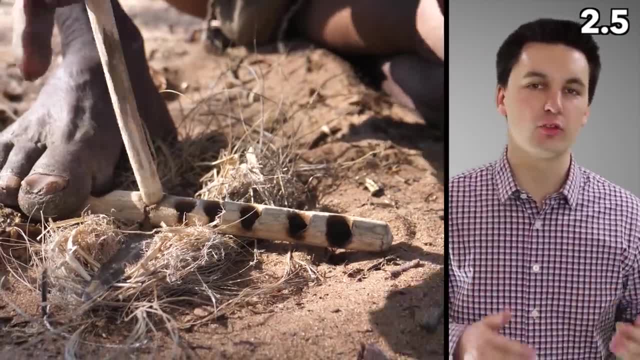 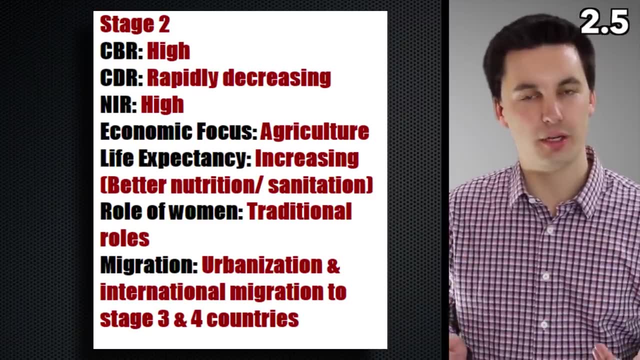 There is no country in stage one. Stage one is more isolated groups: hunters and gatherers, nomadic people. Stage two starts off pretty similar to stage one, With a very high birth rate. Now what starts to deviate, though, is our death rate. 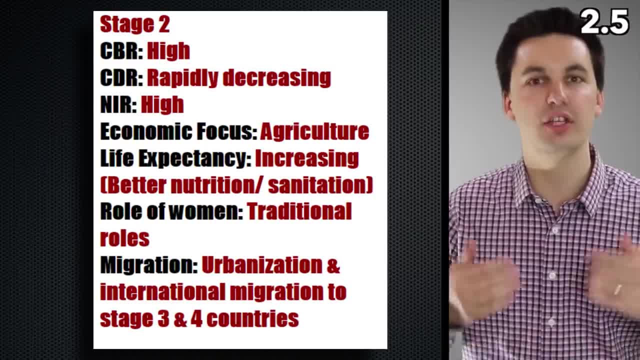 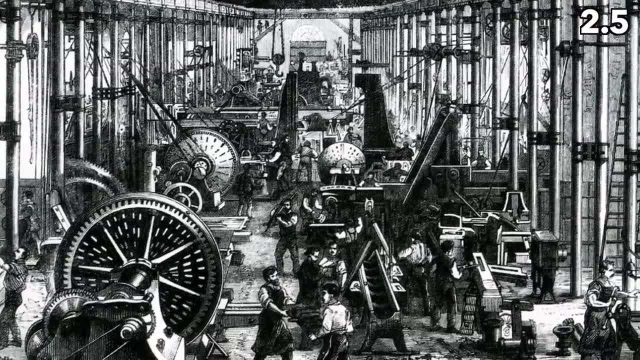 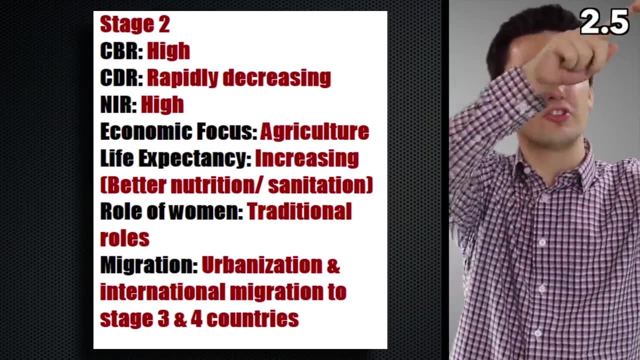 Our death rate actually starts to decrease. That's because we've now had the industrial revolution that started to occur, The medical revolution that started to happen. Less people are dying, but people still don't realize that All of this leads to a very high RNI, where our births are now up here but our deaths 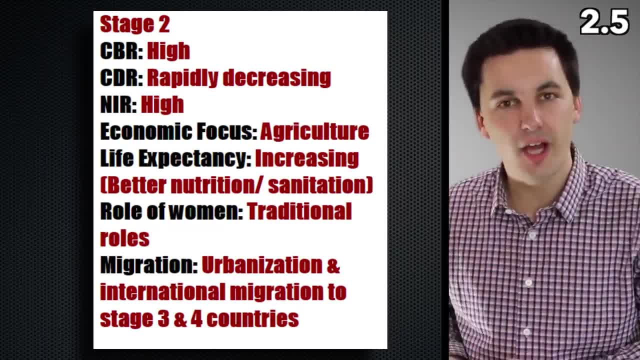 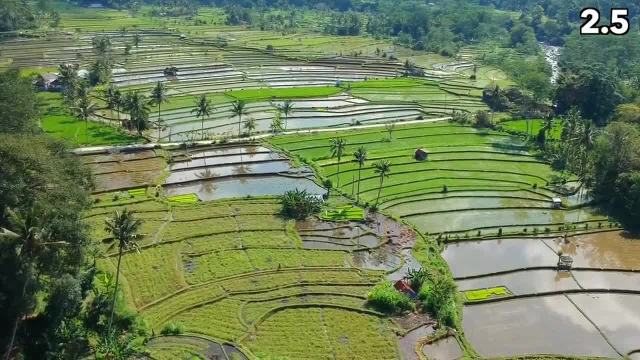 have decreased, And so now more people are being born than dying. Now, with this big growth, we still see agriculture as a main focus. Ultimately, though, now it's for trade, So we're starting to see more production of food, and health gets better as well. 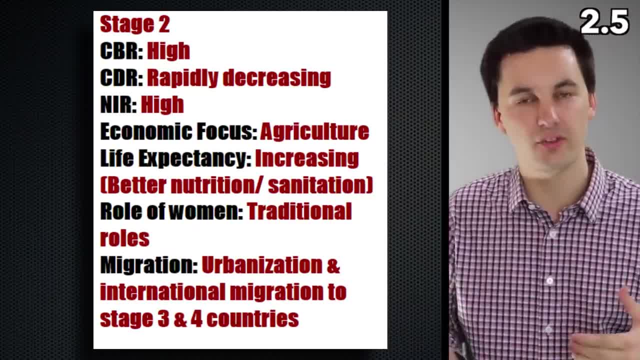 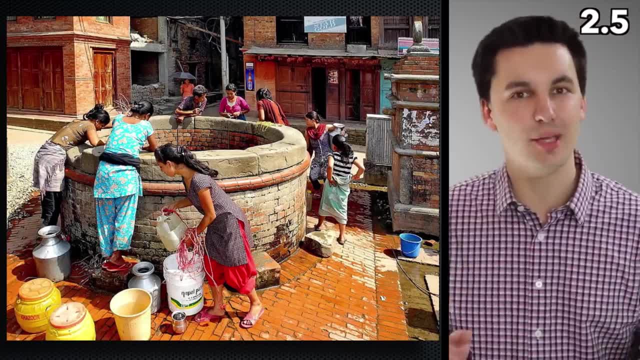 As things like the medical revolution start to change the concept of medicine, we start to see slightly better living conditions and society starts to advance. Women, unfortunately, though, kind of stay the same here. They're still viewed as mothers or caretakers. 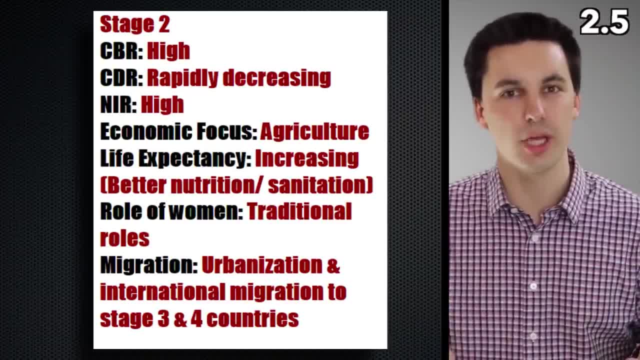 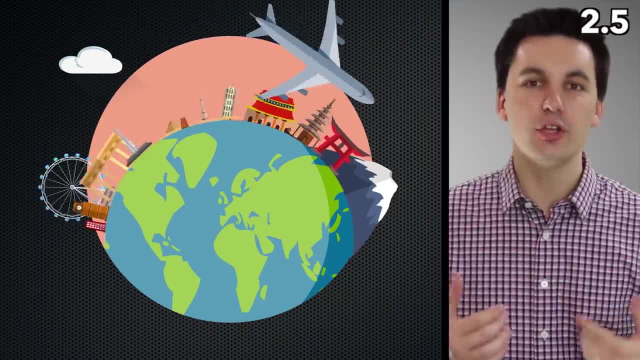 Lastly, we start to see our migration patterns actually shift a little bit, Connecting back to Zelensky's model. people are more likely to move to a stage three or stage four country, And that's because they're looking for job opportunities. 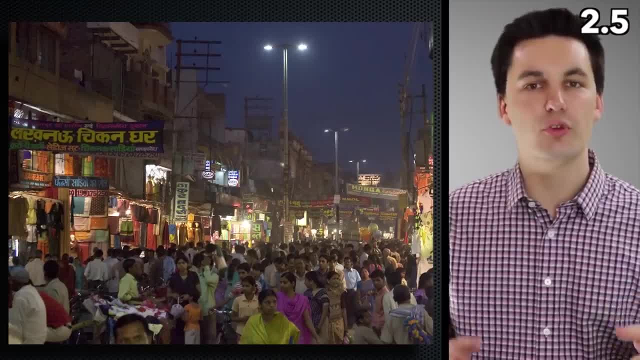 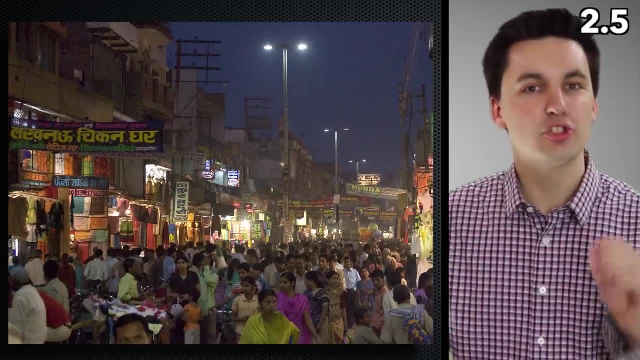 If they are going to stay within the state, they're more likely to move from rural communities into urban areas. So more people move to where the businesses and the jobs are, And that reminds me. before I forget, make sure you know the difference between inter-regional 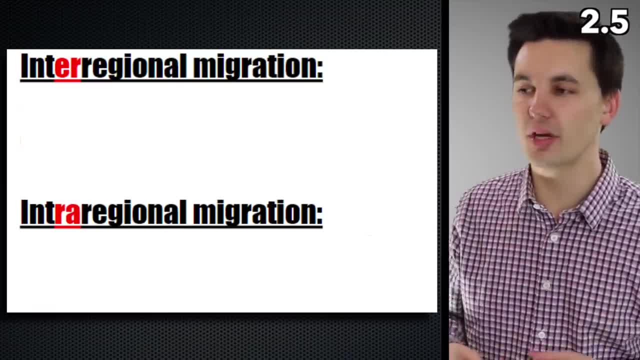 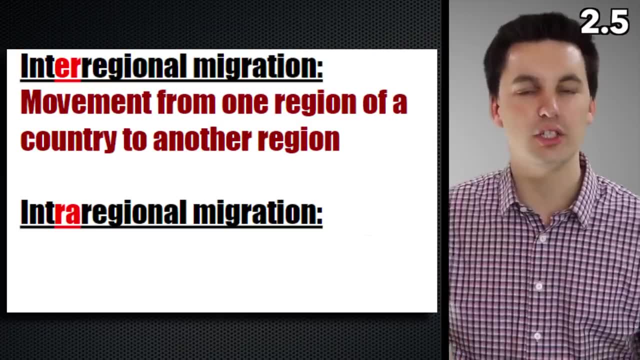 migration and intra-regional migration. Inter-regional migration is when we're moving from one region of a country to another- Now we're staying within the same state- while intra-regional migration is when I'm staying within the same region. That would be. 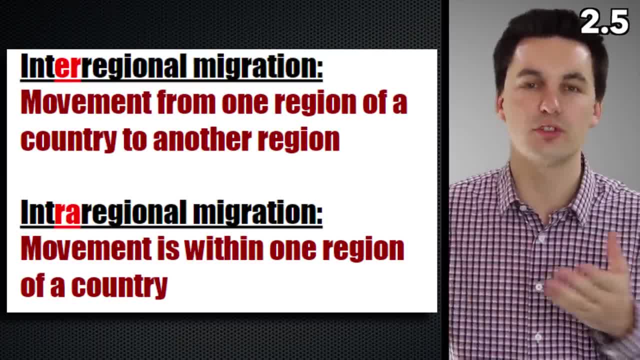 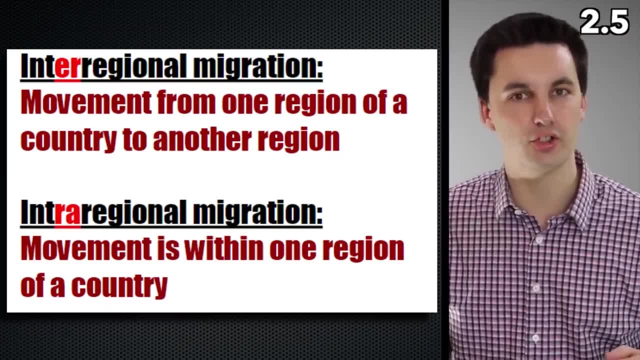 I don't have to live in the cities anymore and maybe move to the suburbs, or I moved into the rural community or vice versa. So we can see, in stage two we actually start to see people moving with intra-regional migration, moving from the rural life into urban life. 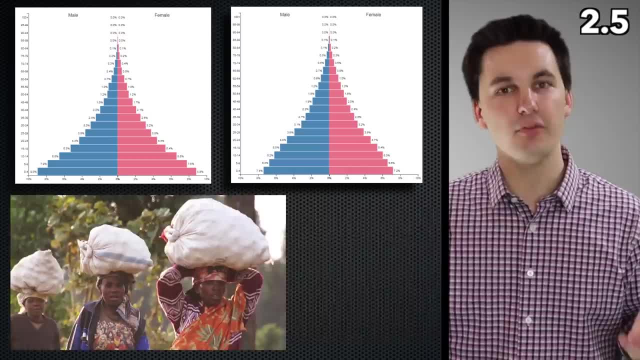 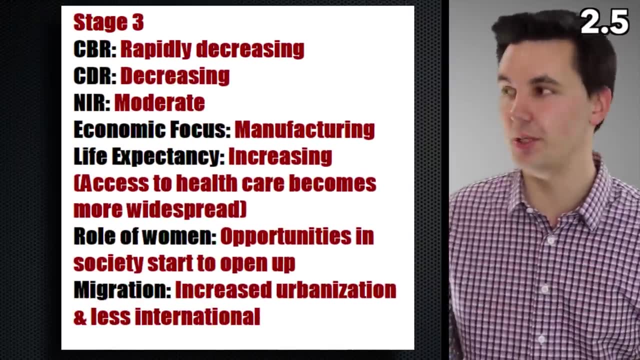 Modern examples for stage two is Angola, Sudan. Actually, a lot of Africa currently is in stage two, starting to transition into stage three. Stage three starts off with this like epiphany moment where people are like, oh hey, all these kids we just had, they're all living. 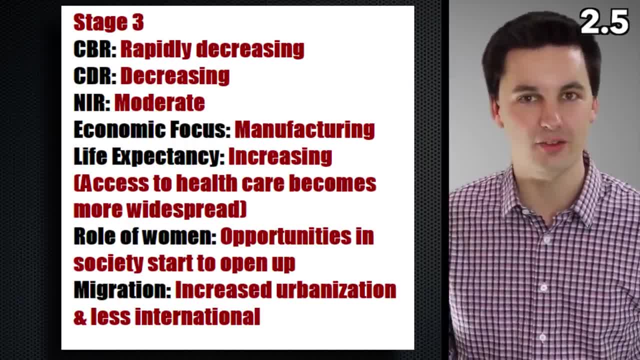 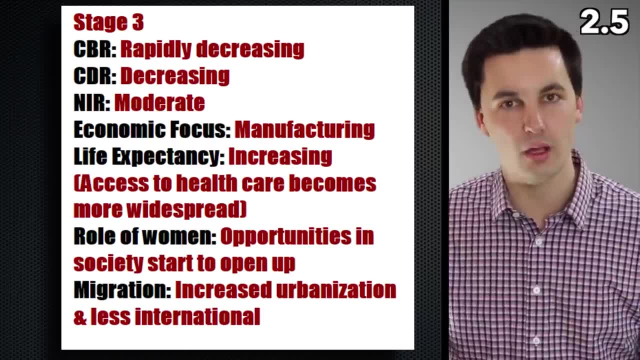 Now we got to pay for them all. We should probably stop having so many kids, And our birth rate really starts to decrease. More advancements are made, which allows our CDR, our death rate, to go down as well, And all of this finally reduces our population growth. 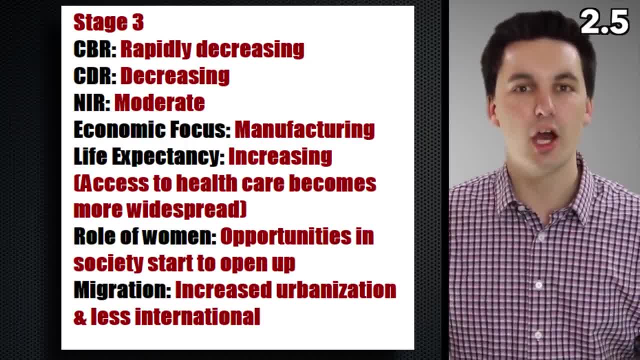 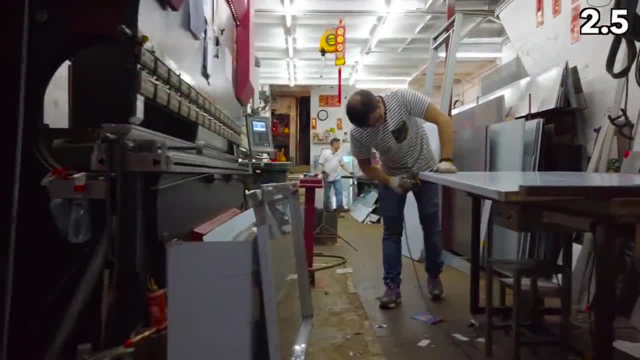 We start to see more moderate growth occurring here. The NIR has now gone down Due to the advancement of society. we see our economy really shift. It moves from agricultural practices to now focusing on manufacturing Factory. life starts to expand And our life expectancy starts to increase. 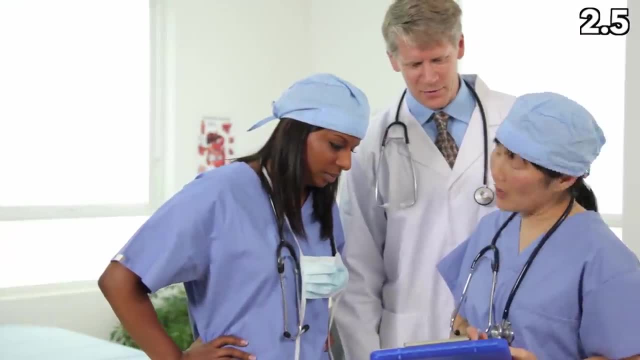 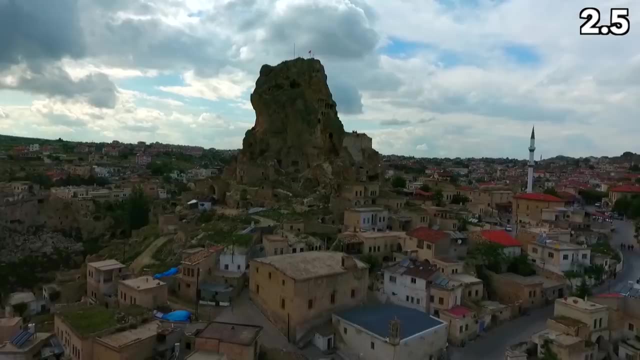 Even further As healthcare gets more complex, as more people understand things and we start to see more advancement. Now, sometimes, when we have large urbanization occurring, we can actually see that more people start dying And that's because of the crowding of cities and poor infrastructure. 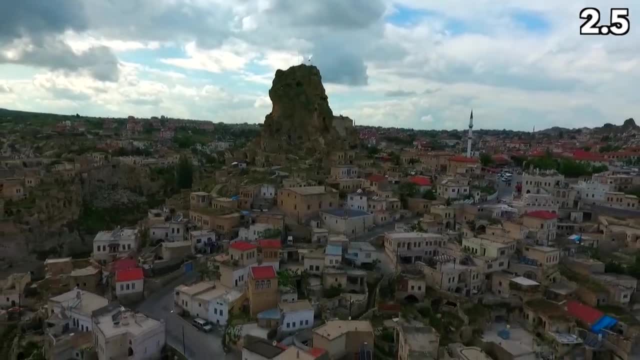 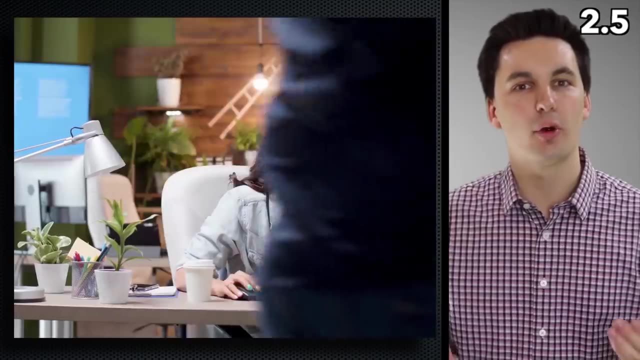 But overall, what we start to see is advancements in the medical field which allow people to live longer, healthier lives. Finally, women start to get more of a role in society. They're now making up more of the workforce. They're no longer just seen as child bearers. 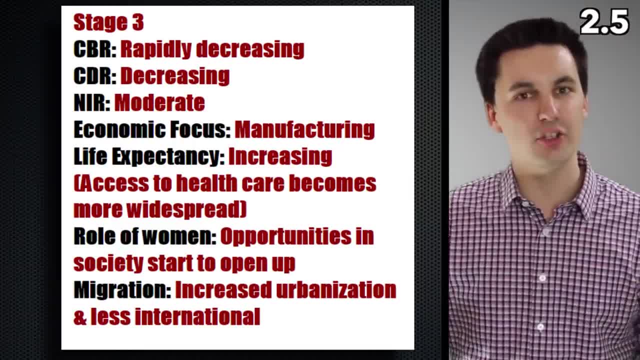 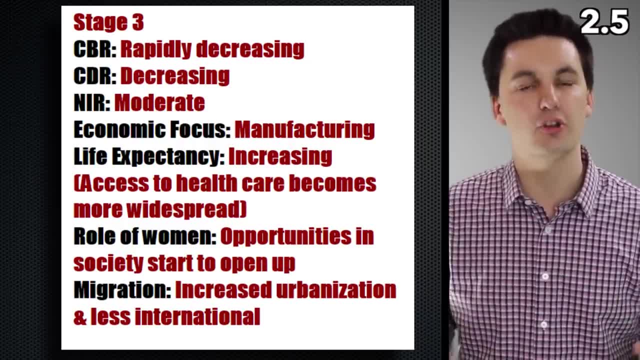 Or just taking care of their family Or taking care of the home, And our migration actually is pretty similar. still, It's starting to increase, though. More people are going to the cities As the cities expand and we start to see large urban areas and more and more workers. 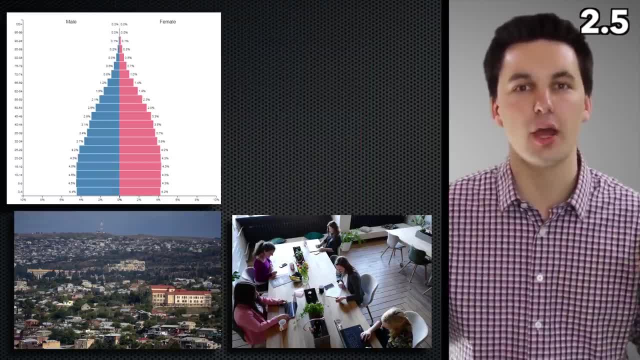 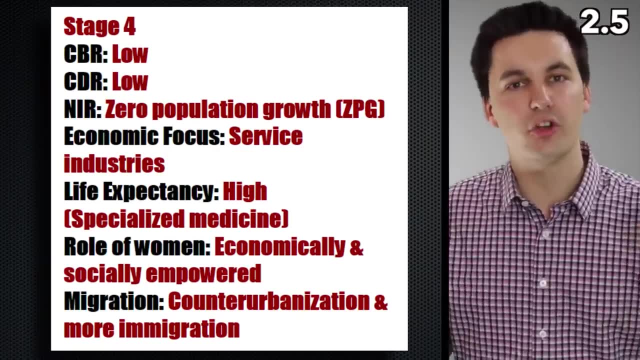 are needed. Modern examples for stage three would include countries like Mexico and Vietnam, where we've started to see population growth decline as they start to become more advanced. So stage four: our birth rates, our death rates have all leveled out. Kids have become more expensive. 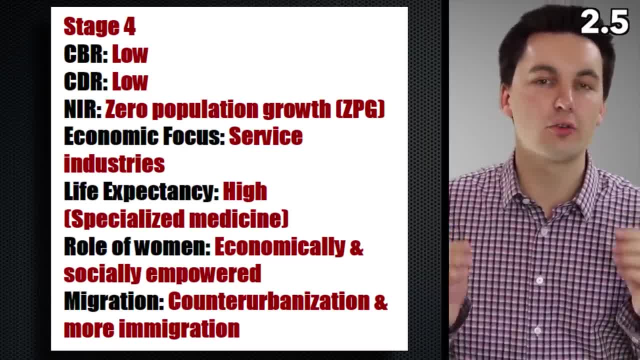 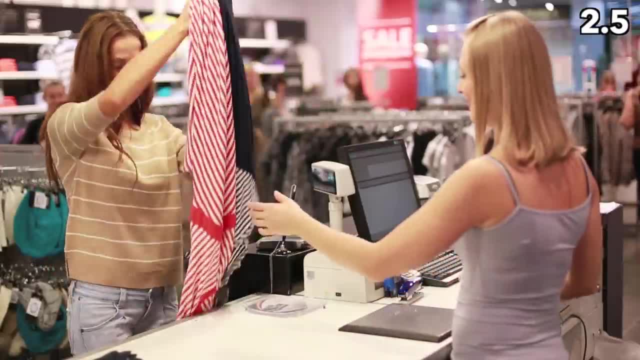 There's not necessarily a need for large families anymore And our growth rate is now down to ZPG. That's again that zero population growth, As we start to see more service industries take shape. we're even moving away from manufacturing as our economy becomes more complex. 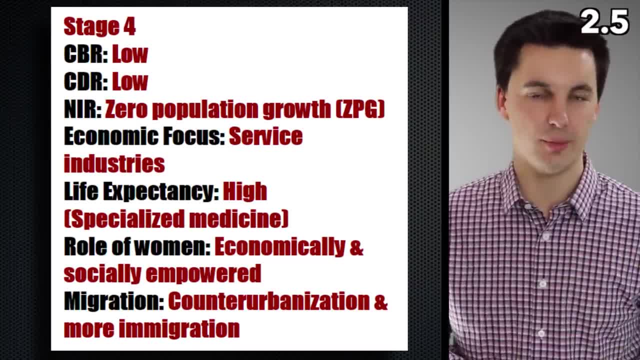 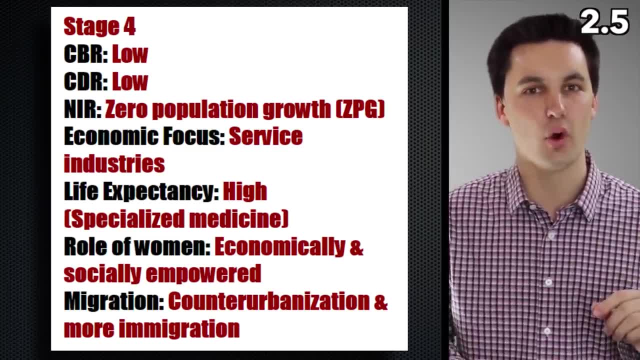 Our healthcare system continues to grow as well, along with the economy, And we actually start seeing more degenerative diseases as a main cause of death for people. in a state that is in stage four. People are living so long, the body's decaying. 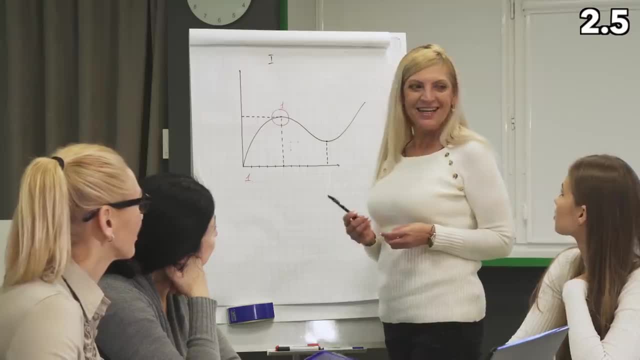 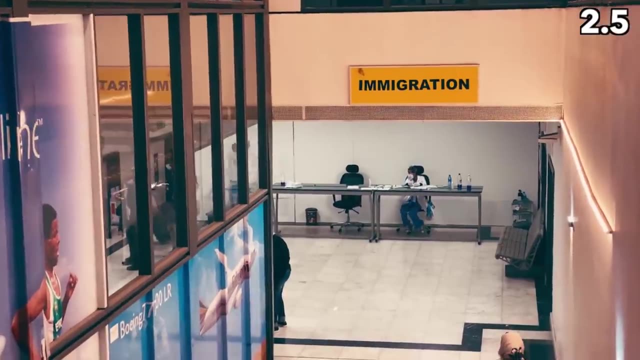 Women as well in society now finally have empowerment, Both economically and socially. Women are starting to now be treated the same as men. For our migration, we actually are going to see more immigrants coming from stage two countries and other countries that are developing around the world. 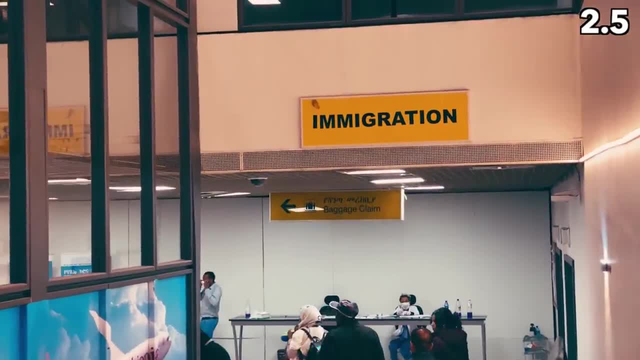 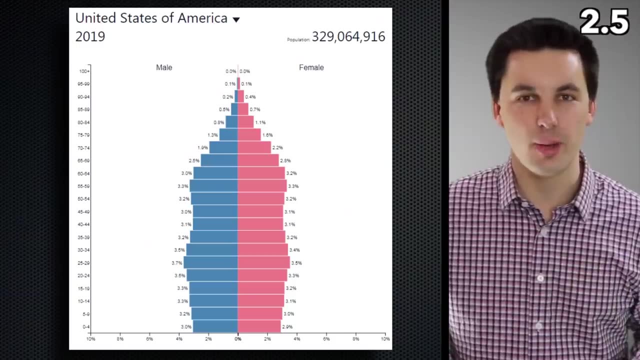 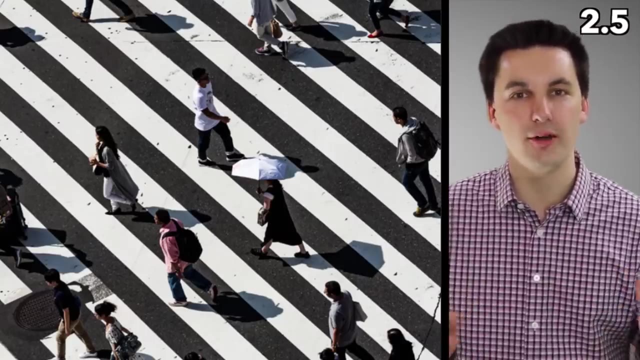 In stage four. there's just so much growth and so much opportunity for citizens, And we also start to see people move out to the suburbs. Modern examples for stage four would be the United States of America or China, whose economies have become really robust and their populations have really started to decrease and level. 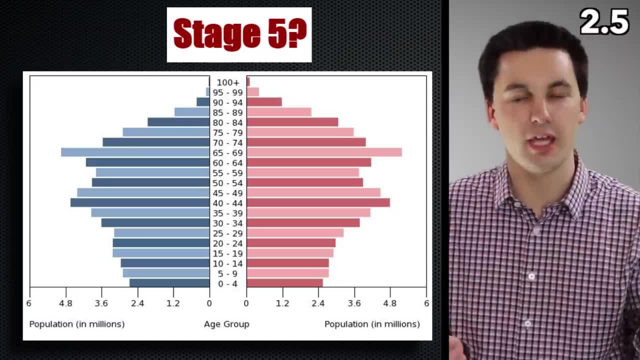 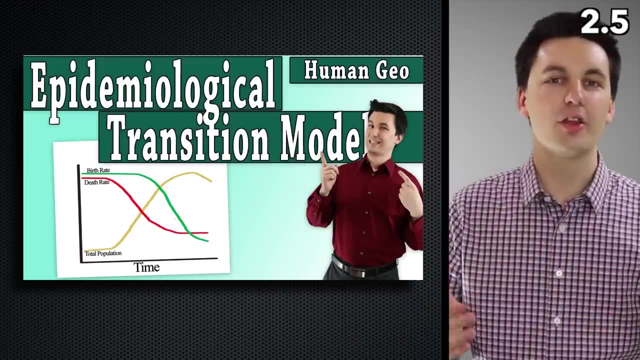 out. We've even debated stage five, where some people say, okay, this is when our population growth goes negative and we start to see our death rates higher than our birth rate. Another model that we can see connect with the demographic transition model is the epidemiological. 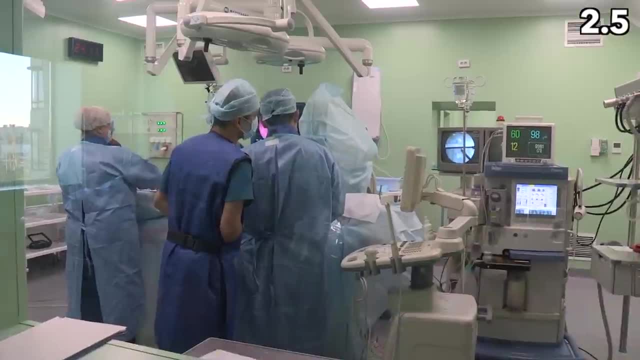 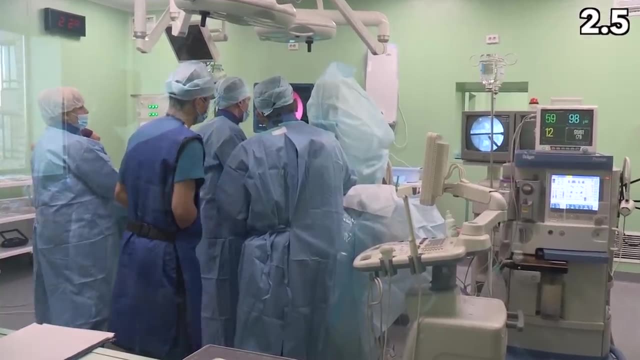 transition model. This one looks at how people are dying in society As we continue to advance down the demographic transition model. we deal with things like degenerative diseases, where people are living longer, eventually trying to cure and delay those For 2.6, we're looking at Malthusian theory. 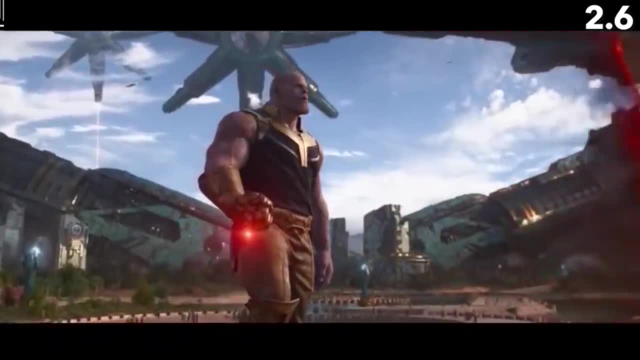 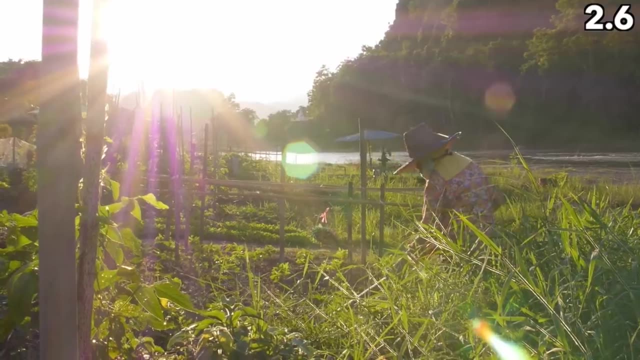 Or really we should be calling it Thanos' theory. Titan was, like most planets: too many mouths, not enough to go around. Thomas Malthus believed that our food production would grow in an arithmetic pattern, while our population would grow in a geometric pattern. He believed that we would reach a Malthusian catastrophe. There's not enough food to go around to feed everyone. Malthus believed that we would need the government or some act of God almost to stop this from occurring. Otherwise we would have major consequences for society. 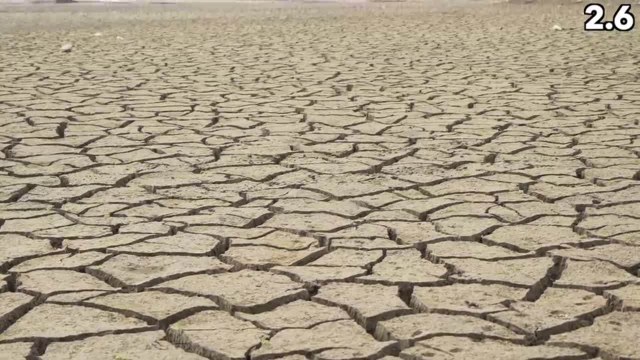 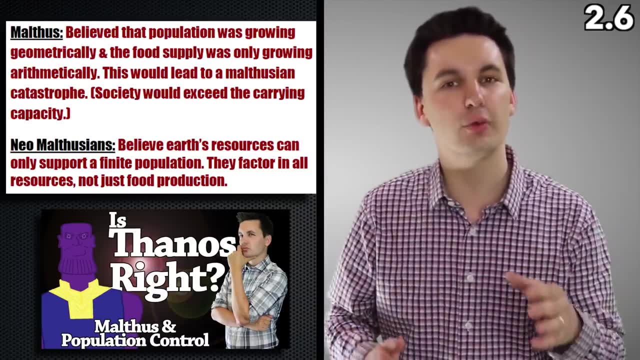 Eventually it will change into Neo-Malthus. These are people that take Thomas Malthus' idea and they change it a little bit. Malthus needed to focus more on the environment in general and our resources. That it wasn't just food we'd run out, of, it's all the other resources that we use for. 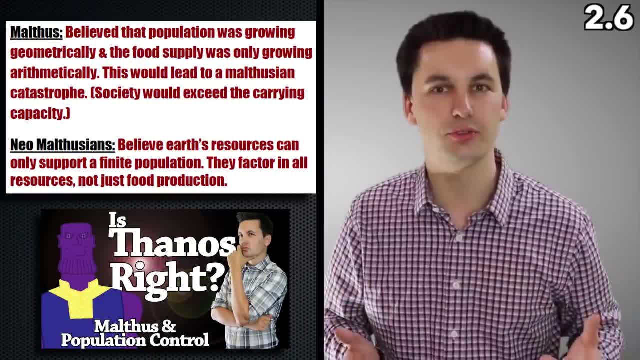 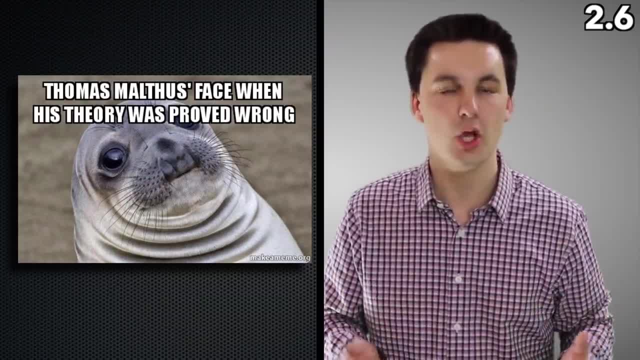 society to function. Thanos would definitely be a Neo-Malthus. Congratulations, you're a prophet, I'm a survivor. There's a bunch of different reasons why Malthus actually wasn't correct. What we started to see is, as society has developed, we start to see our population growth go. 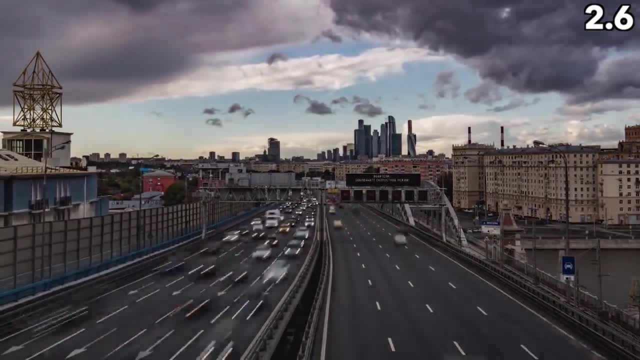 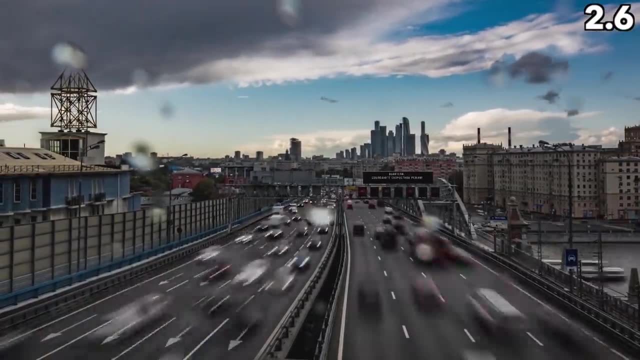 down. With the economy advancing, we start to see birth rates decrease. All of these different things prevent a Malthusian crisis from occurring. Malthus was around during stage two, so he was very focused on this high birth rate and our deaths decreasing. 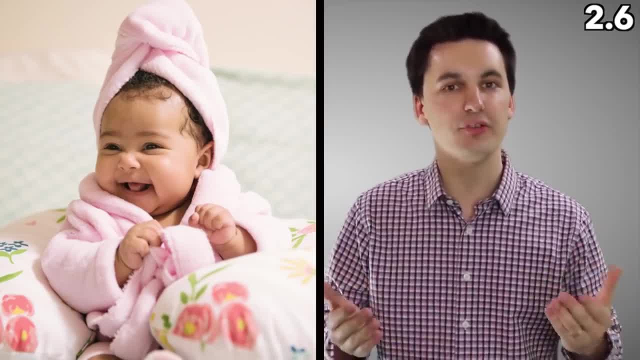 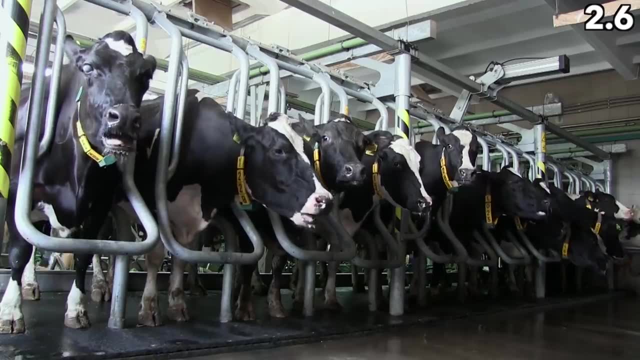 He was worried that this population growth would never end, But we definitely see it does. We also start to see that food production increases as well As technology gets more advanced, As we see things like the combine get created Or fertilizer and pesticides be used. 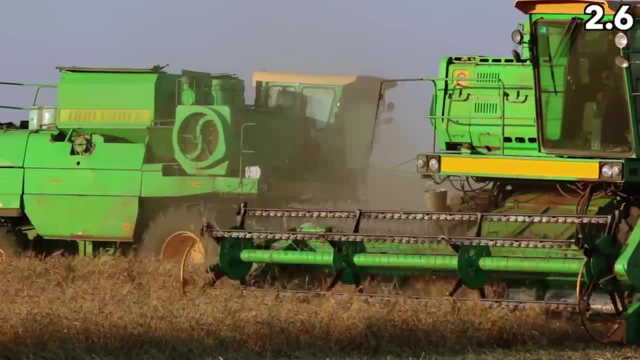 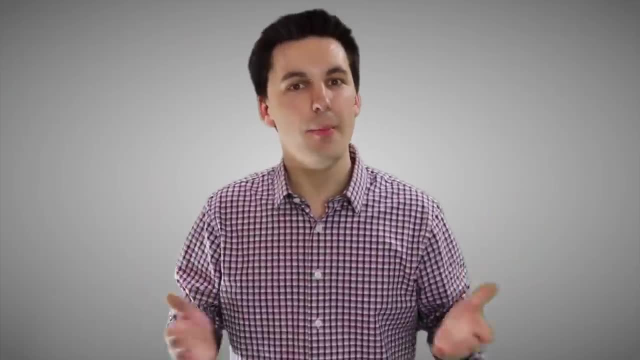 As we go through the agricultural revolutions, society is able to get higher yields from farmers, And all of this reduces then that chance of a Malthusian catastrophe. So Malthus turned out to be wrong. We're now going to move into 2.7, where we're going to look at population policy. 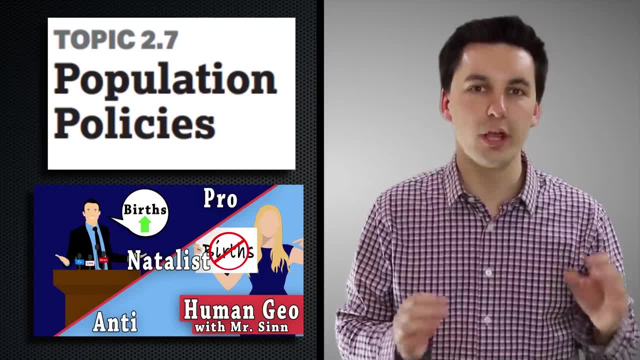 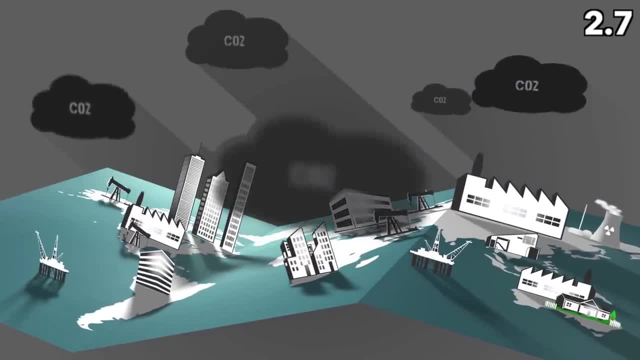 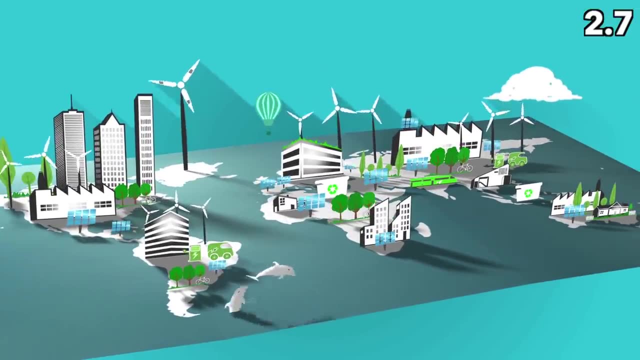 One of the reasons why governments even get involved in the first place with population growth is because of sustainability, Sustainability. Sustainability is just humanity's ability to satisfy the current wants and needs of society without negatively impacting the future generation's ability to satisfy their wants and needs. 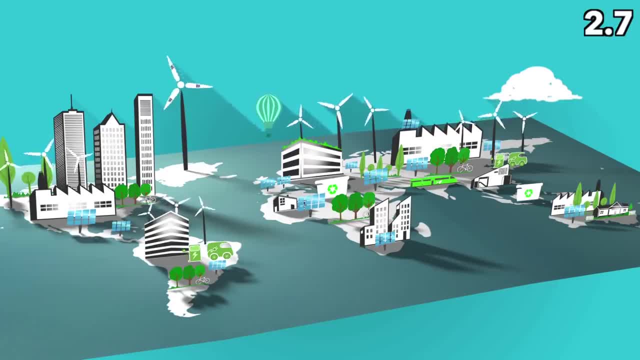 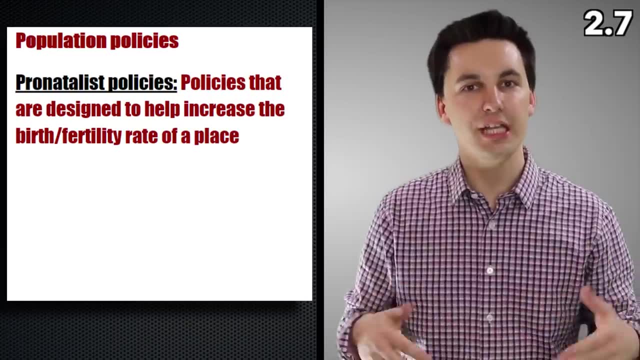 There's environmental sustainability, there's urban sustainability, and this can lead the government then to create policies that might be pro- or anti-natalist policies. Countries that are starting to see a decrease and need more people to be born often use pro-natalist policies to encourage citizens to have more children. 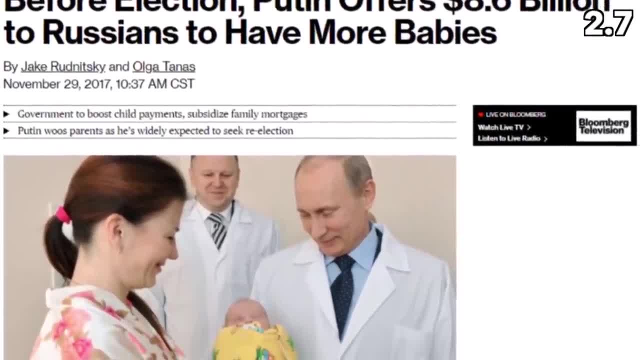 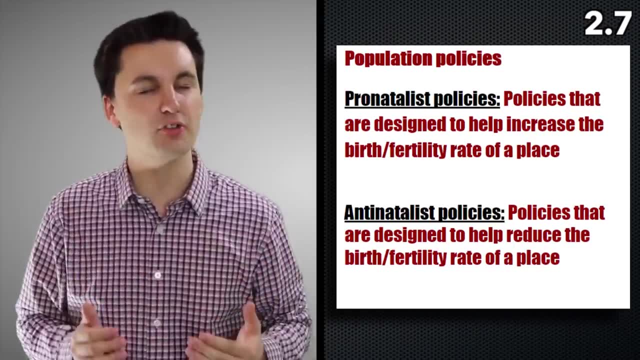 This might be in the form of exemptions. This might be in the form of exempting them from income tax or offering different benefits to larger families. Should a government actually regulate birth rates or not? Some areas around the world, it gets controversial. 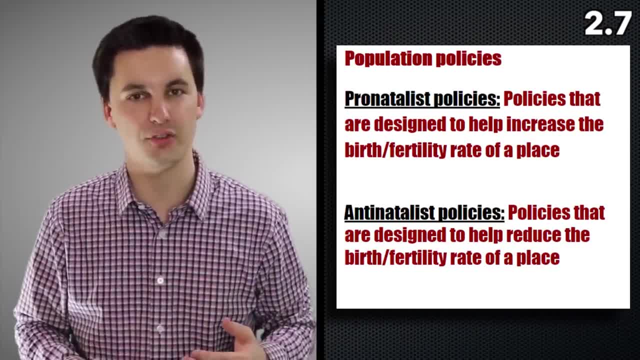 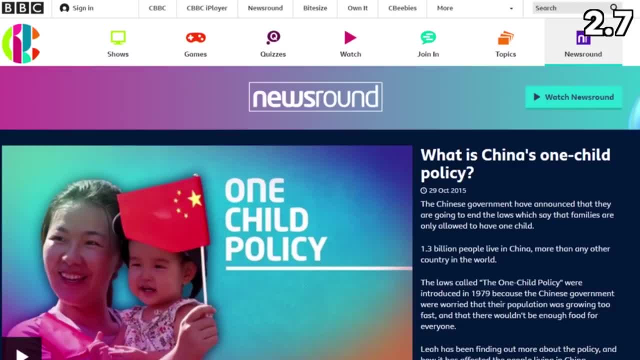 One of those areas of controversy is when we get into anti-natalist policies. Here governments are actually preventing population growth. Most famous example is probably China and their one-child policy, where they actually limited the legal amount of children a family could have. 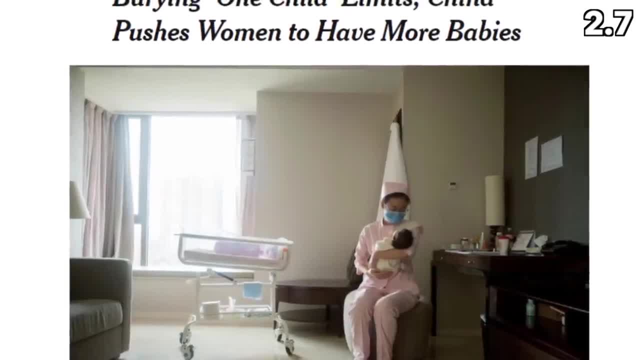 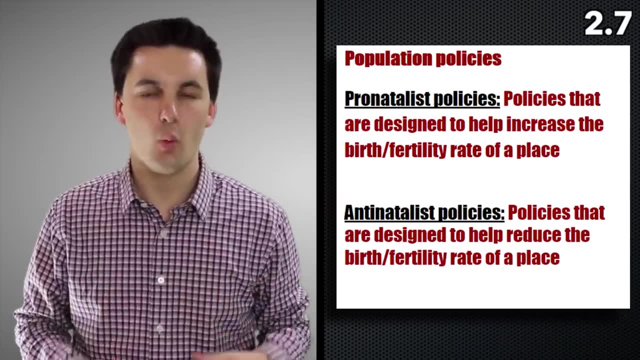 And recently it's been reversed a little bit and that's because some of the unintended consequences that have come from it. They're falling below that replacement rate. There also became a huge gender imbalance where we start to see more men being born. 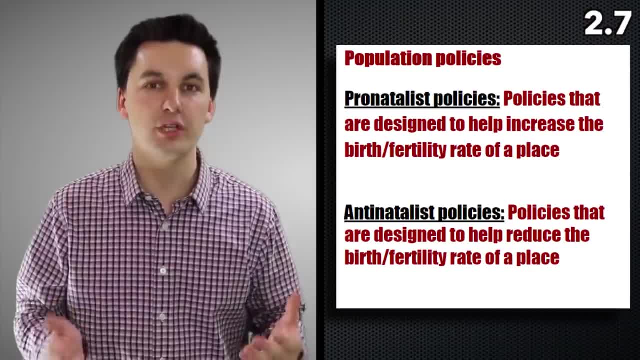 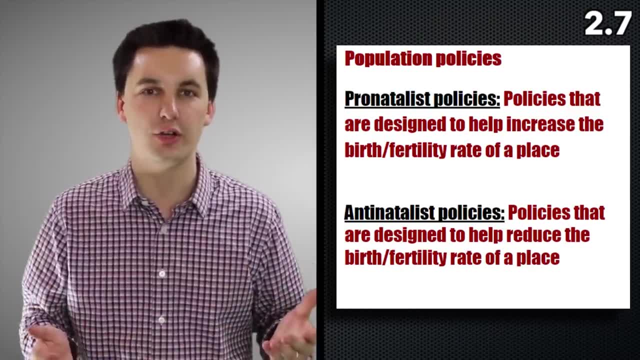 and actually gender selective abortions occurring and, unfortunately, has created a massive shortage of women. And when it comes to marriage, we're starting to see things like mail order brides and human trafficking occurring in the area. Next we have 2.8, and this is all about women and demographic changes. 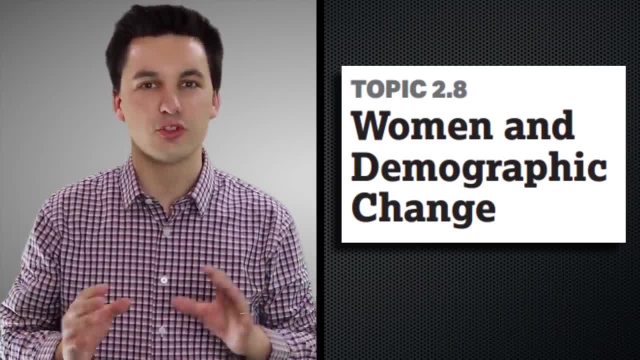 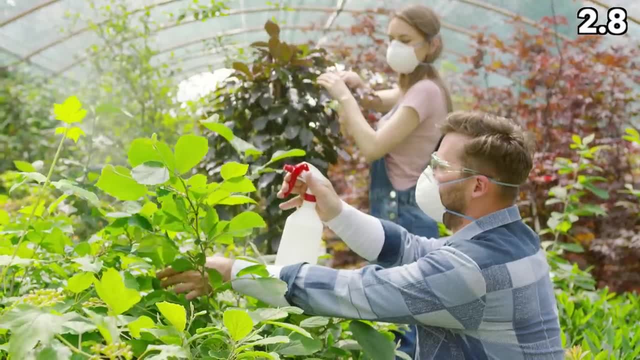 The nice thing here is this is actually a recap. 2.8 is all about themes and trends that we can see. As society continues to advance, We start to see the TFR go down. One of the things that causes this is women now have access to contraceptives. 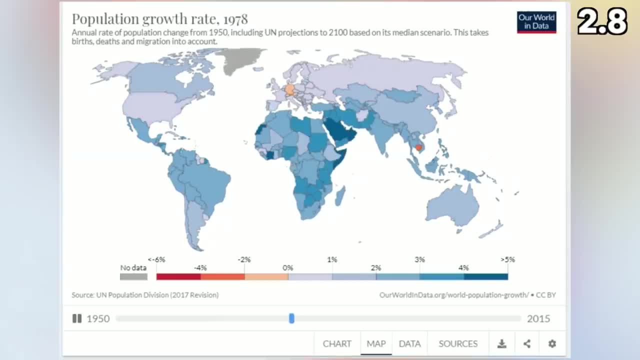 Family planning becomes actually practice. We also see women gain opportunities within society, And that allows them to have a job, a career, and pushes back the amount of time they have to have children. And these opportunities that are created for women only happen when we see cultural shifts. 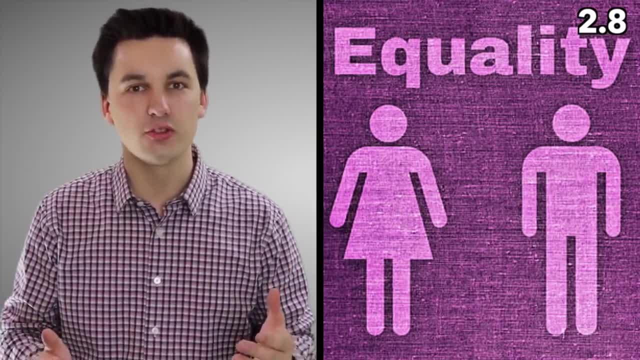 When women are no longer seen as caretakers and are seen as equals to men. 2.9 is another one. 2.9 is another one. This is a bit of a recap. We've already talked about a lot of these concepts. 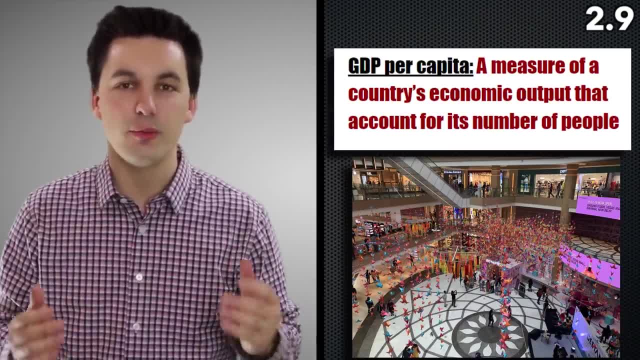 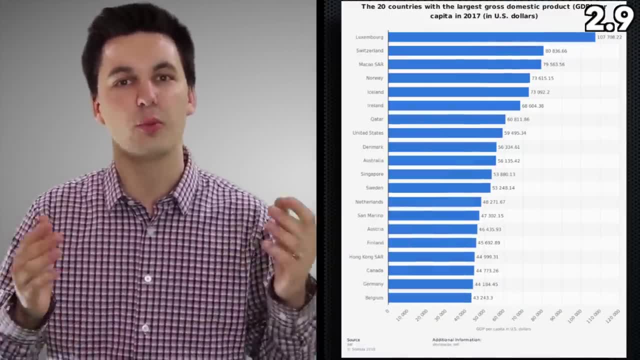 This is all about aging population. Today, the standard of living is much higher And that's because of our GDP per capita. We have more access to goods and services. We have more production, more specialization. All these things have increased our life expectancy, allowed us to travel more, allowed us to interact. 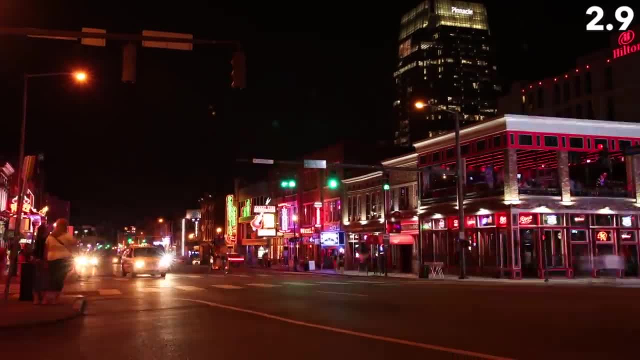 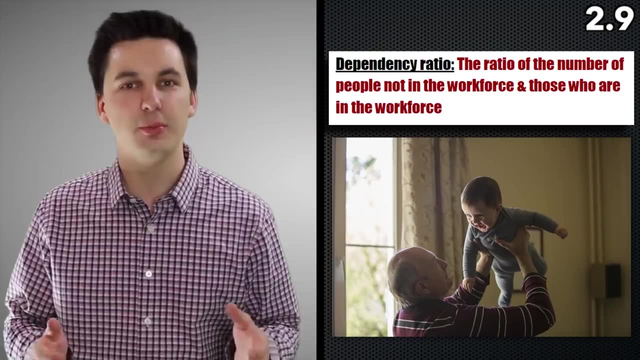 with one another in new and exciting ways. Now, one of the issues with our population aging and as we continue to live longer is our dependency ratio. The dependency ratio is the amount of people who are working that support, the amount of people who are not. Normally focusing on people who are retired or children who aren't able to work. If your dependency ratio becomes too high, we're going to run into some issues here. Not enough people will be putting money into the system to be able to support those who 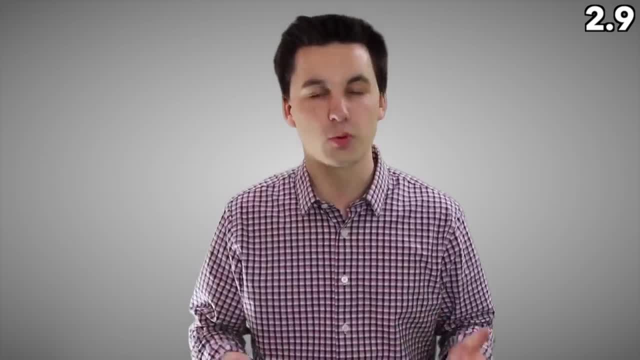 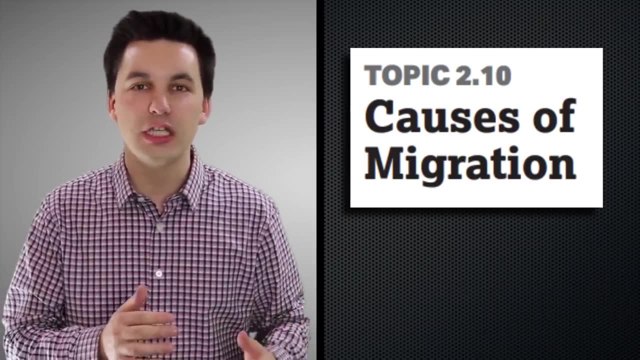 can't. Countries like Japan and Germany are having a hard time where they don't have enough workers to be able to support their population. This is the final part now of Unit 2, and we're moving away from looking at some of the demographic data and focusing more now on migration. 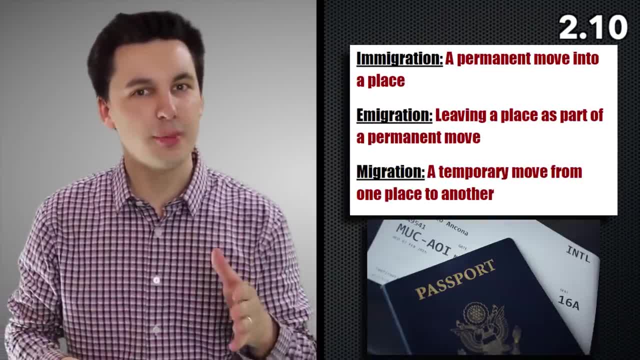 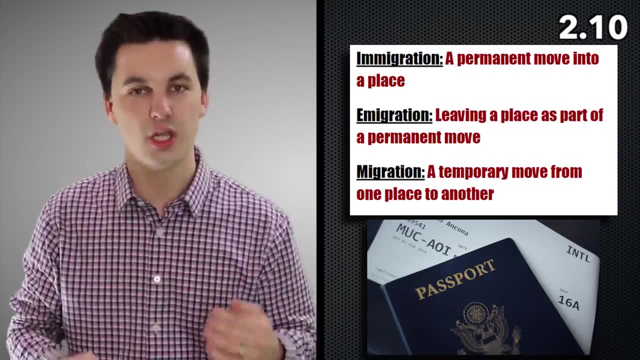 2.10 is all about the causes of migration. First thing I got to make sure that you remember is the difference between immigrate and emigrate. Immigration is when we are coming into a country You are going to live there permanently, Not temporarily. that would be more of a migrant. 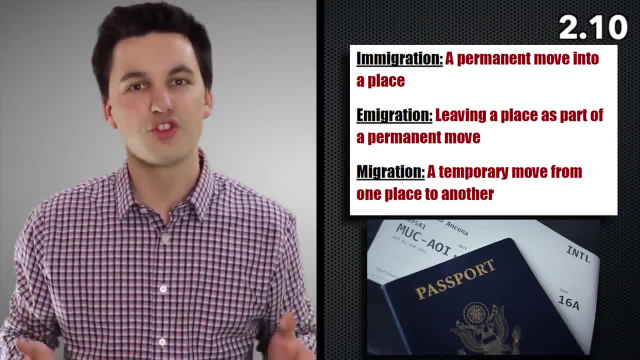 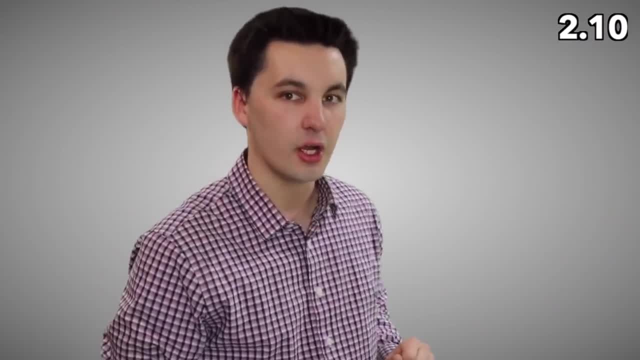 Emigrate is when we are exiting a country. A lot of times when we talk about migration, we're focusing on push and pull factors. Push factors are when you're pushing something away- It's pushing you out of an area- While pull factors are when you're moving away. 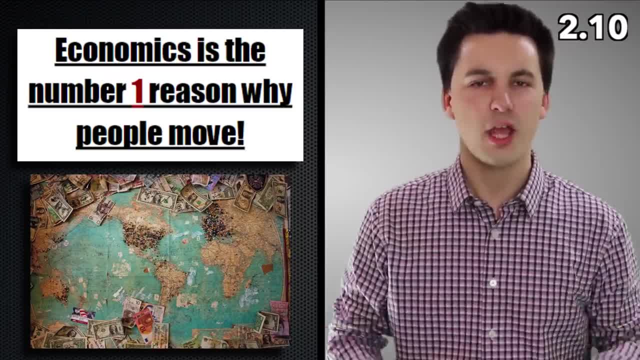 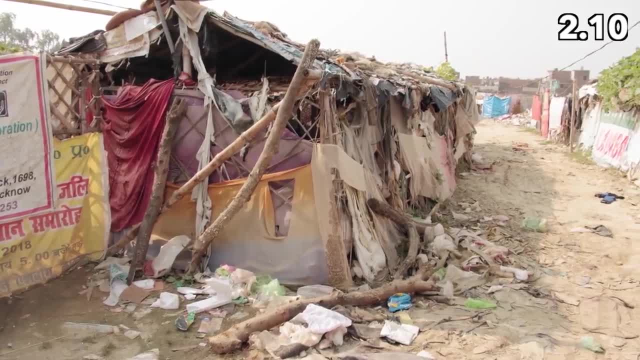 The number one reason why people migrate is economic. If I live in a city that doesn't have a lot of opportunities for me and I don't have a job and I can't find work, I'm not able to support my family or even just myself. I'm 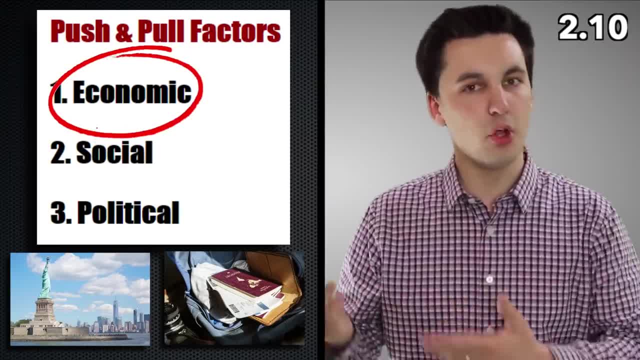 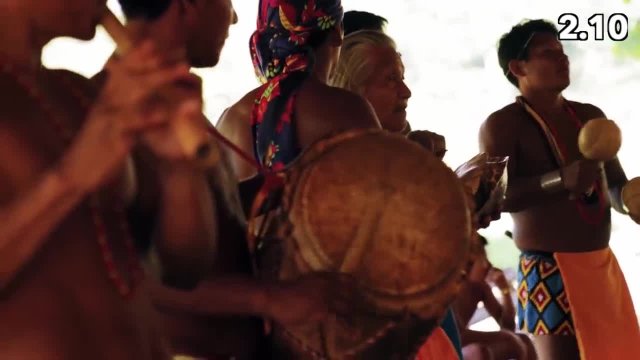 going to probably look for somewhere else to live. On the other hand, it could be a pull factor as well. I'm going to go to an area that has a lot of economic opportunity. Another push and pull factor is social factors: Going to an area where you feel like you belong. 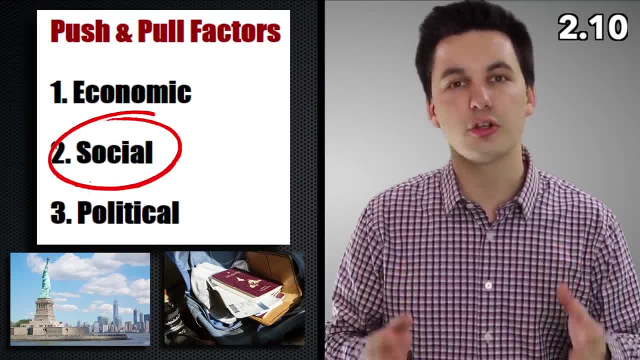 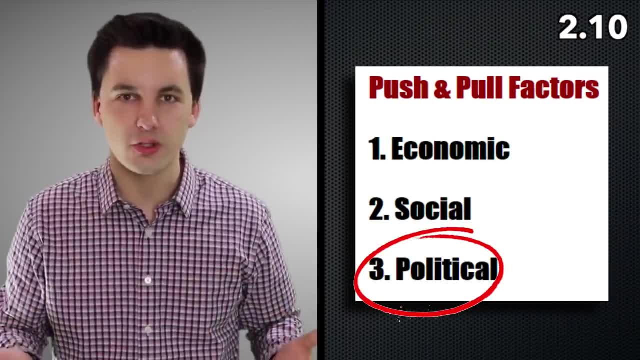 On the other hand, it could be a push factor as well If you don't feel like you're included in a community, if you feel distant or not accepted. The last main category for why people move is political reasons. If we're running into issues with crime and there's corruption, that's happening and I 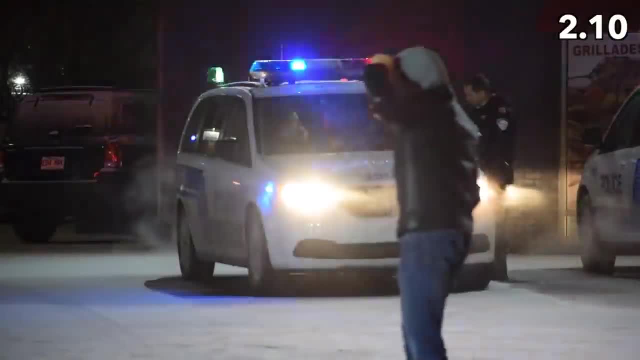 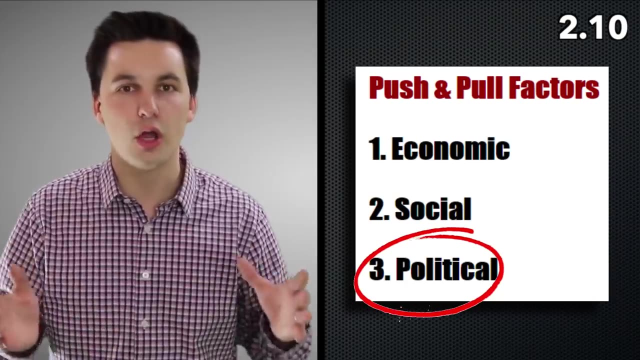 don't want to be part of this anymore and I'm looking for more stability. I'm going to move out. If I'm living in a region of the world that's struggling to have stability, or a state where the government overall is corrupt or they're abusing their power, I'm going to want to. 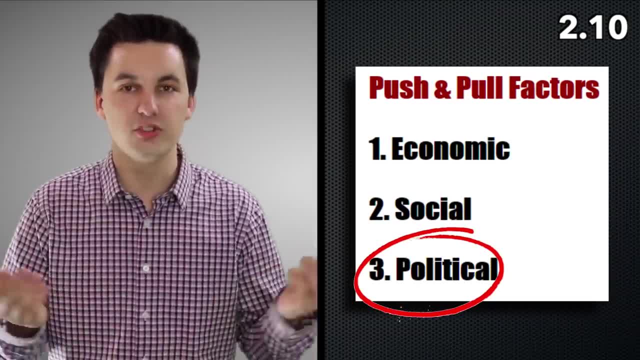 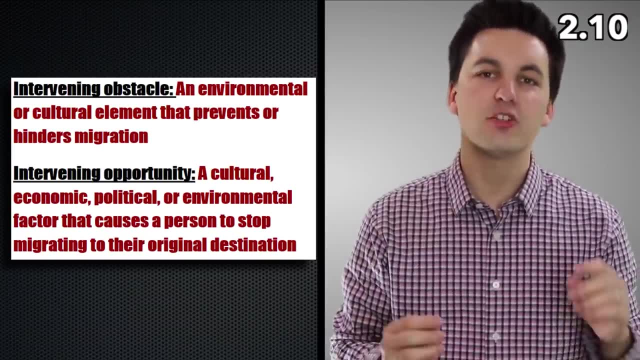 find somewhere else to live And a pull then for political reasons. So the government plays a role into migration patterns as well. One last thing: when thinking about causes of migration that I almost forgot about: make sure you know the difference between intervening obstacles and intervening opportunity. 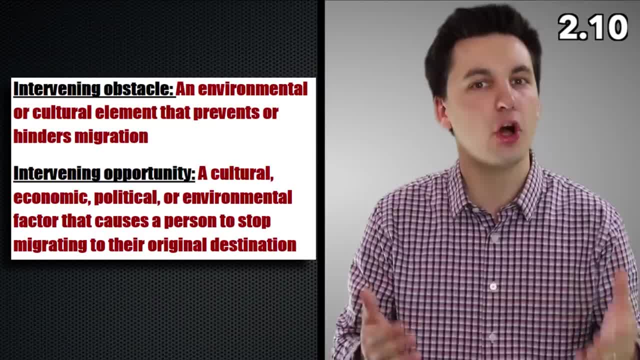 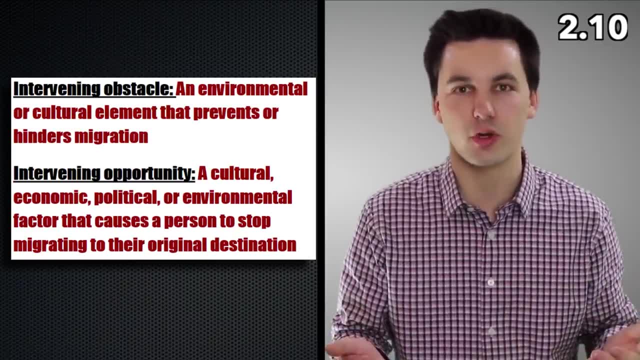 Intervening obstacles a lot of times are the rivers, the mountains, different cultural factors that would prevent someone from getting from one location to another. Sometimes, it's actually governments that are putting restrictions on immigration. Intervening opportunities, however, is something that would prevent us from getting into our. 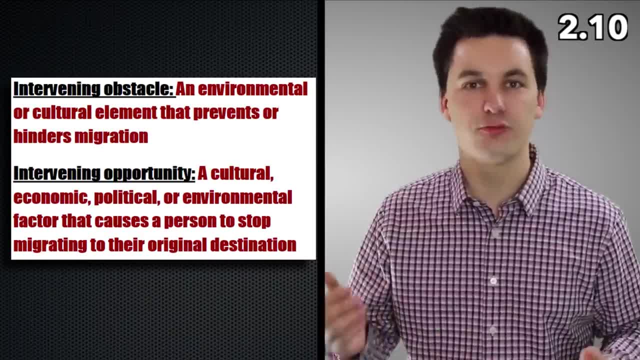 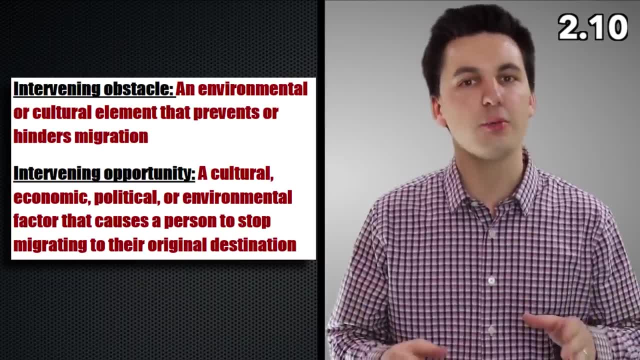 original destination. For example, If I was going to move from Minnesota to Florida and while I was going down I stopped in Chicago and was offered a job and decided to take it and stay there, that would be an intervening opportunity. Before we move on to 2.11,, I want to quick highlight Ravenstein's 11 laws. 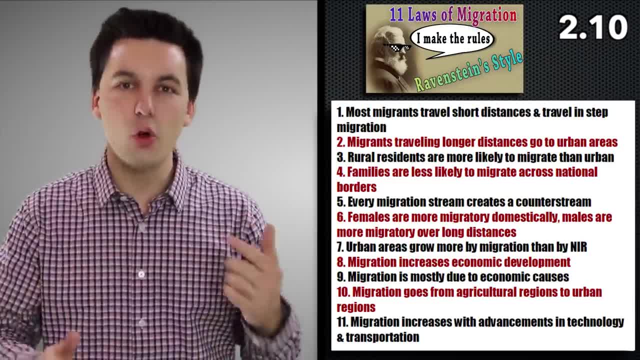 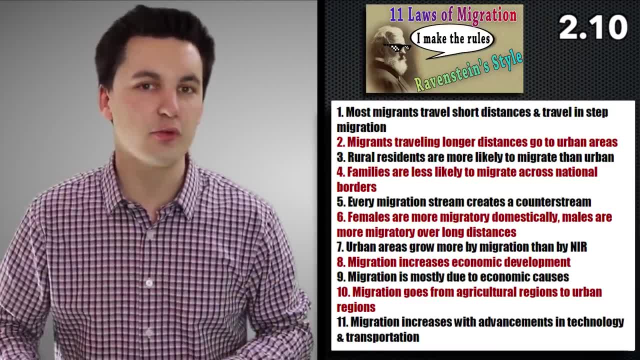 The laws are important, not necessarily just to memorize. what's more important about them is to look at the themes and trends we can see. These are the reasons why people are moving Now. they have changed. over time. We've started to see more families migrating longer distances. 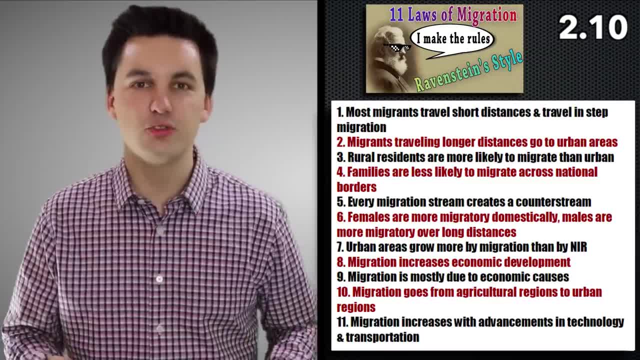 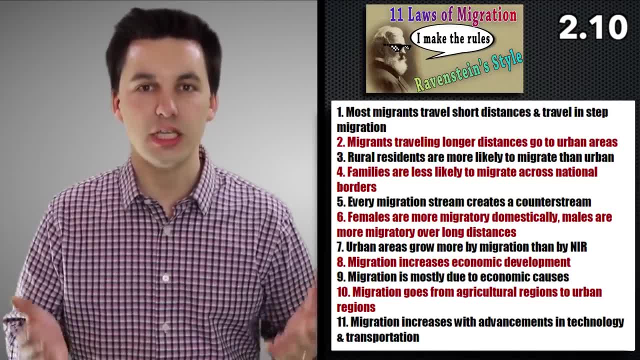 Some of these laws are actually becoming a little bit outdated As technology keeps changing, allowing people to communicate with others more, be able to access information they need and to be able just to move easier through harsh terrain. 2.11 is all about forced and voluntary migration. 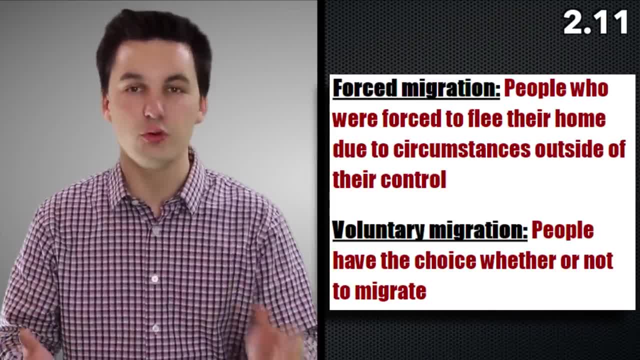 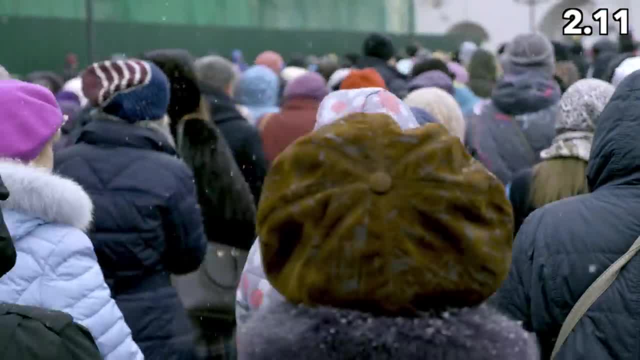 Now, forced migration is when someone is forcing you to move. You don't have an option here. Voluntary, you can probably guess it, you're the one deciding to move. Most of the time, forced migration happens because you are not in a safe environment. 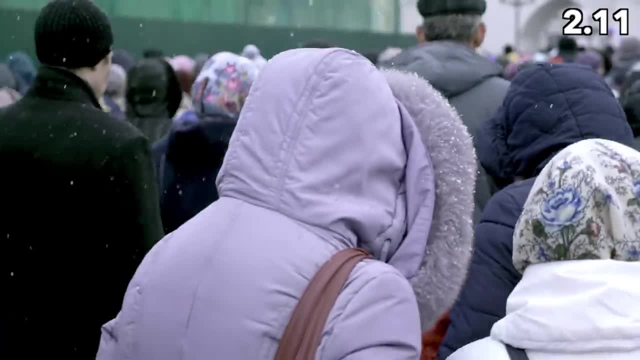 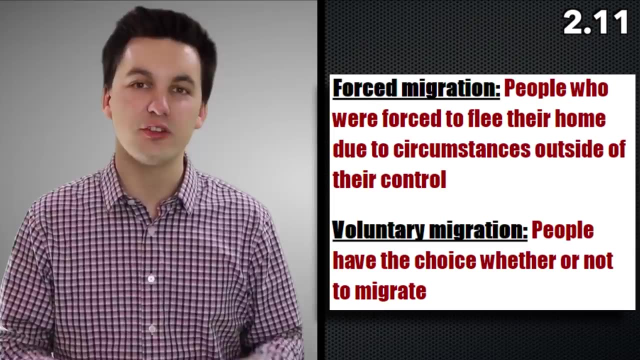 maybe it's a natural disaster: civil war, Genocide. the government is oppressing people. Voluntary. you're normally looking for other opportunities in life. however, you're the one making the choice. Your life is not in jeopardy When people migrate for things that were out of their control, and especially for things 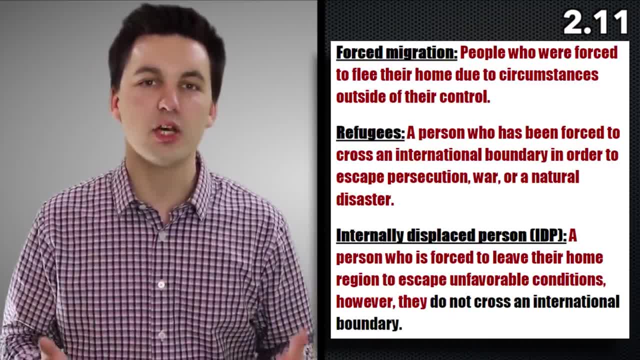 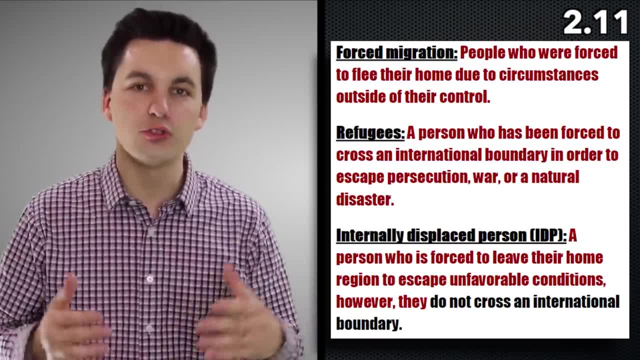 that are putting their lives in danger. they can try to become refugees. You have to cross an international border. You cannot stay in your state. If you stay within your own state's boundaries, then you are an IDP, an internally displaced person. 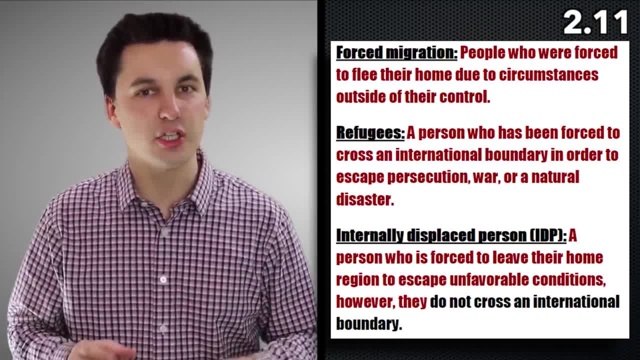 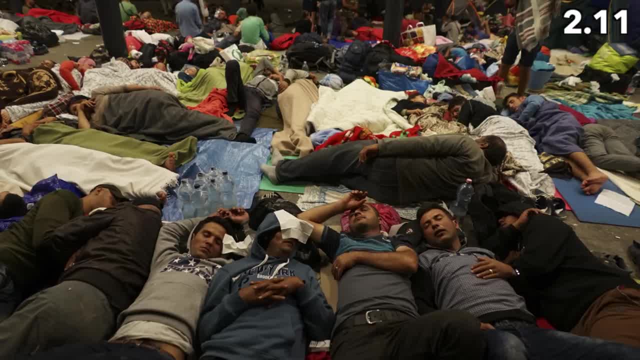 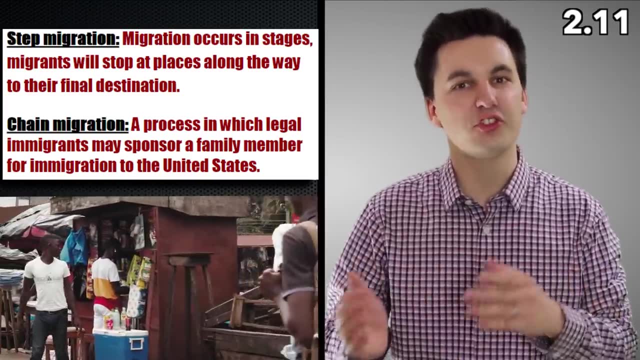 These are seen as domestic issues and most of the time, the UN isn't going to get involved, And we can look at Syria as a great example of the most recent refugee crisis, as people have fled Syria due to the Syrian civil war. Another important distinction to make in 2.11 is the difference between step and chain migration. 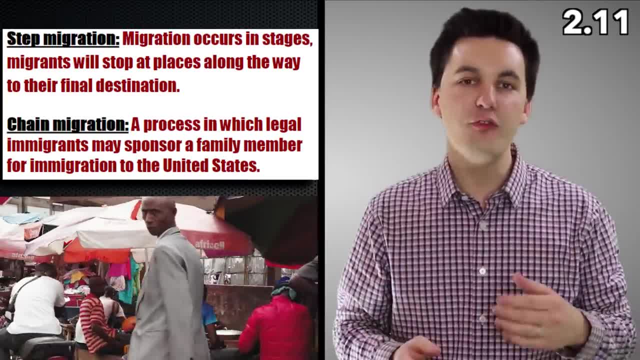 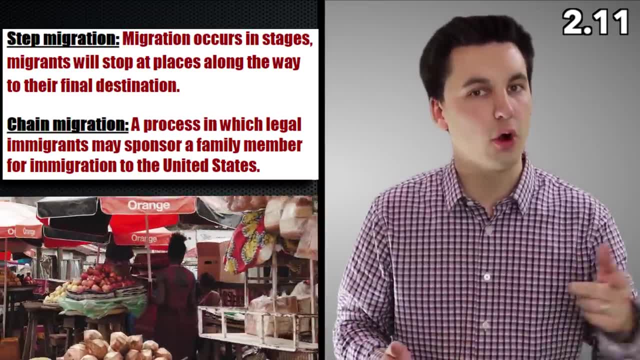 Step migration is when we're traveling long distances. Often, migrants will stop at certain locations for a period of time. Sometimes they'll end up actually staying there due to intervening obstacles or other obstacles. Chain migration, on the other hand, is a family-based policy for migrants. 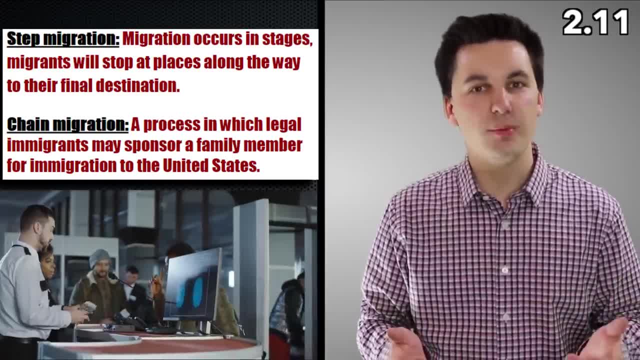 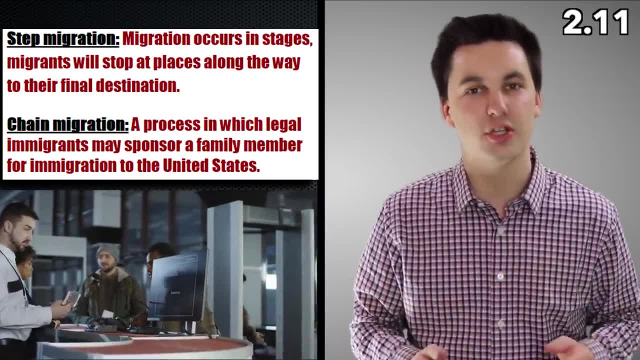 If someone immigrates into the United States illegally, they could use chain migration to get one of their immediate family members to come over with them. It requires someone to have legally immigrated into the country, and then they would apply through the government to get their immediate family members to come over with them. 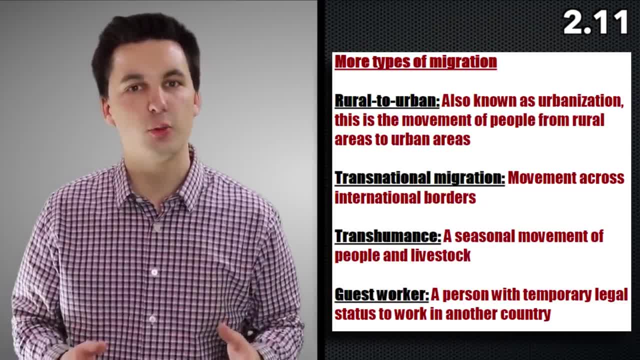 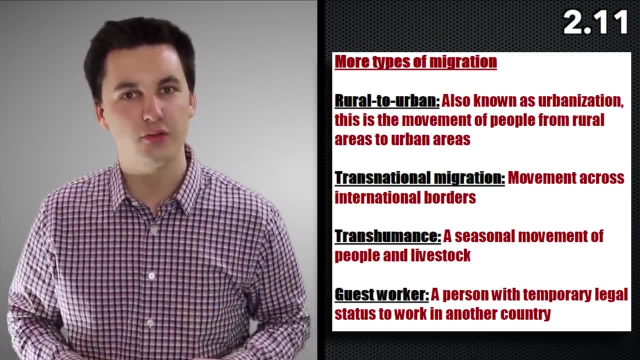 One last thing that we should really talk about is we're seeing a lot of migrants moving from rural communities into urban areas. This is known as urbanization, And again, economics is the driving force here. Cities and urban areas offer a lot of opportunities for people to work. 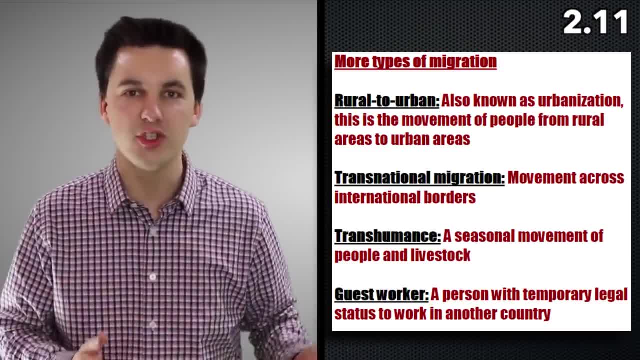 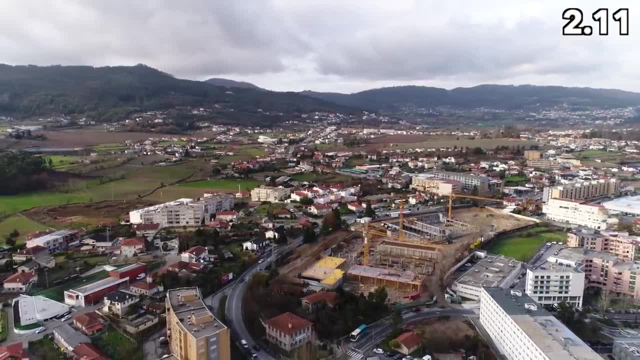 They offer a lot more money, more access to goods and services, even such things as healthcare. Now, in some areas, though, we're also starting to see some counter-urbanization occur, where we're starting to see people leave the city and move back into the suburbs or into rural. 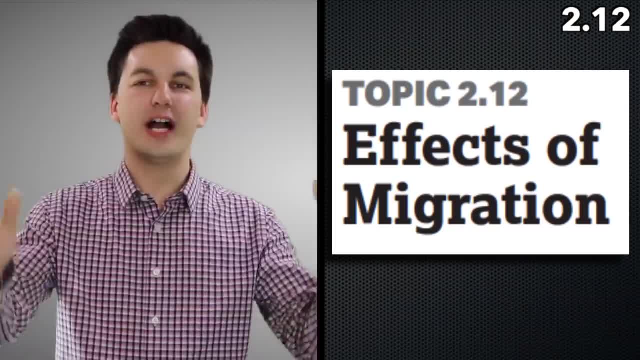 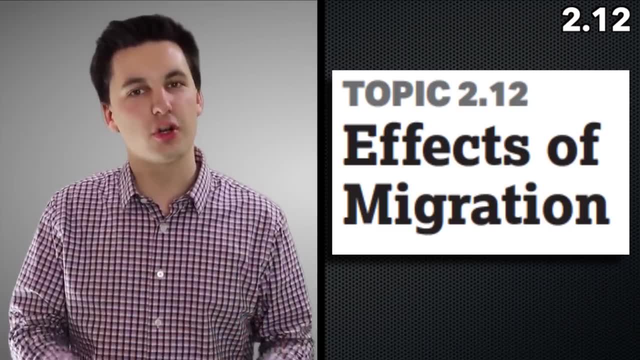 communities that still are relatively close to the city. All right, We are on the last one, 2.12.1.. Which is the effects of migration. The nice thing here is this one's a little bit shorter because it's going to come up. 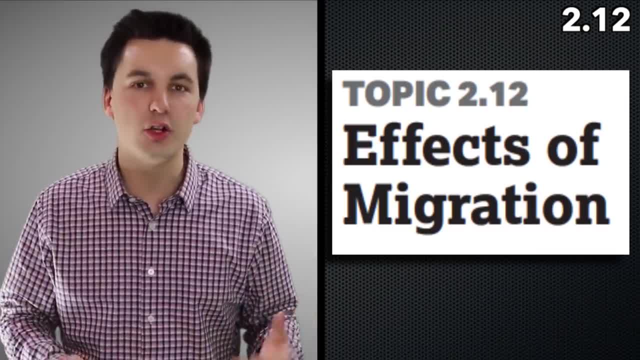 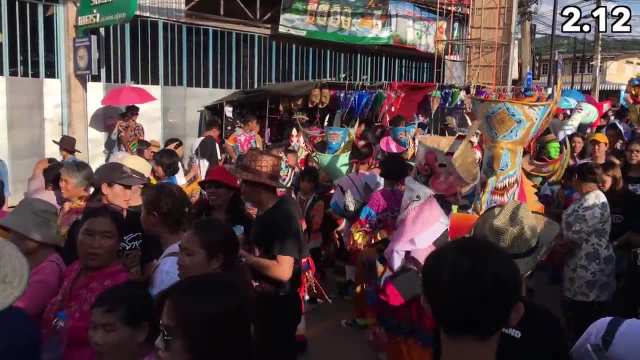 a lot in our culture unit in unit three. But really when we're talking about here, we're looking at what happens to people when they migrate to a new area. What are some of the impacts? How does the host culture change? How does the new culture coming in change? 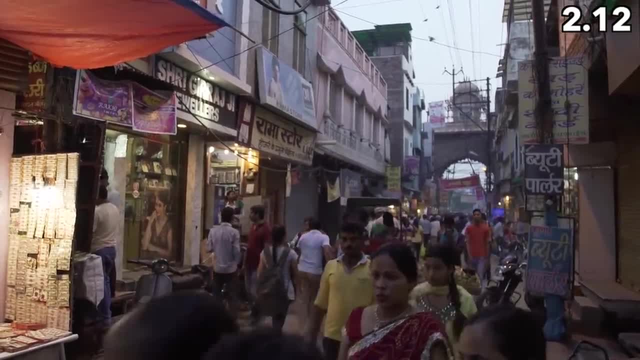 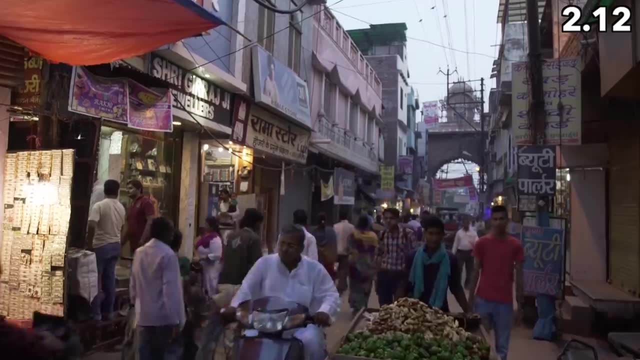 What's going on? One of the things we can see is assimilation might happen where whoever moved into the new society will leave behind all their old cultural traits. They'll just adopt what society they moved into. They'll take on the new culture, wanting to fit in. 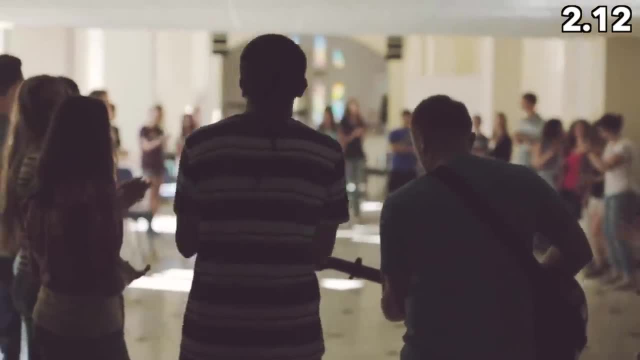 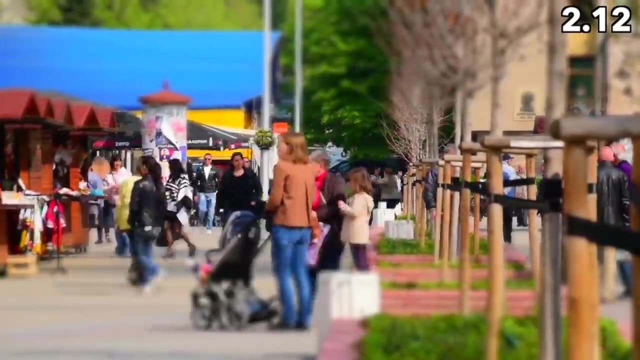 Or we can maybe see acculturation, where it's a hybrid, it is back and forth. I will retain some of my cultural aspects, but I'll also take on aspects of the new culture that I just got into, And we might see things where we have alienation occurring as well, where the society actually 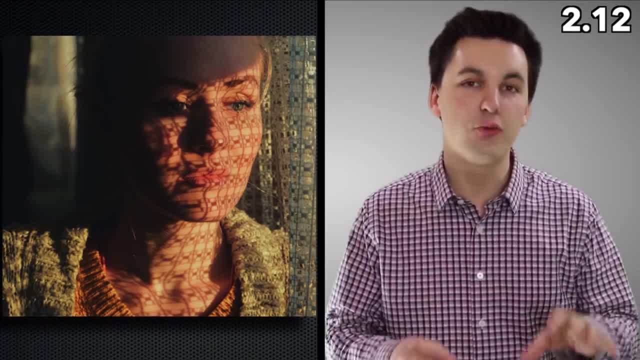 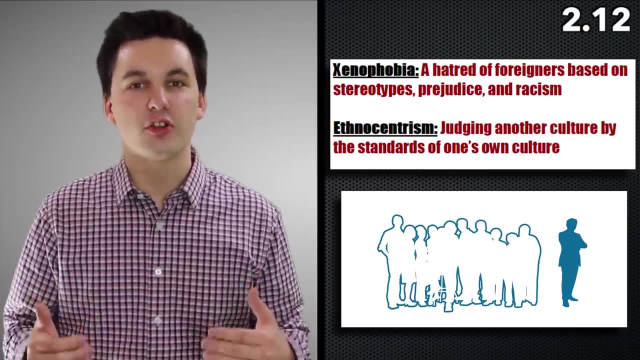 rejects the migrant or the culture that is coming in and forces them into isolation, And that can be dangerous. One of the issues that could occur is xenophobia. This is when we start to see stereotypes, Prejudice and racism be applied to certain cultural groups, sometimes even resulting 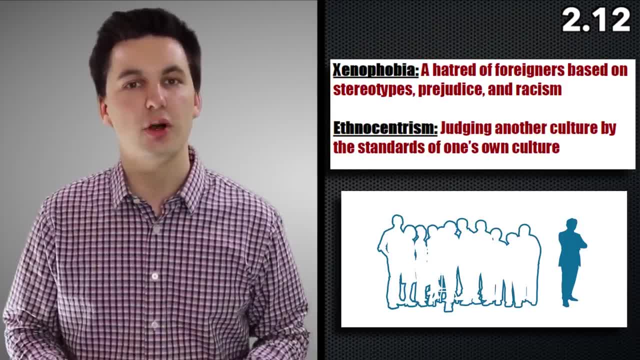 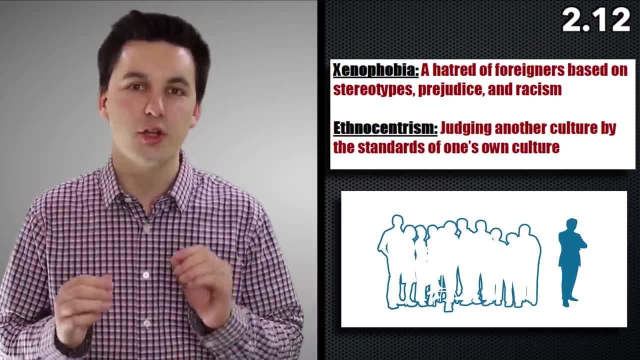 in violence that could occur. We also could run into the issue of ethnocentrism, where people don't even bother to understand the other side. They just focus on their cultural perspective, applying their own standards onto the people that they're judging. 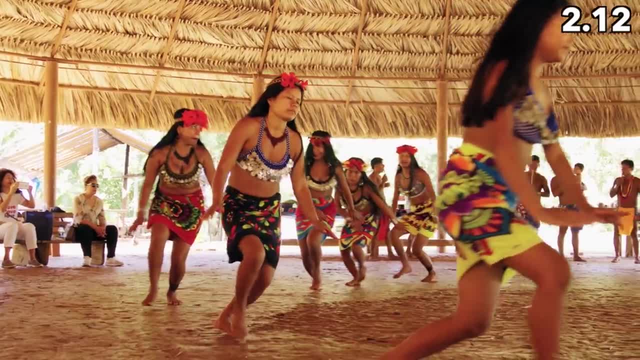 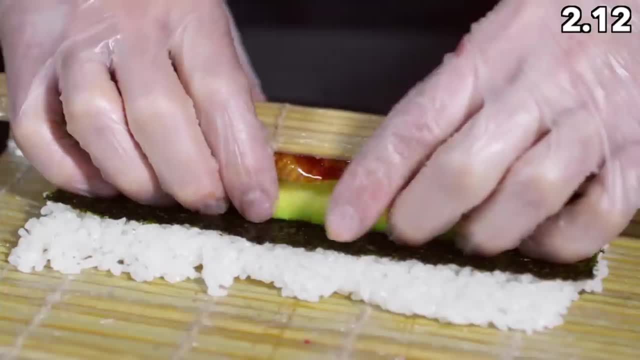 Now I don't want it to sound like migration has all these negative connotations. There's a ton of positive ones as well. We see economic growth as more immigrants come in. They bring ideas, jobs, They are entrepreneurs, They bring new cultural things we've never experienced before. 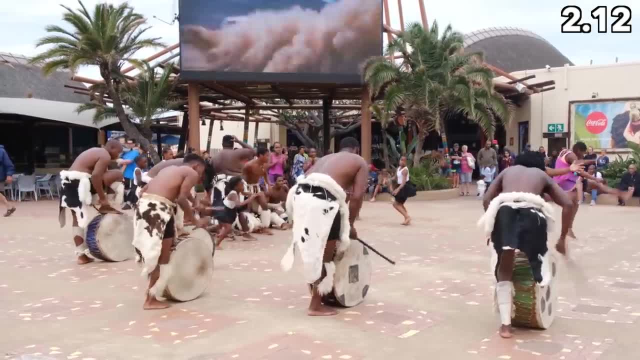 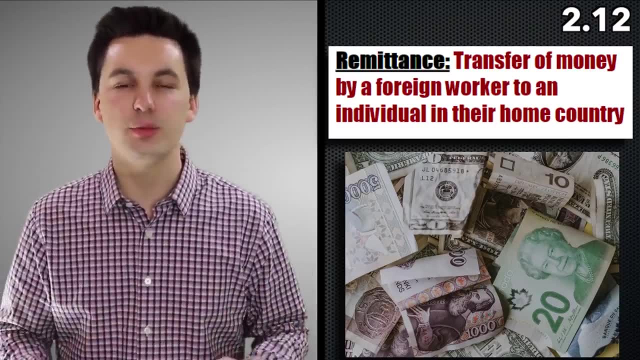 And this allows us to have new experiences in life. Other things have also occurred: re-admittance, for example. Some migrants will actually send money home to families. It allows them to be able to support families from afar and can actually help some of the 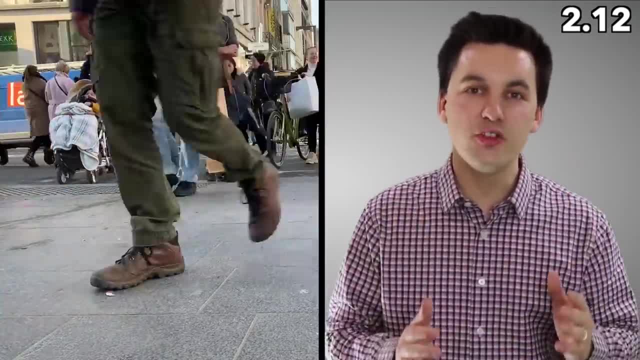 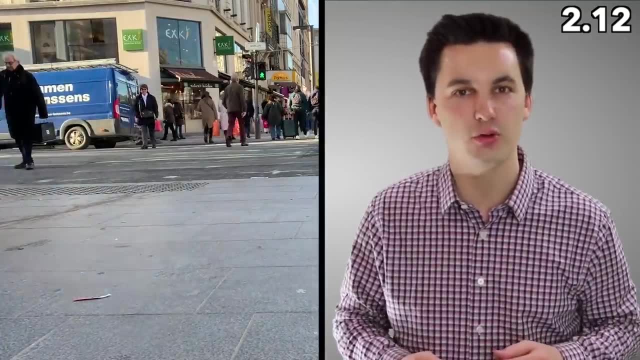 developing countries. One last thing, too, before I forget: Countries that are more developed in the demographic transition model actually need immigrants to be able to support them. They need to be able to continue their population growth As they become more developed. that natural birth rate, remember, decreases. 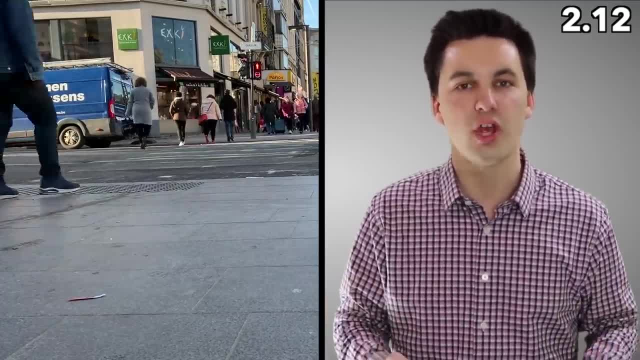 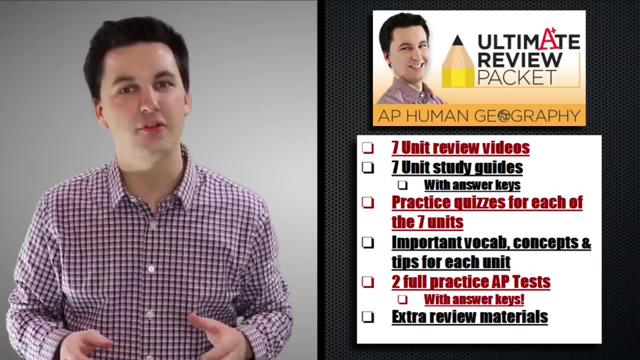 And so without immigrants, we actually wouldn't be able to have enough workforce to be able to support our population. Boom, Geographers, you did it. We are done with Unit 2.. These are all the main points you need to have a good understanding of. 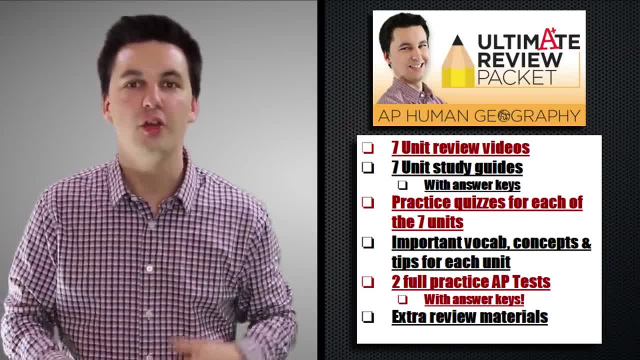 If you're still struggling on any of them, check out some of the videos on my YouTube channel. They'll go more in depth in all these different topics. Also, make sure you go back to that ultimate review packet. There is vocab there that you need to review.